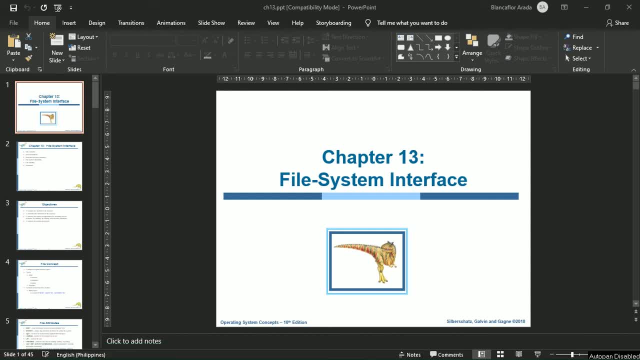 Good day to all of you. So we're already in chapter 13,. all about file system interface. So file system interface- this is another feature that makes the different OSS different with each other, So to know more about file system interface. so let's start this lesson. 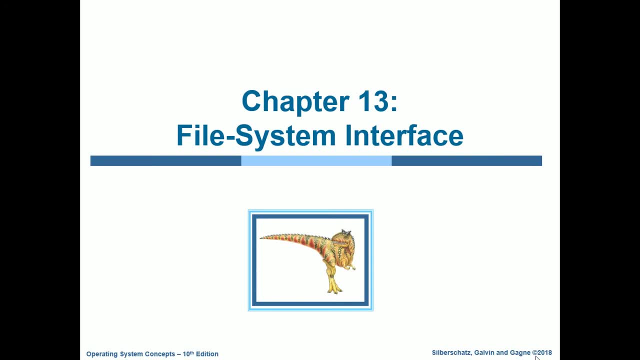 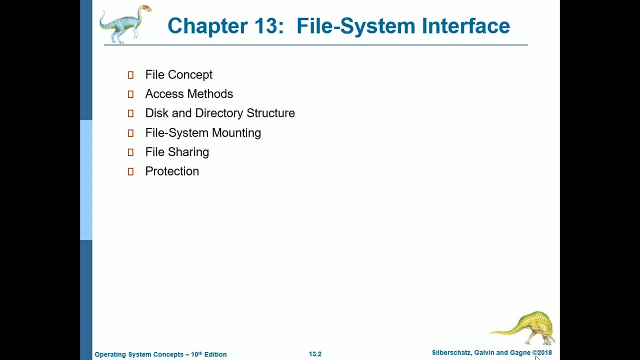 So again, chapter 13 is all about file system interface. So the contents of this chapter is all about file concept, access methods, disk and directory structure, file system mounting, file sharing and protection. So the objectives of this chapter are to explain the function of file systems, to describe the interfaces to file systems. 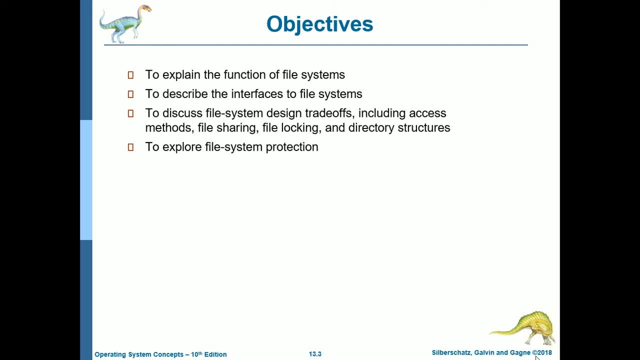 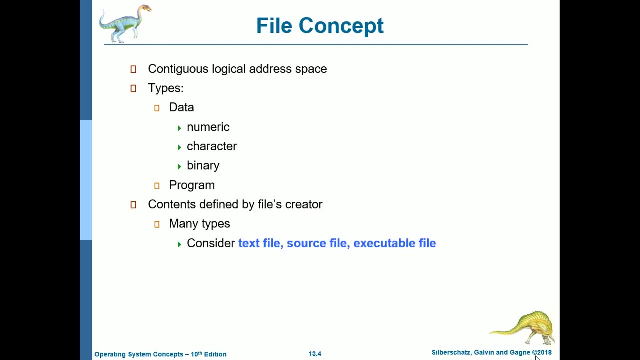 to discuss file system design trade-offs, including access methods, file sharing, file locking and directory structure, and then to explore file system protection. So let's go around with file concept. So a file is a contiguous logical address space, As I've already discussed. for example, if you have a video file that is stored in your disk, 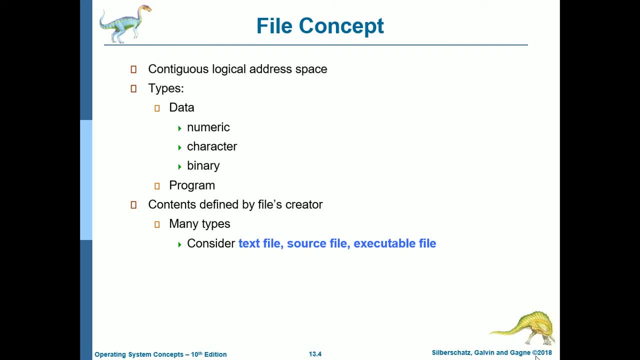 for us users we see that as a one. for example, your movie is one gig. You see that file as one chunk of one gig file of a movie file, But inside the storage or in our disk, in our hard drives, actually, if this video file is already, for example, stored in your hard drive for a year ago. 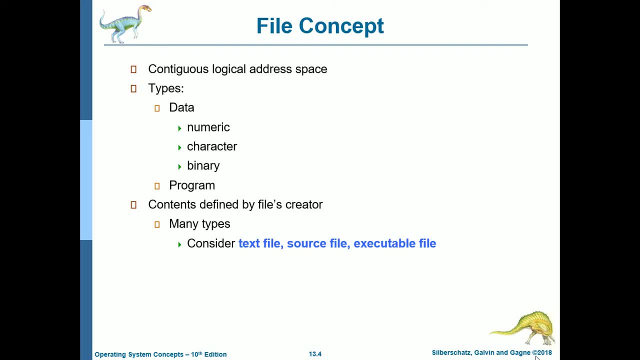 it is possible that this one gig file, its parts, are scattered around, scattered, it's not in one place in a hard drive, Okay. If, example, you're not, You're not performing defragmentation process, okay. So that is the idea here, that the file for us, we see it as one file. but if it's a large file, 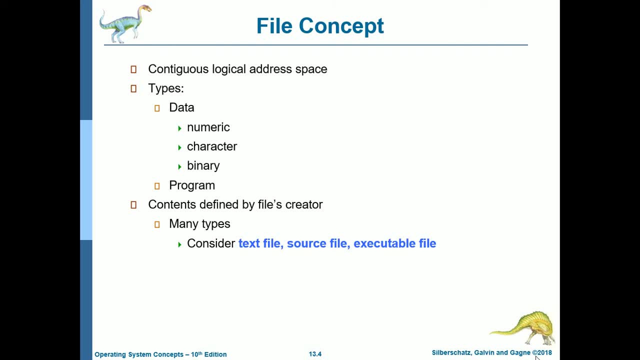 there is a possibility that its parts are scattered in all the spaces in the hard drive. It is up to the operating system that if you're going to, for example, open that file, the operating system knows where are these parts of the file. 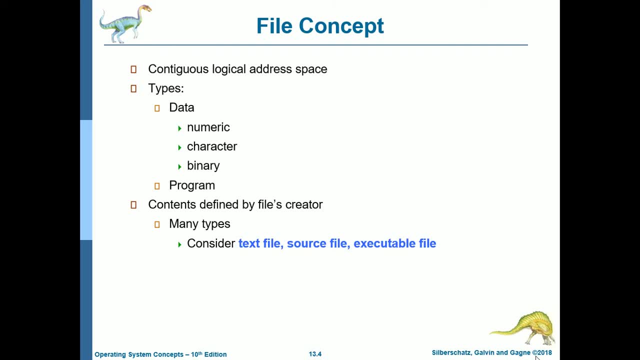 So that's why, as I told you in the previous lessons, in our previous chapters, that it's very important to do defragmentation process, because it makes the loading of the file easier, Because if your file is, if your hard drive is not going, that defragmentation process, 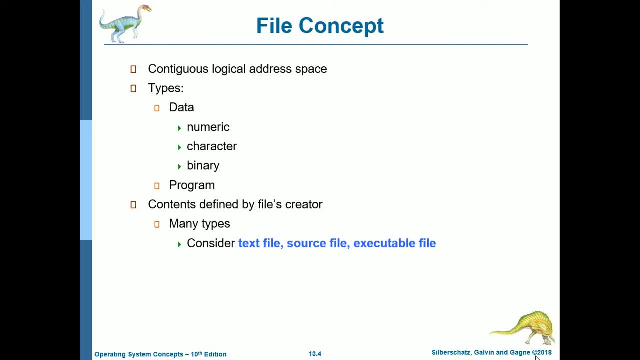 for example, for that video file, the operating system is very doing itself rigorously to locate it, all the parts of the file. So again, so for easier loading of your files, specifically large files, you must do the defragmentation of disks. 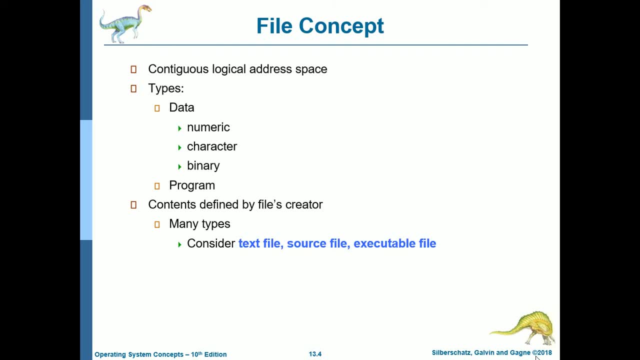 Okay, So next is we have types, So files actually has many types. It can be data, So data can be numeric, character or binary, or it can also be a program. And then the contents defined by the file. Specifically, if you are using Office Productivity Suite, so you're the ones who control what will be the contents of your document. 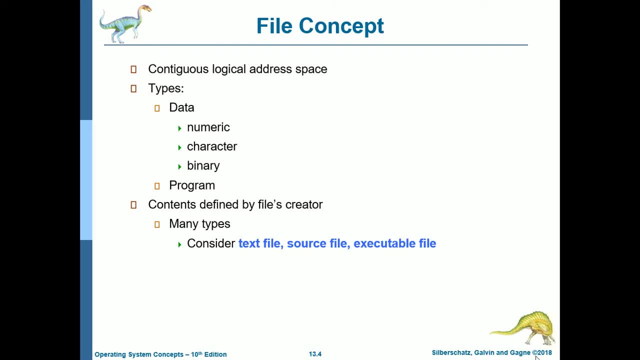 of your Excel file or of your slide presentation file, And file, of course, has many types. So this is an example. So consider a text file a source file, an executable file. So later on this slide presentation, there is a table. 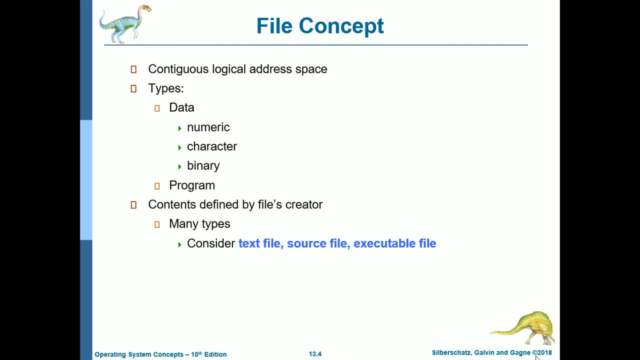 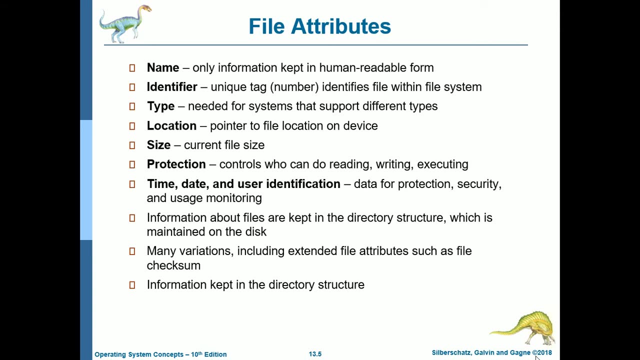 Of the general classifications of file types. Okay, Next is we have file attributes. So the common file attributes are: we have the name only information kept in human readable form. Of course, this name is also called the file name And for files that the user is creating, 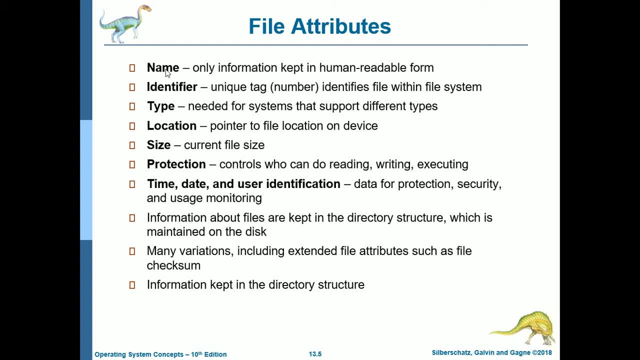 So it's also the user's description, Okay, Of what will be the name of the file, but of course for system files, for operating system files, So of course it is done by the system, but for files that is solely created by the user. 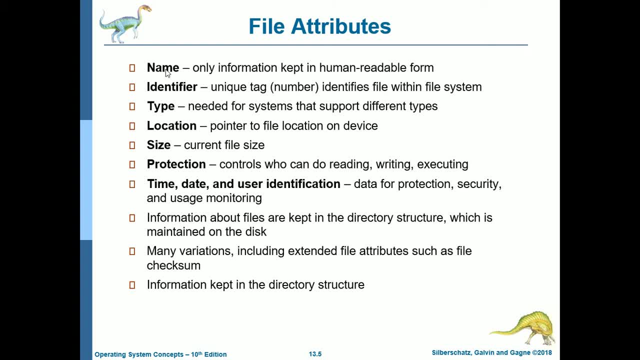 it is the user's discretion of what he or she will be the name of the file. Next is we have the identifier. It is a unique tag or a number that identifies file within the file System. And then next is we have the type needed for systems that support different types. 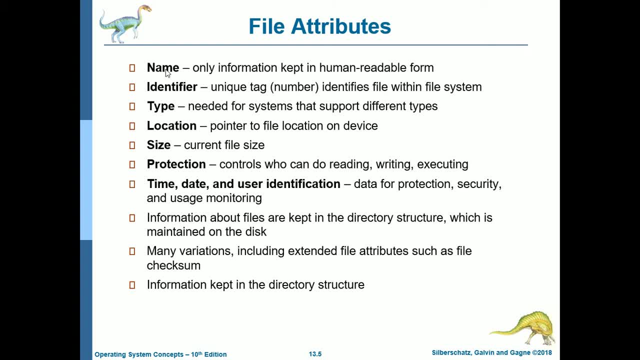 So, for type it is, it can be identified, of course, by using the file name extension. So if it is a doc X, it's a word word processor file, And then if it is, for example, a PPTX, so it is specifically a Microsoft PowerPoint. 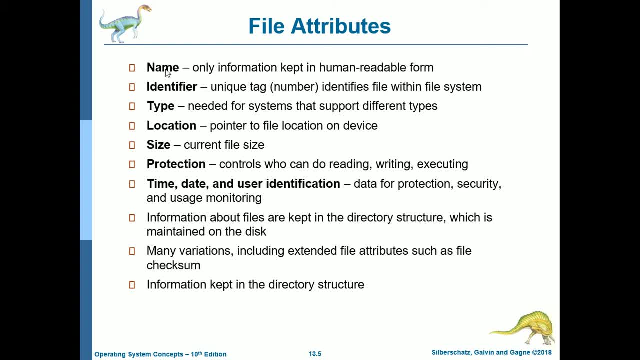 slide presentation file. Okay, Next is we have the location, So pointer to location of the file, location on device, And then, of course, the size is the current file size. And then next is we have the protection controls: who can do reading, writing and executing? 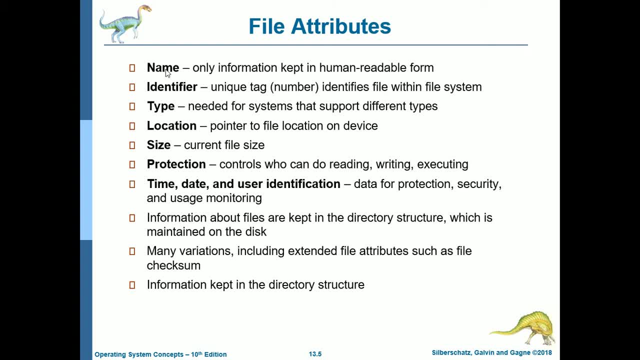 and then time, date and user identification. So data for protection, security and usage monitoring. So information about files are kept in the directory structure which is maintained on the disk. It has a separate space for the directory structure, has a separate space in the disk. 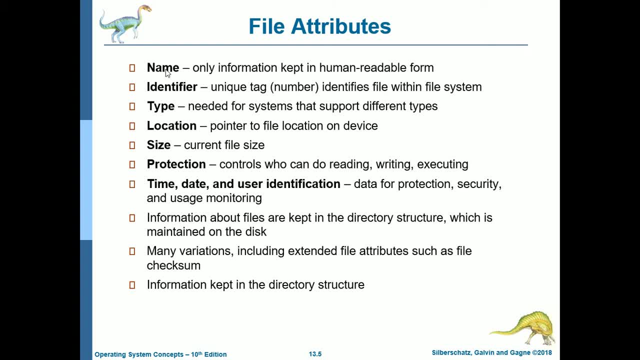 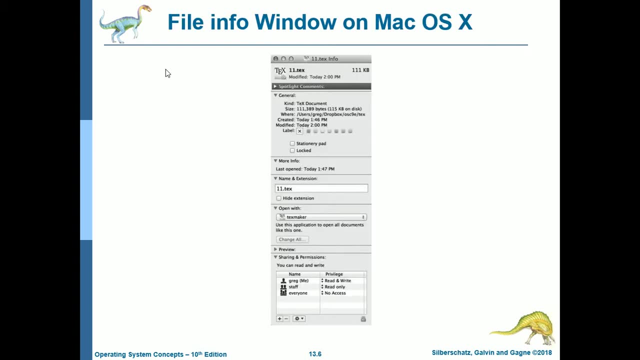 And then it has many variations, including extended file attributes such as file checksum, So that if there is a error in the file and then information kept in the directory structure. So this is an example of a file information window on Mac OS 10.. 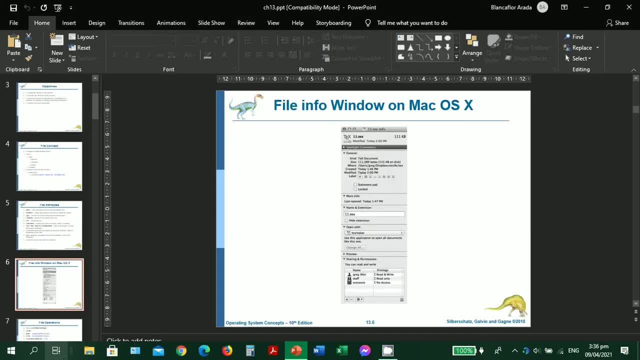 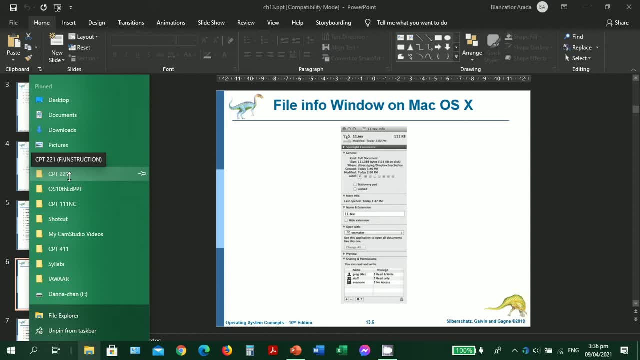 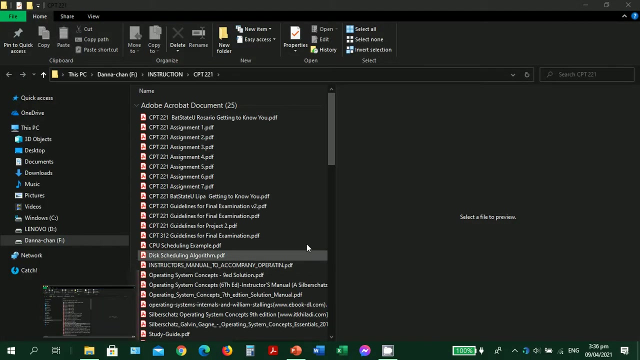 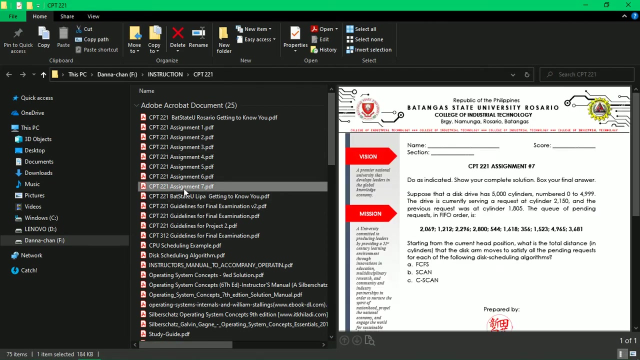 Of course Windows has its own. So Let's have an example here. So let's open our subjects folder, for an example. Okay, Just please wait for my very fast computer to load the folder. Okay, So, for example, let's open the: how are we going to know the file attributes? 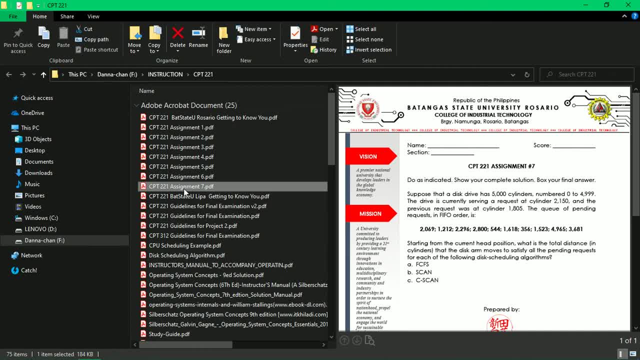 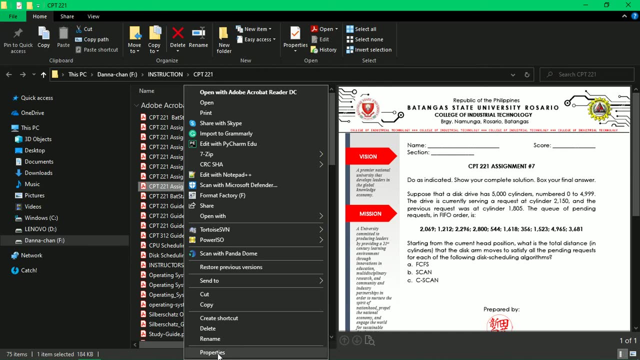 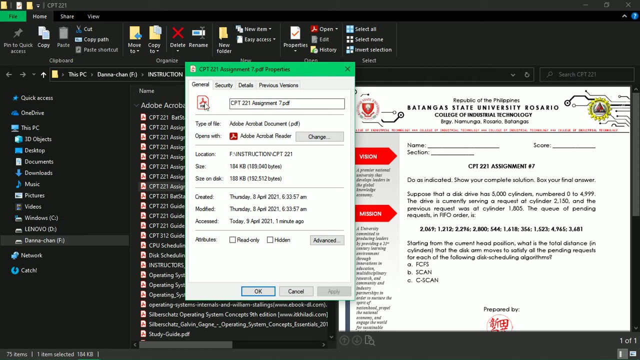 Actually it is in. uh, we're going to right click. Okay, Let's wait again to load even the, the the context menu. Okay, So we have here the properties, So this one, so with the properties. so in general, of course, this is the file name. 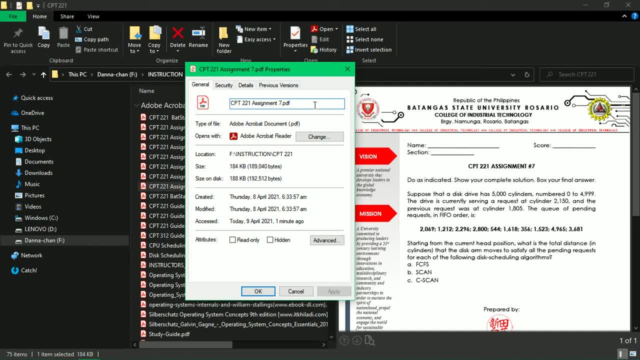 actually because it's a text box. You can edit here The name of your file And then of course it is also included here the type of file. So it's an Adobe, Adobe Acrobat document or PDF portable document file and opens with. 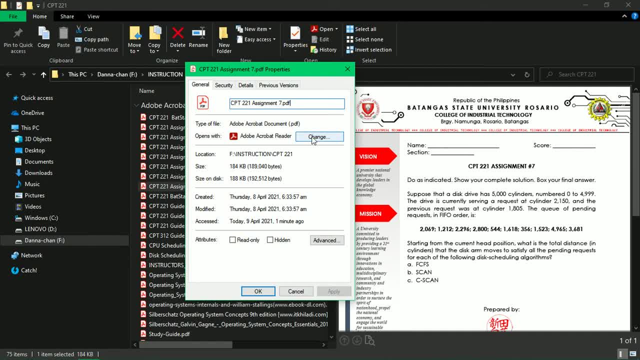 with, of course, Adobe Acrobat reader, but actually you can change if it, if you want to, and then the location in the folder, and then the size, and then the size on disk. So there is difference with the size, Okay, And then the size on the desk. 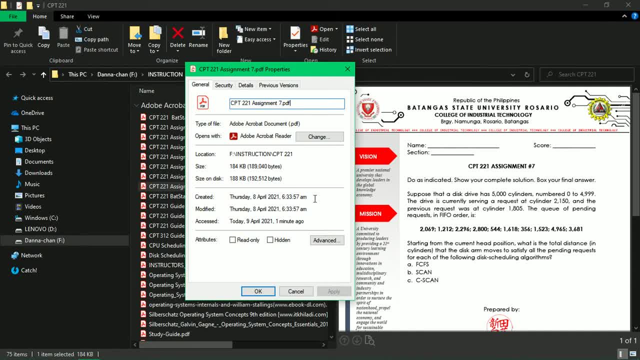 And then also here we have the uh created when it was created, when it was modified And, of course, since um we accessed it today, even the property So uh, for security purposes. So it has a log that um the latest that it was accessed, one minute ago. 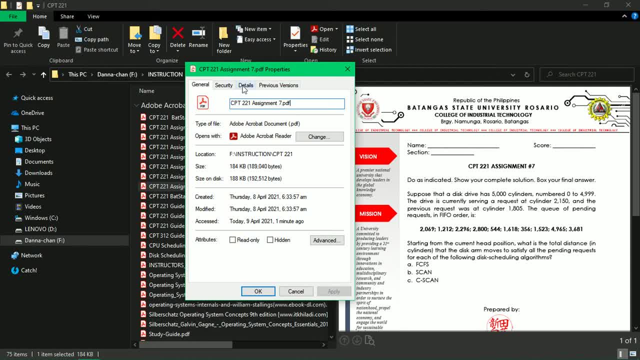 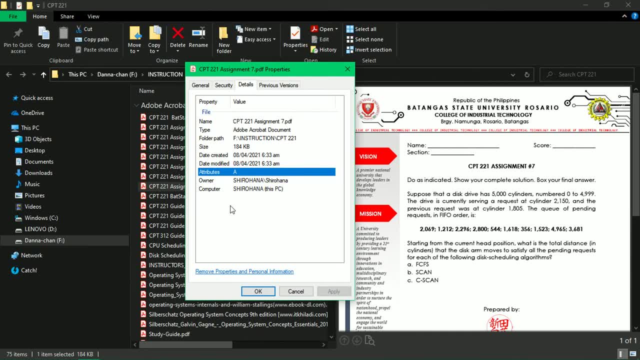 So if you want to know more the details of the file attributes, Okay, We have here, so it's almost here. but there are also different um files that has longer details. So for PDF it's also just the same as with general. 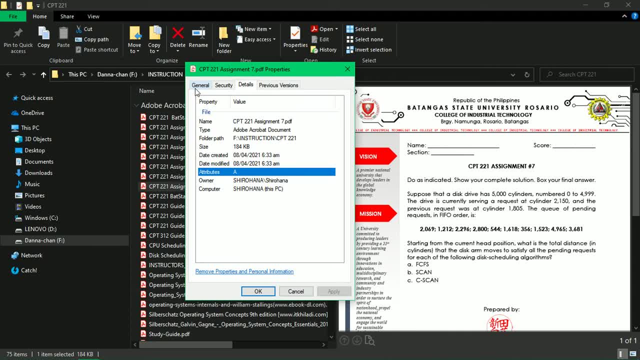 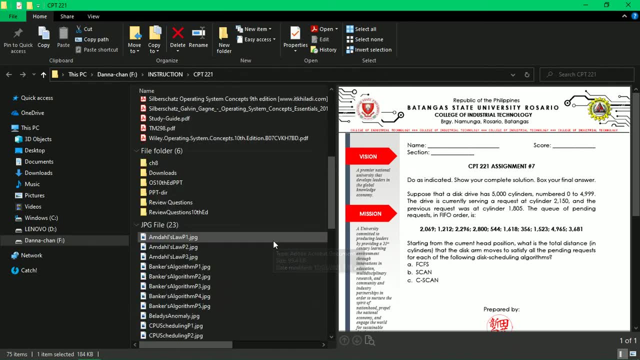 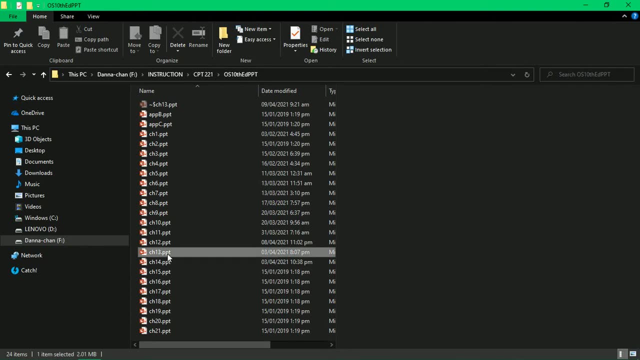 So actually, it depends upon the, the, the file that you're going to look for, the properties, because there are, for example, uh, let's look with other properties, Okay, So This is a slide show presentation, So let's see. 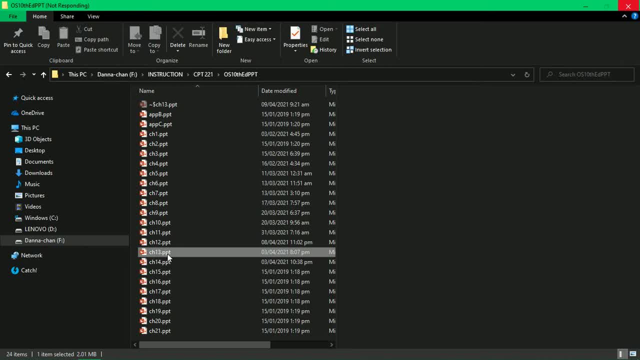 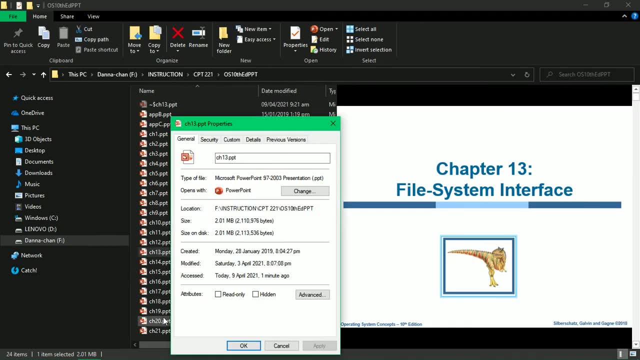 Okay, Let's wait for it to load again. Okay, So this is the general, just as the same, since it's like. this general is the summary And then these are the details. So, as you can see, for slideshow presentation there are authors and then who last saved. 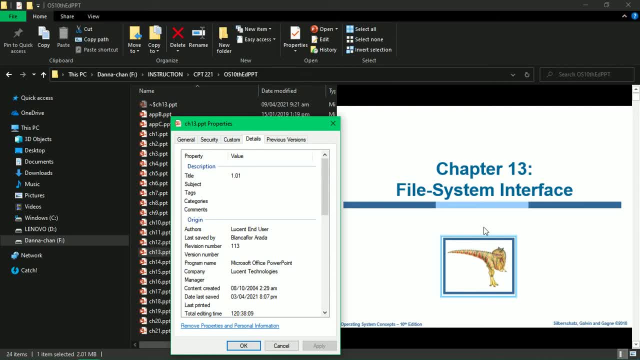 by how many revisions does this slideshow presentation has undergone? and then, of course, the program name for it to open, and then the company who produced this um slideshow presentation, as i've already mentioned, and the first slide that i don't own, this so- and then it was created oh 2004, and then 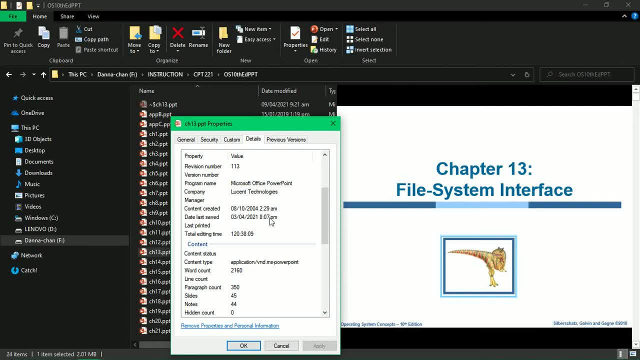 it was last saved um last april, 3, 2021, so, and also the editing time. so, again, it depends upon the, the, the, as i've told you, it depends upon the file type, because these are the other um other details of the file. okay, okay, so we're already finished with that, so 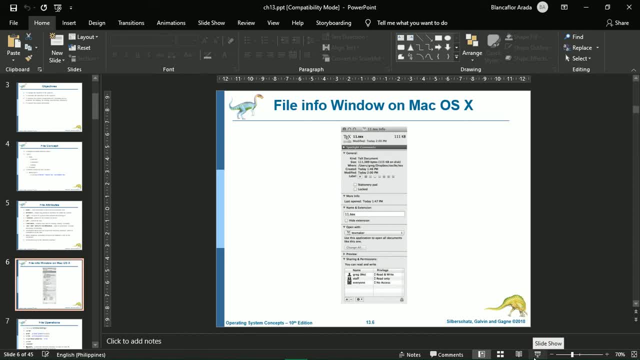 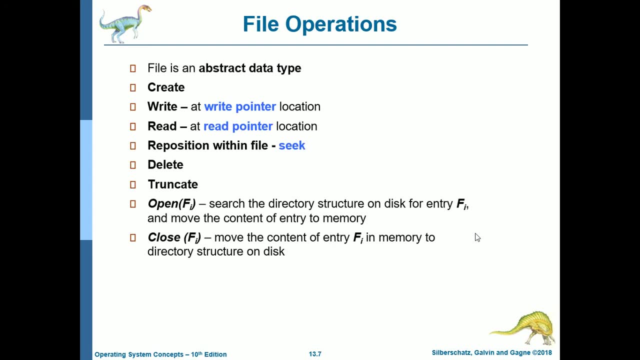 okay, okay, so we're already finished with that. so, okay, so we're already finished with that. so mac os has their own versions and, of course, windows has also its own version, okay. next is we have file operations, so file is an abstract data type, and then these are the common. 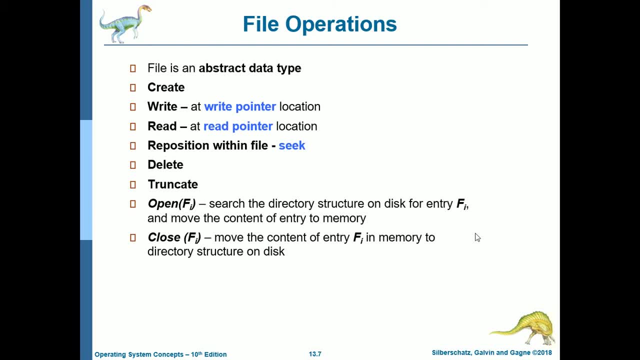 operations that is done or in a file, commonly uh file operations. that is general to all files. so of course we have create- so you know how to create a file- and your document and your slideshow presentation, a new excel file and the next is we have, right at right pointer location and then 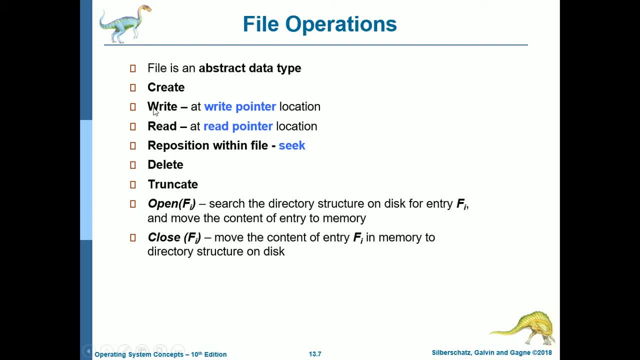 specifically write and read is if the file is loaded in memory and then read is at read pointer location and then reposition within file is we're going to use the seek and then also, with reposition within the file, the file is loaded in memory and of course, we can delete a file. okay, we can delete. 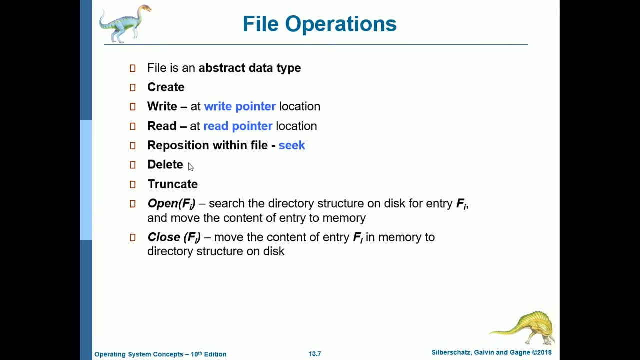 user files and then we can also visit the folder. and we can also visit the folder and we can also- actually we can- delete also system files. but we have to be careful because um, specifically files that is in drive c, because if you're going to delete that and you don't know the consequences, 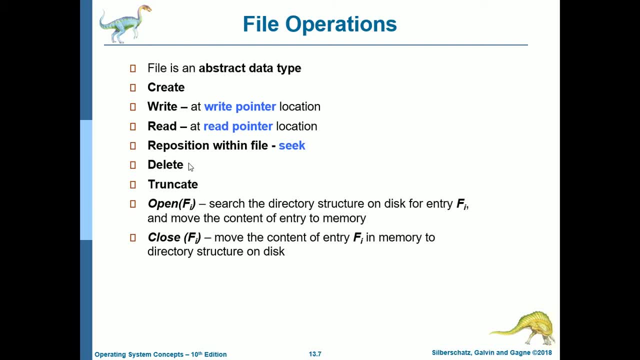 so better safe than sorry, do not delete it. but of course you can delete the user created files. and then what is truncate? so the user may want to erase the contents of a file but keep its attributes, and then we also have this file operations open and then the parameter is: 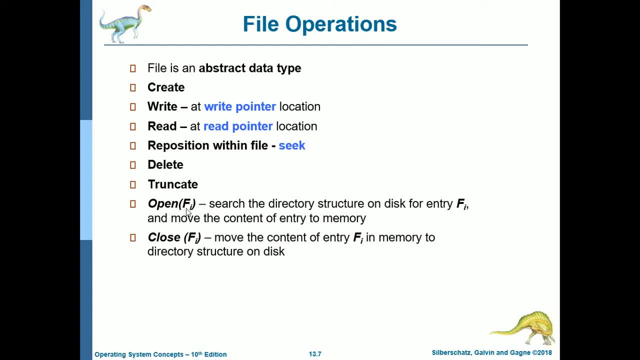 f sub i or any file that is existing. so search the directory structure on disk for entry f sub i and move the content of entry to memory you can imagine open, such as example: you're going to open a file, you're going to click the icon of that file, so by clicking that you are invoking the. 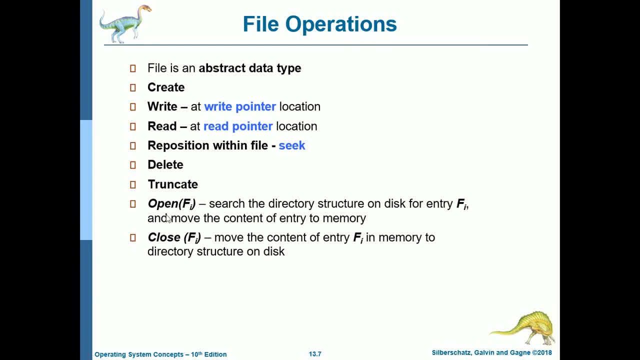 function open and then the parameter is the file that you have clicked and of course we have another. we have close. we can only invoke the close um system call or function if the file is open, of course. you cannot close if there's nothing to close, of course. so we have this one move, the. 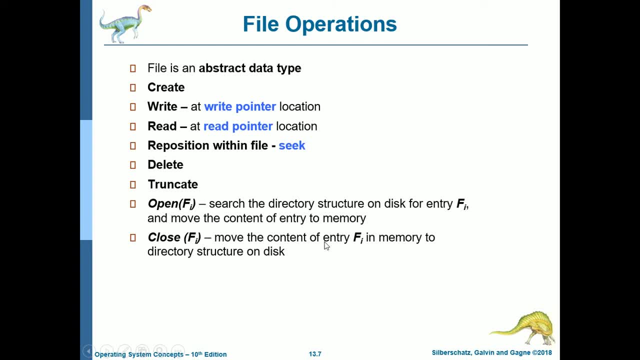 content of entry f, sub i in memory to directory structure on disk. so it's like, for example, you're doing your file and then if you want to save and exit or close, so clicking the exit or the close button, that will invoke the command close and then, of course, the file that you are closing. of course, 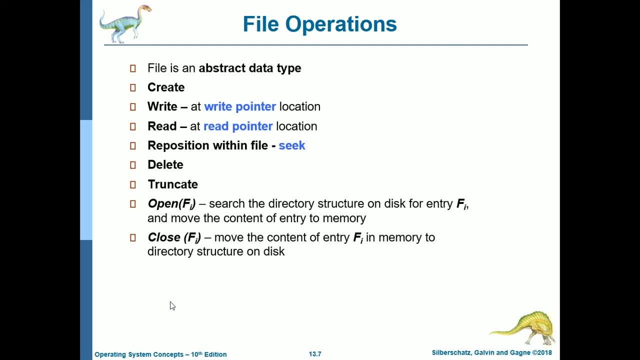 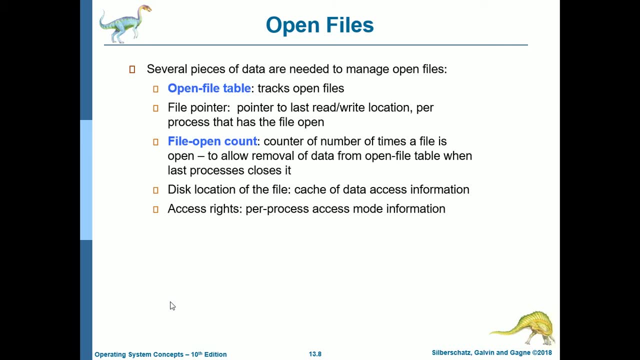 so these are the common file operations, okay, okay. next is we have open files. so so several pieces of data are needed to manage open files. so, for open files, there is an open file table which tracks open files, of course. and then we also have file pointer: pointer to last read or write location. 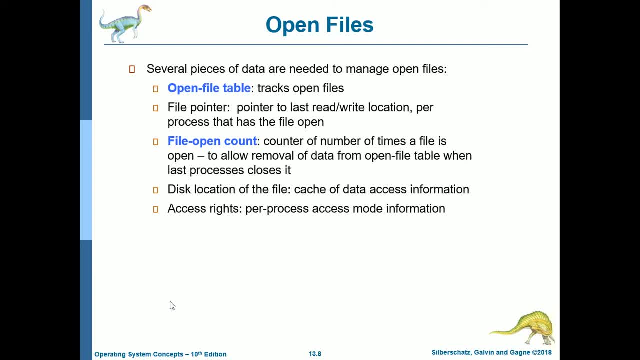 per process that has deep file open. and then we also have the file open count counter of number of times a file is open to allow removal of data from open file table when last processes closes it. and then disk location of the file, cache of data, access information and then access rights per. 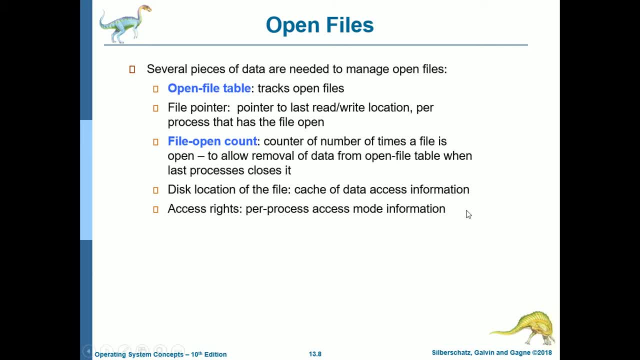 process, access mode information. so we will be dealing with the access rights and then, of course, the disk location. as you can already see, with the properties we have already the path name where the file is located. so how about this file? open count- okay, so let's illustrate a file: open count. okay. 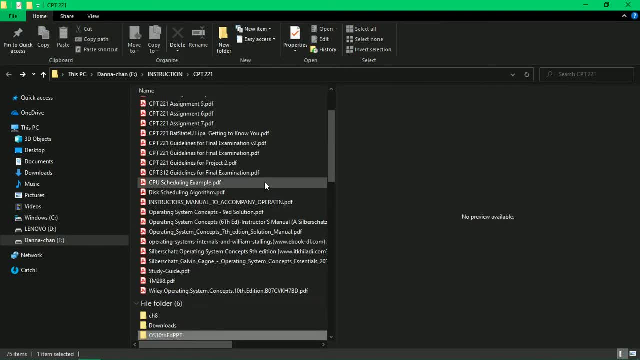 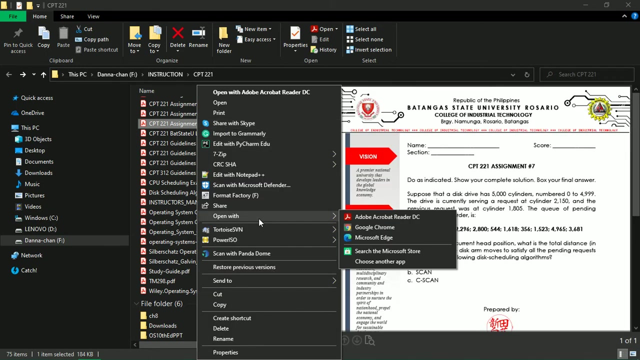 again. let's go back with our folder, with our subject folder, again with our assignment. we're going to open it in, of course, the default program, so let's wait to load the context menu. sorry for the lag, okay, so let's open it, of course, by the default program, the adobe acrobat reader. 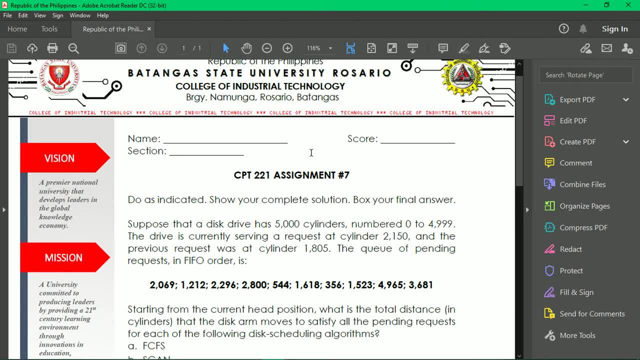 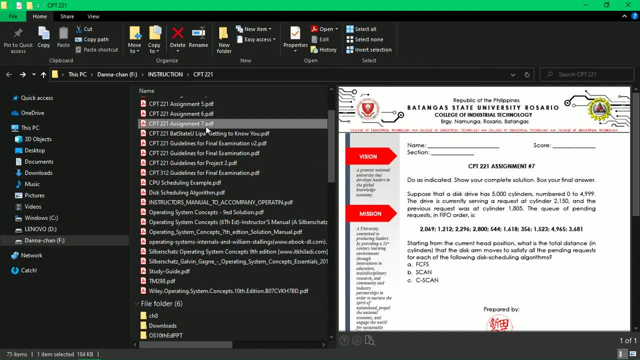 and then the other one. so we've already- uh, you already are familiar with this assignment, if you are. and then next is: let's open it with. let's open it with a browser. okay, this is already open, and then we just need to make a文 like window. 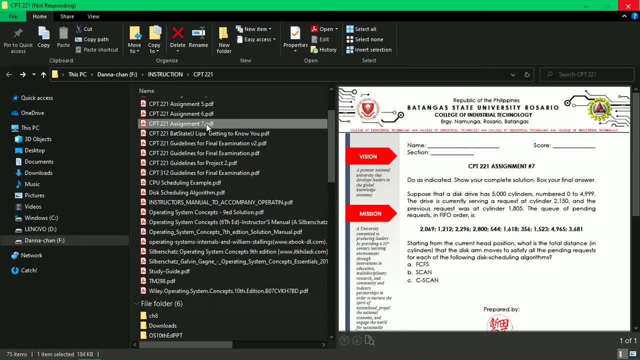 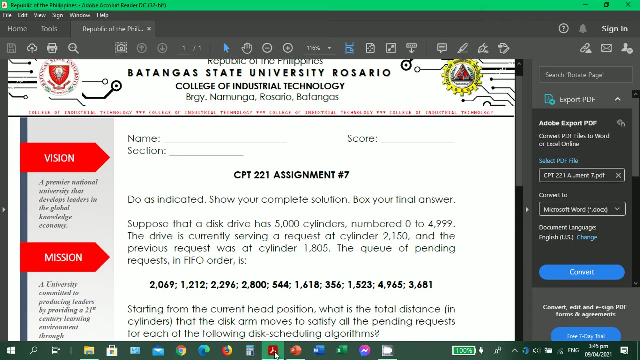 so, yeah, it has done what we asked it to. okay, let's see what happen. um adobe GX slowdown. good, we just need to wait. wait. okay, this is already open and then we just need to leave the interface concepts. viens struggle to close. I'm sorry because my laptop started to stall earlier, but I'll add something next time. now. 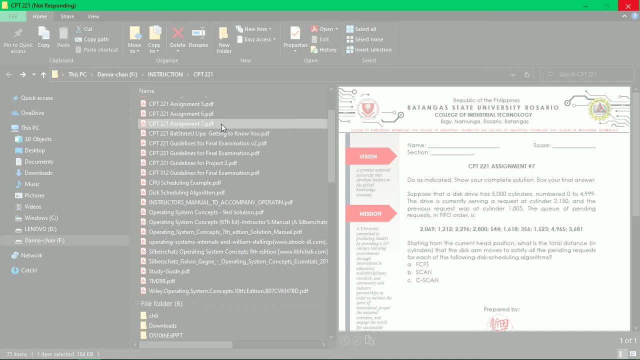 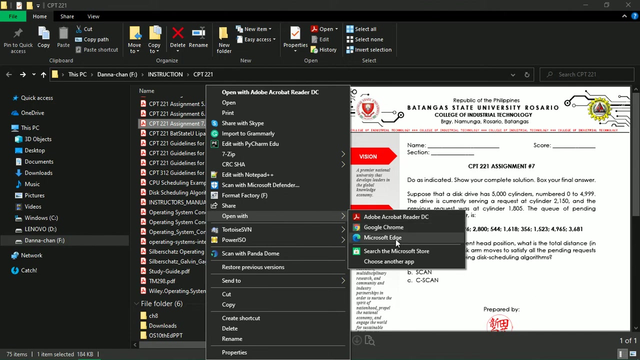 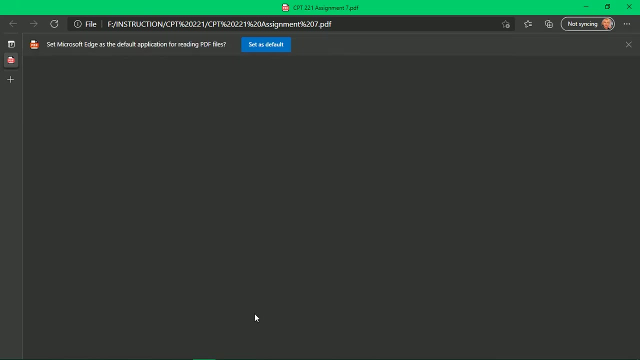 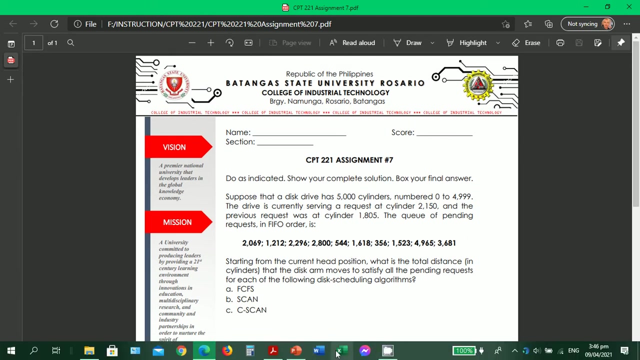 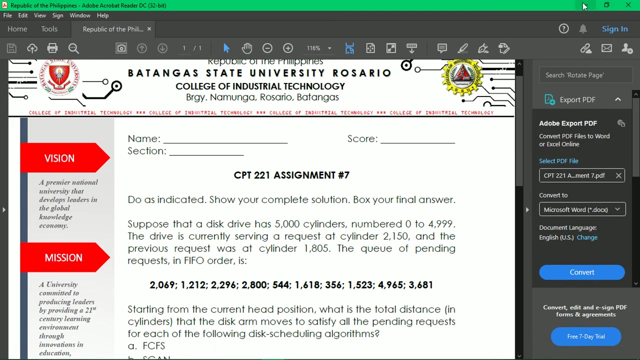 need to wait for my forever, my ever fast computer. okay, we're still waiting, okay, thank you. okay, so let's open it with microsoft edge. okay, we can possibly open one file in with two different applications. so first is we open it in the default, which is the adobe acrobat reader, and we can also open it. 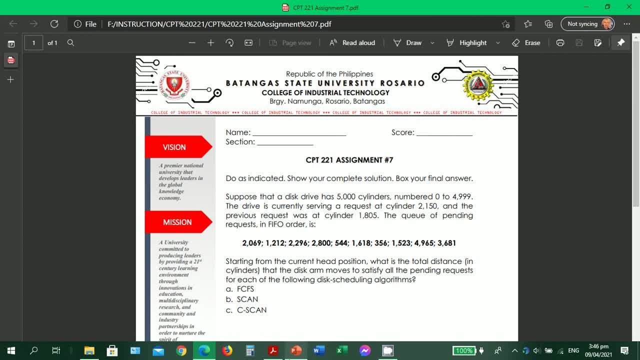 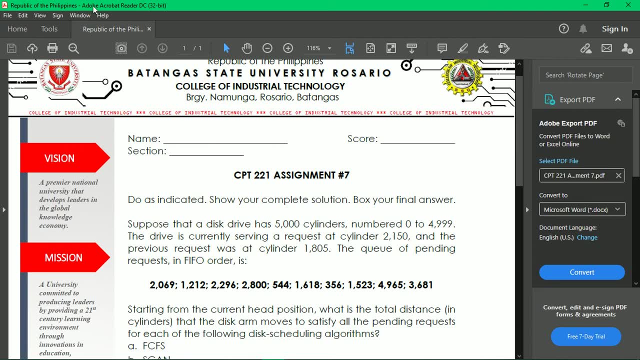 in a browser. as you can see, there are just the same files. so, for example, if you're going to edit anything- because you can actually edit pdf now in, for example, this in adobe acrobat reader- so actually if you open this file in two different applications, so the the mode is in read. 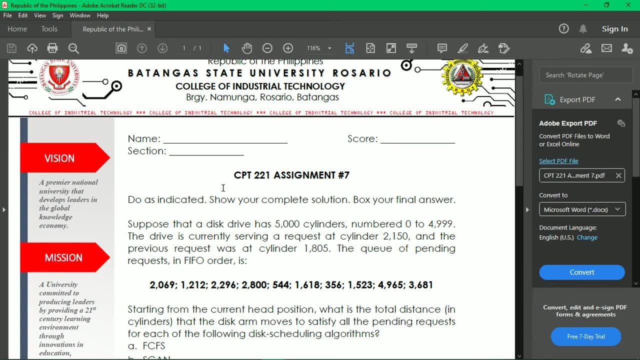 on only mode. so if you're going to edit- edit this- you will be warned that you have to close the other applications. that has this another instance of the file opened because you're going to edit it. so there is actually a discussion in the presentation that for for you to edit a file. 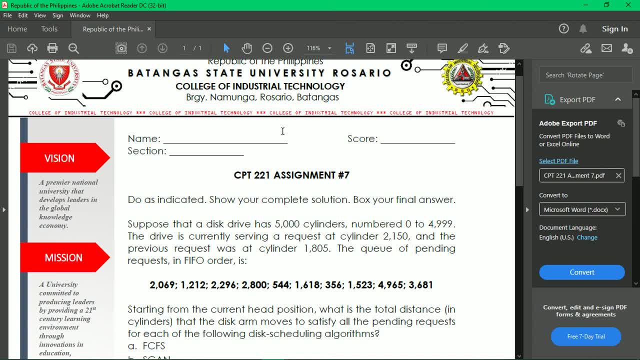 it must be exclusively open to one application only. actually, this can be open in any other application. that is, of course, applicable with us a certain file type. so for this mode. so since, even though this is a, a portable document file, this are all in read only mode. 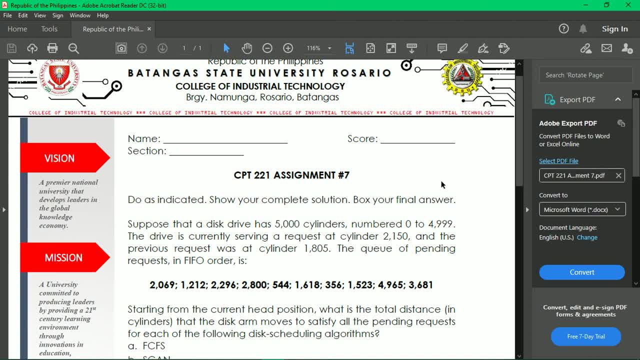 you can. you can open concurrent copies of that in read only mode without, without any modification or editing of the file. so what i am illustrating here is cambio file open count. so in our system, Fuhrman's sociales file open count, sontизing file number one. file number one file, the cutting out. 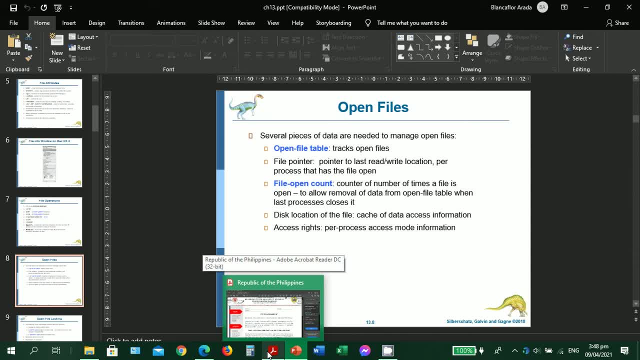 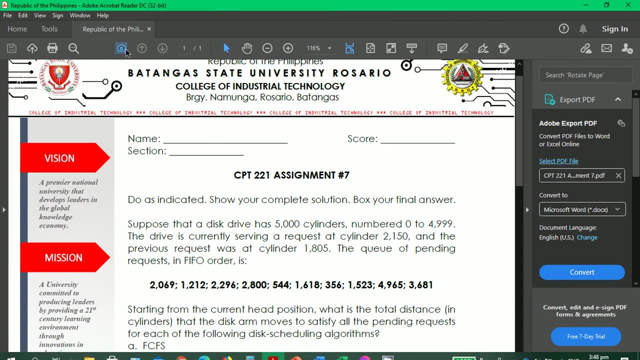 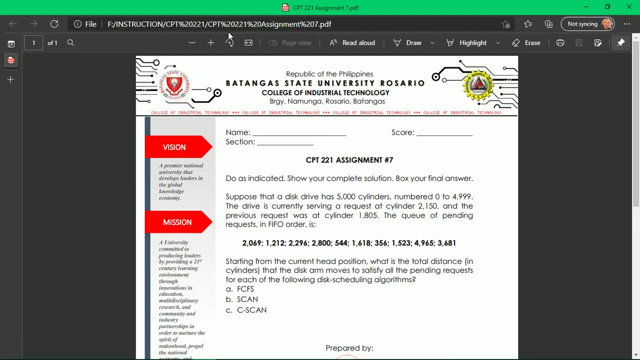 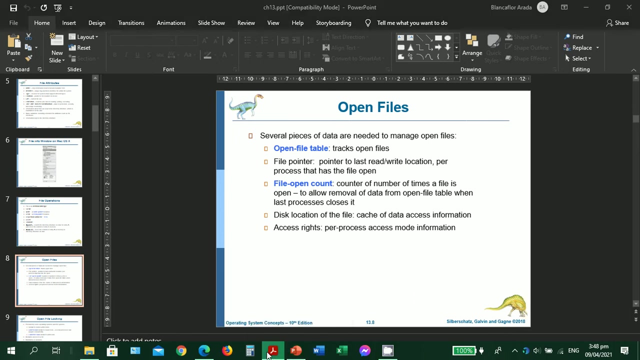 our system, in this computer system, so we can see here that um this file, the this file is, we have um a specific file, the name is cpt221, assignment seven is opened in two different applications. so that's we, that is, we have the file open, count. okay. so we can close it now, because i've already shown you that it is possible to open. 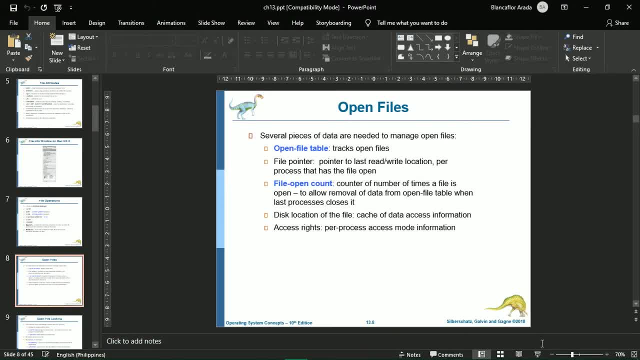 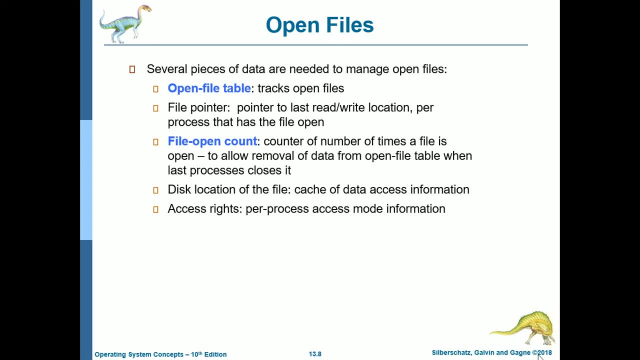 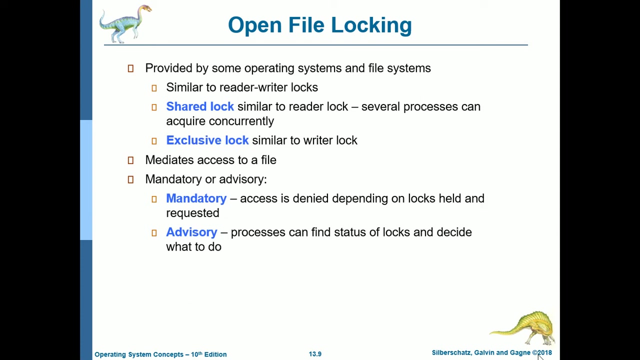 the same file with different applications. as long as the, the application is correct, is i mean correct- it can really open that particular file type. okay. next is we have: okay, next is we have open file locking, so provided by some operating systems and file systems. so it is similar. 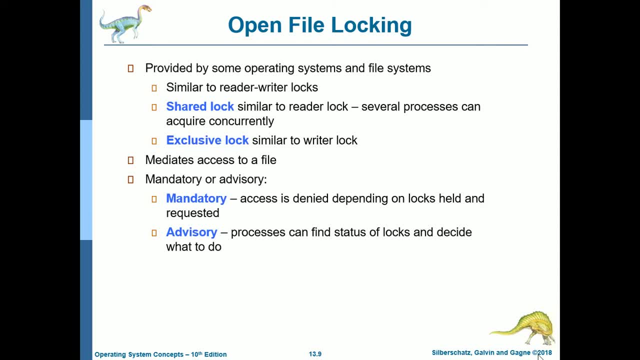 to reader writer locks. so we have a shared lock, similar similar to reader lock, several processes can acquire concurrently. this is what i'm saying when i opened that same file in two different applications, that uh, those um application. they have shared luck because, of course, if your purpose is just to read, it's just to view the file, but if you want to edit it, 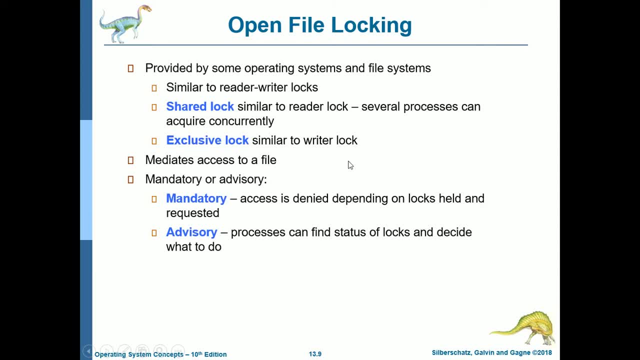 it's really going to be a lock, so it will have exclusive lock similar similar to writer lock. so, for example, if you really want to edit um, there will be a warning that you have to close all the other instances of the file for the for the changes to be effect in effect. okay, next is. 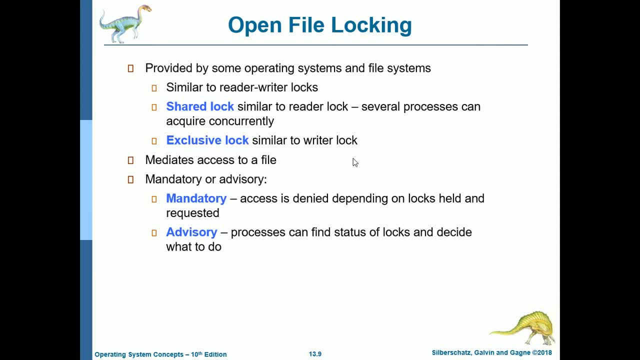 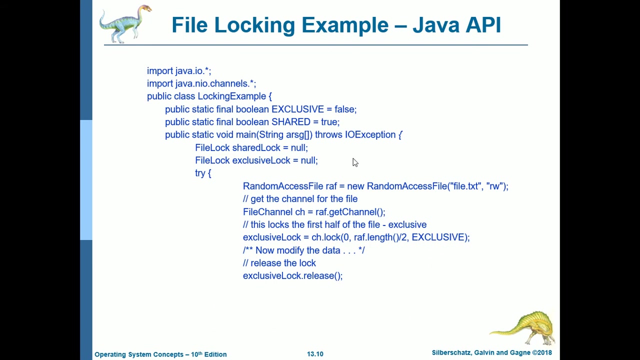 mediates access to a file, the open file locking. it can be mandatory or advisory. so for mandatory access is denied depending on locks held and requested, And then we have advisory processes can find status of locks and decide what to do. Okay, so for this code, so a file locking example by using the Java API. 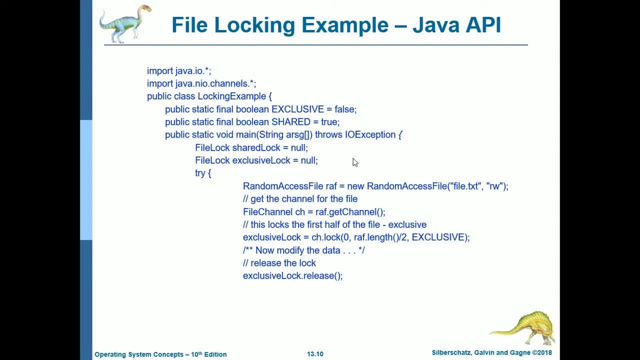 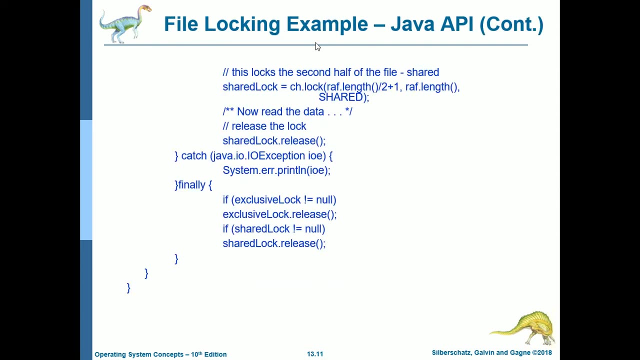 So this illustrates file locking in Java. This program acquires two locks on the file filetxt. So this first half, so the lock for the first half of the file is an exclusive lock And then for the second half of the file is a shared lock. 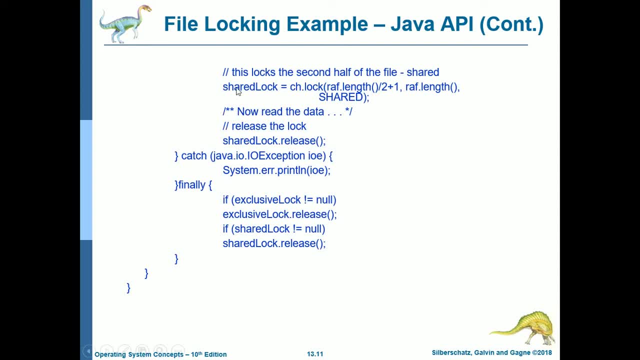 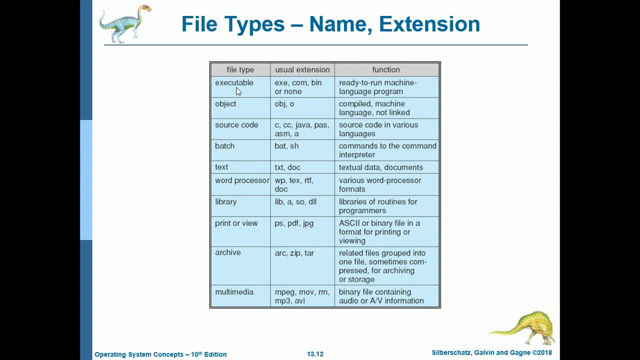 So, as you can see, we have this shared lock. Okay, so next is we have a table for file types, their names and then extension. So these are the general file types existing in a computer system. So we have first the executable. 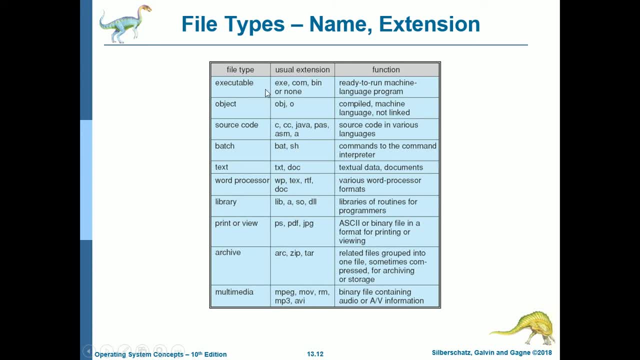 So the usual extension is the exe, So exe, Of course executable, exe, then com, command, then bin is binary, or it can be. there is a file that has no extension at all, But for Windows it comes with exe, com and bin. maybe for none. 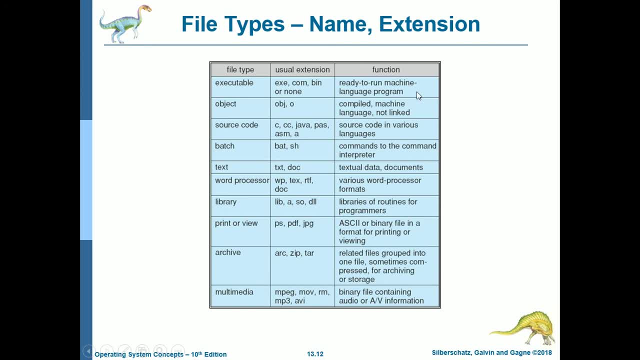 These are for other operating systems. So the function of executable is ready to run machine language program. And then next is we have the object, We have the obj and then o. So these are the compiled machine language, not linked. So obj is produced for example in Turbo C. 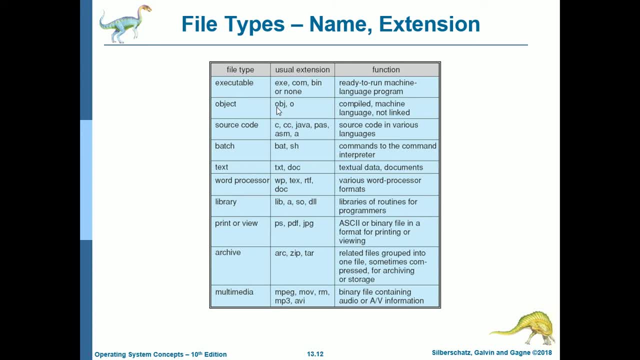 This is evident in Turbo C. If you're going to compile your code, it will produce the obj file of your source code And then next is we have the source code. It can be for C And then we have for C++. 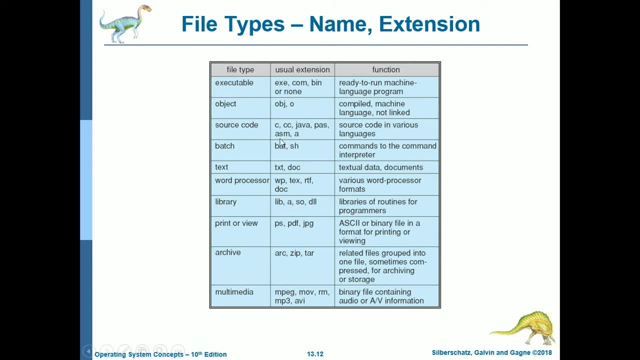 And then we have for Java, We have for Pascal, We have asm for assembly language programming, And then a is for static libraries. So these are the source code in various languages. So of course, these are not limited to this one, because there are other programming languages that exist, such as, for example, Python. 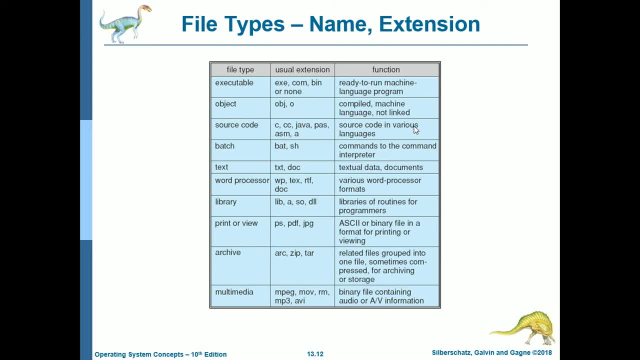 That's py, So it depends upon the programming languages that you are using, So this is not limited just for C, Java, Pascal, assembly language. Next is we have the batch, So it is in bat or sh or shell. 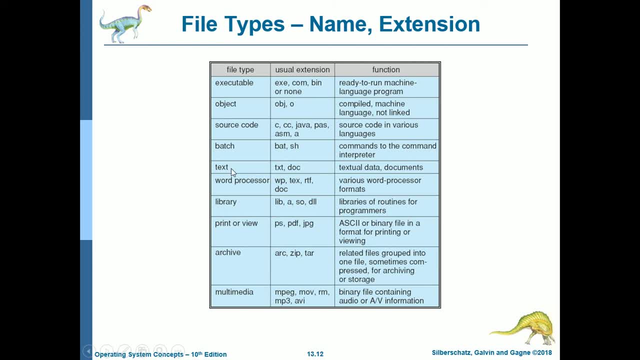 So commands to the command interpreter. And then for text file type: of course the file name extension is txt or doc, or for more modern it's docx. So the function is textual data or documents. And then for word processors. 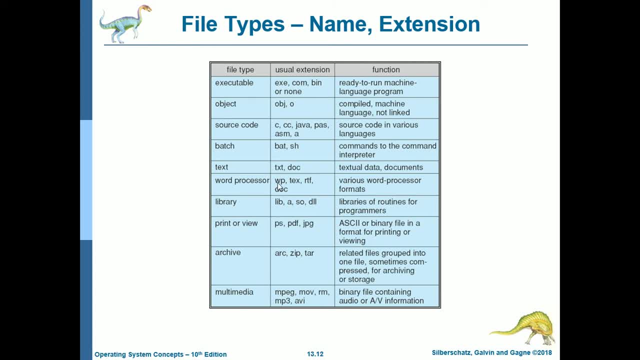 So WP, wp is. this is the file type of Corel WordPerfect. This is specific. It's also, of course, a word processor file type, So the tex. there are other file type such as this: And then we also have the rtf, which is rich text format. 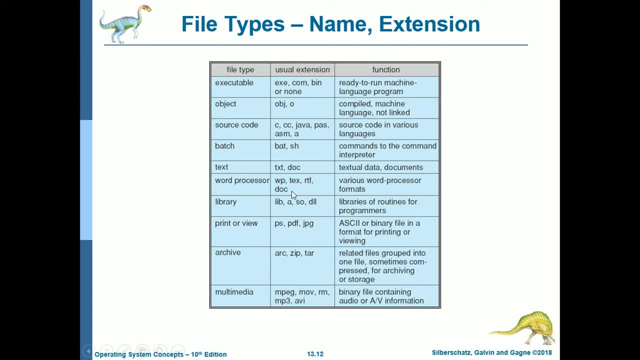 And then, of course, just the same with text, doc or docx, So various word processor formats, And then for a library, So we have live, of course It's easier to distinguish, And then a just the same with the source code, static library. 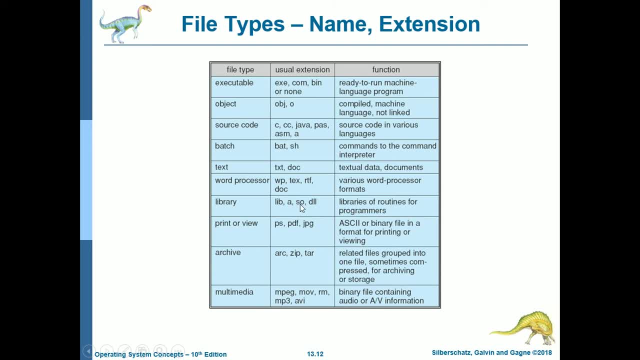 so is shared object. This is specifically in Linux. And then we have dll for dynamic link library. So this is typically with the applications as of today. So libraries of routines for programmers And then for print or view file type, dll for dynamic link library. 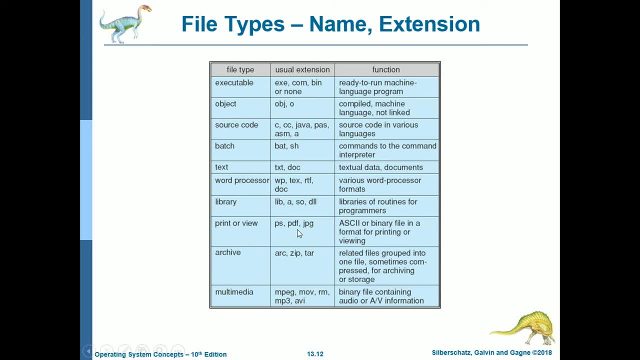 And then we have ps, so pdf or jpg. So ps may be in, of course, in Photoshop, And then pdf, of course, is Adobe Acrobat Reader Portable document file And jpg is an image file. 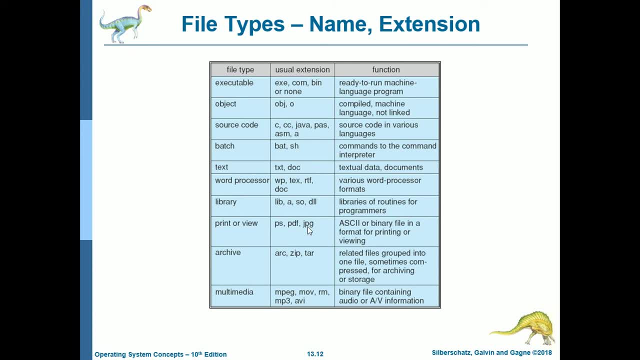 So ASCII or binary file in a format for printing or viewing. So again, this is not limited to jpg, because there are also other image or picture file types, Such as gif, png, bmp, tiff. So we have many file types for images. 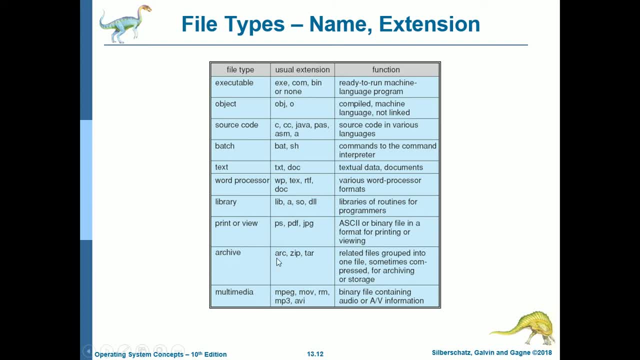 And then we have archive. We have, of course, arc, zip and tar. So tar it came from the name with tape, archive files, So that's why it's called tar, So related files grouped into one file. 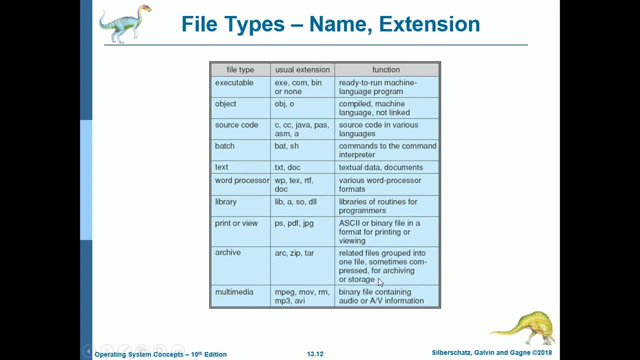 Sometimes compressed, for archiving or storage, And then for multimedia. we have mpeg, mov or movie rm- rm is for real media files- And then, of course, for music, specifically music. this is mp3 and then avi. 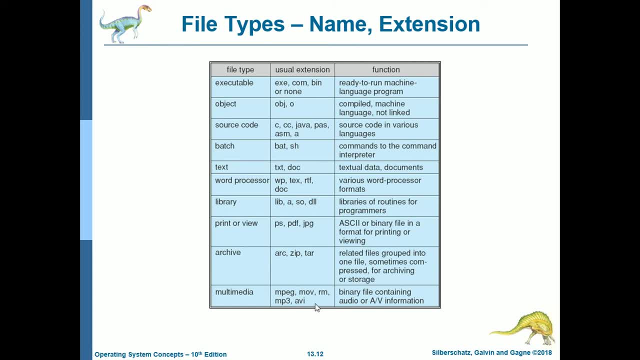 So binary file containing audio or audiovisual information, But again, this is not limited to this one, because we know other file types, Such as mkv or ogg. what other files We have? mpg? So there are many, many files. that is, for example, for audio or for videos. 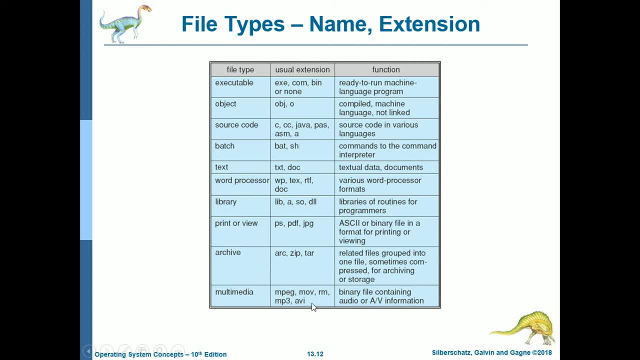 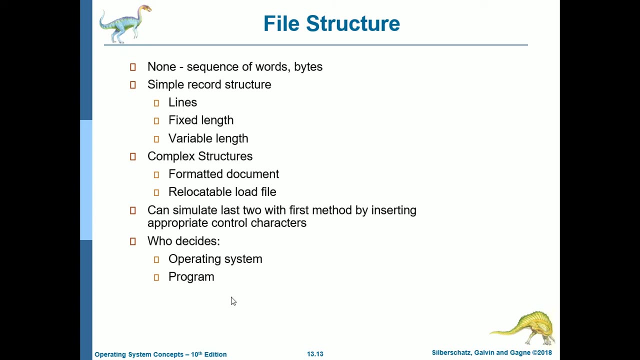 So this is file type multimedia. So music and movies or videos are categorized as multimedia. So this is a multimedia file type. Okay, next is we have the file structure. So file structure can be none, or a sequence of words or bytes, And then it can also be a simple record structure. 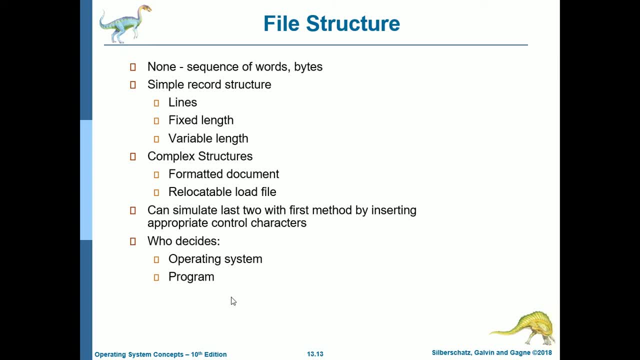 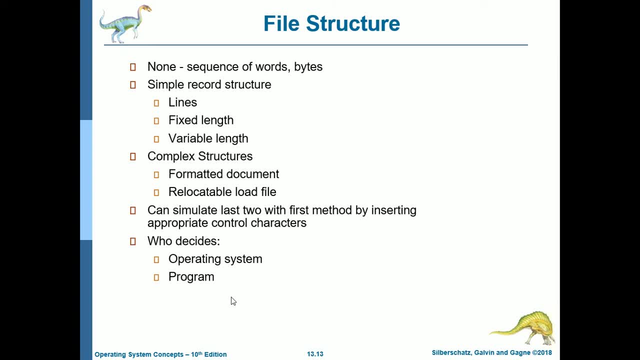 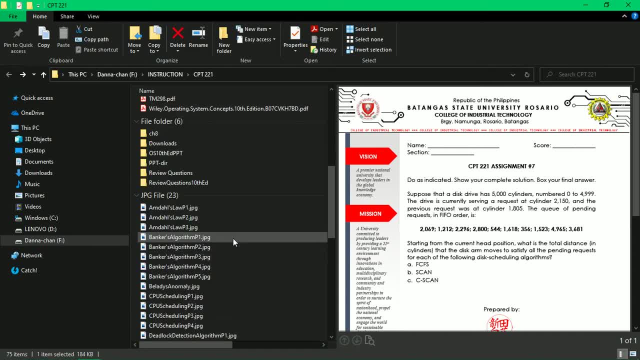 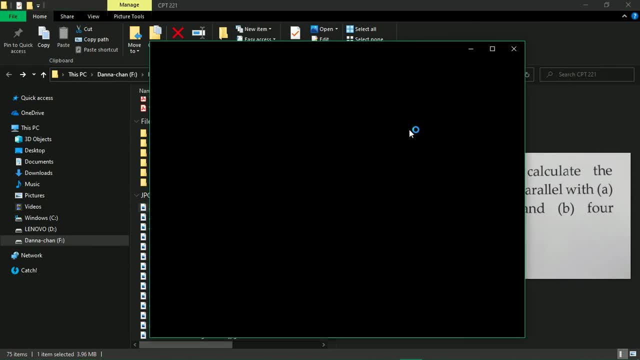 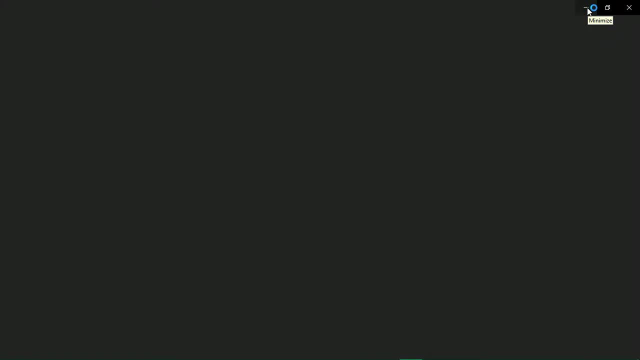 So let's get a go again with our folder. Okay, we have this. If you are familiar with the picture, So of course, if I'm going to click it, So the default program here is, of course, again, let's wait to load the picture. 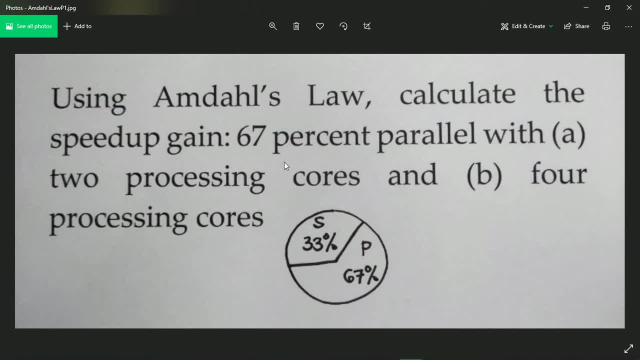 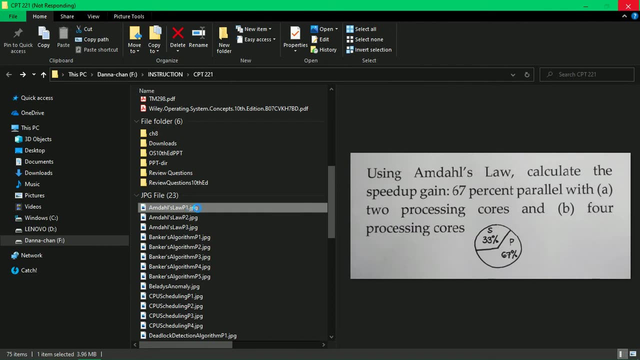 In memory, Okay, so if you can remember, this is one of the previous lesson, past lesson. So, of course, if I'm going to click it, So again, let's right click it again. Please wait for loading again. Sorry for the speed. 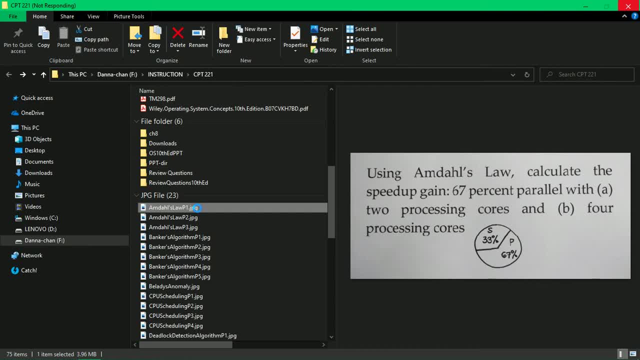 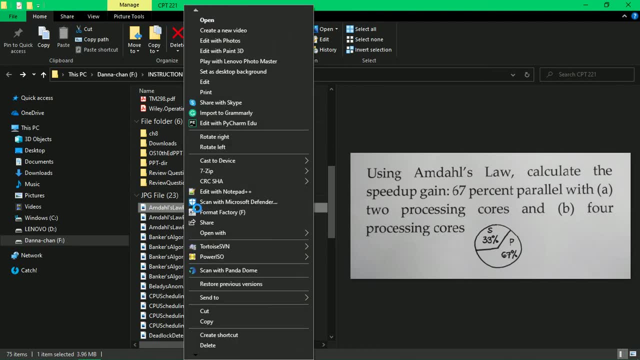 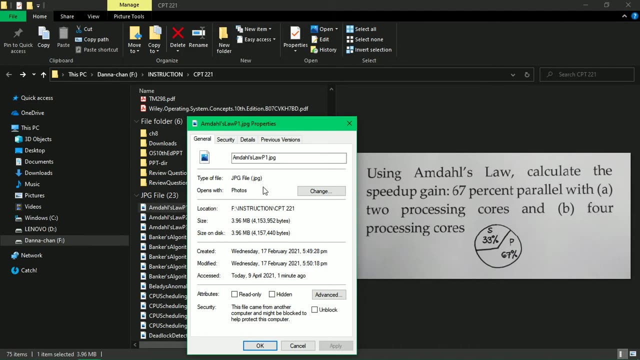 Okay, Counting. Okay. So we're done today. Okay, okay, okay. so let's click properties. so, okay. so this is our default application or program to open that jpg and, as i've told you, with the file pointer location. so this is the file pointer location, okay, okay. so, since we've opened it, it is opened with: 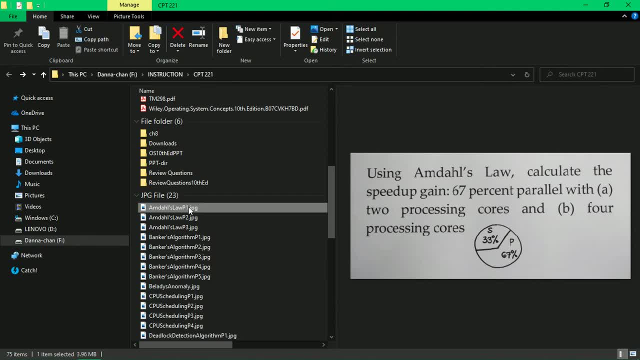 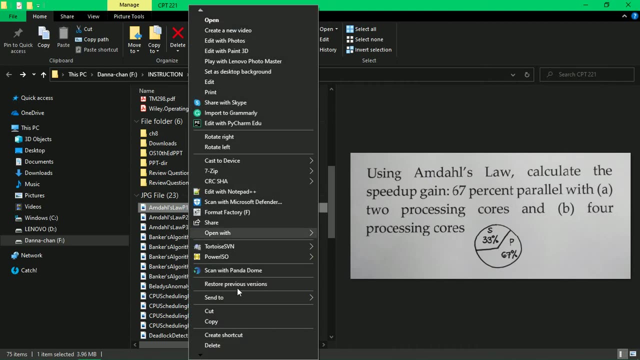 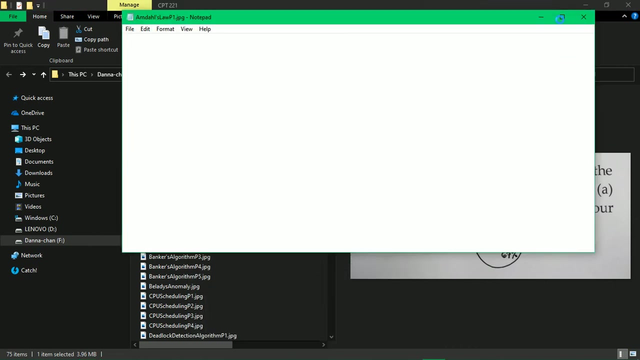 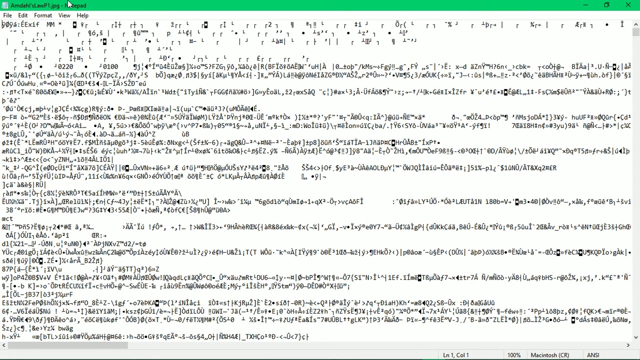 photos, applications. what if we're going to open it in a notepad? okay, okay, okay, okay, okay. so what if you want to? okay, just one, just be curious, what will be the okay, actually, notepad can open anything. so this is the amdals law p1.jpg. 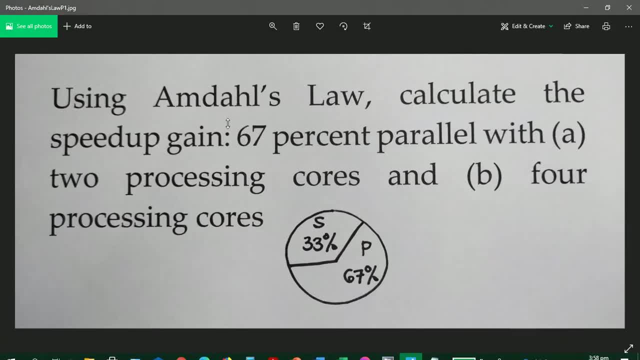 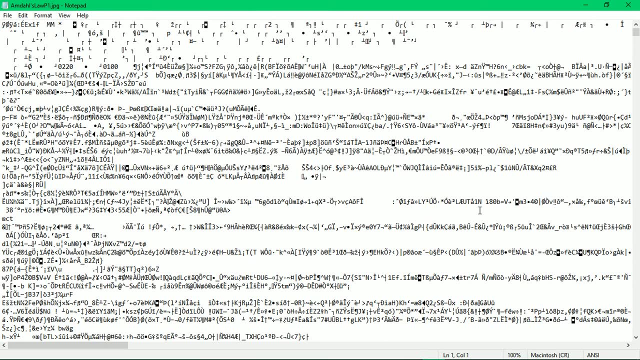 different from what we have seen here. it's actually a picture, but of course, if you're going to put it in a notepad, um this, this incorrigible um characters here, so for us we do not understand this. but if it is going to be processed by the computer, so actually this is the. 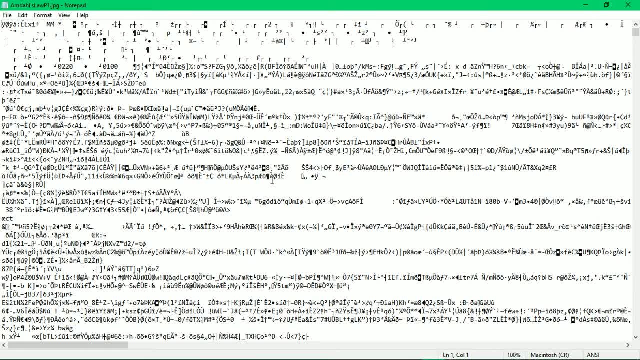 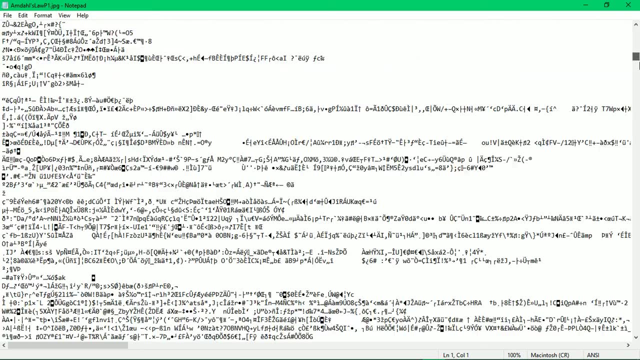 content of the picture file. so for us, uh, if you're going to open it with the right application, we can see the picture, but, of course, if you're going to open it in an application that is not meant to open that particular file, of type of file, you can see this um, these characters. so please don't edit. 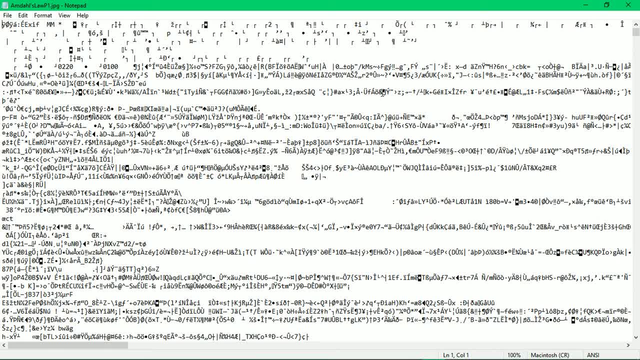 anything, because if you will edit anything, you will not be able to see the picture. so if you're going to edit, even the smallest character, made made your uh file corrupted. so this is what i've been telling. so for formatted documents- they are. they have specific applications to open with you. 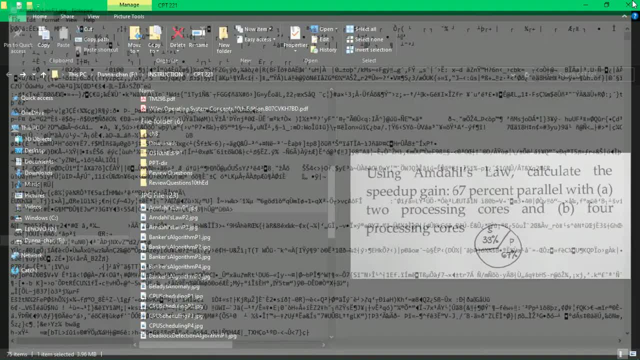 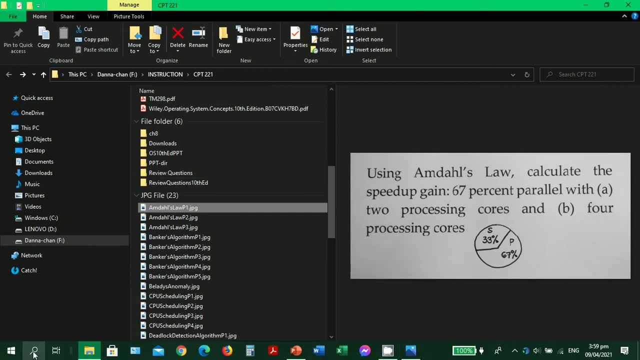 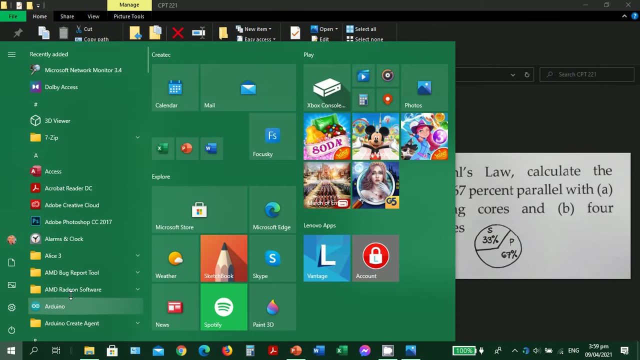 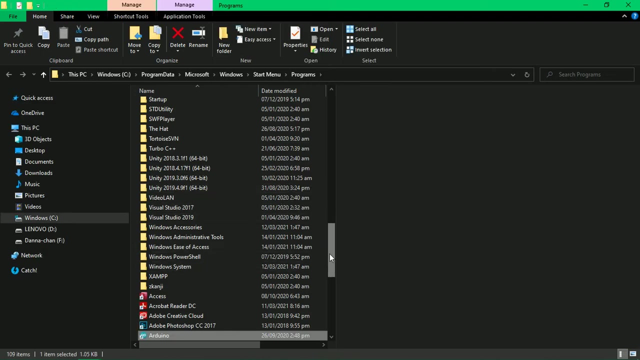 cannot open it to any other file. okay, so i have another illustration here for the file pointer, before i forget. so, for file pointers, for example, we have programs here, okay. so, for example, we have this one arduino: okay, this arduino here is what? okay, this arduino here is actually a shortcut, okay. so this actually, of course, if you're going, 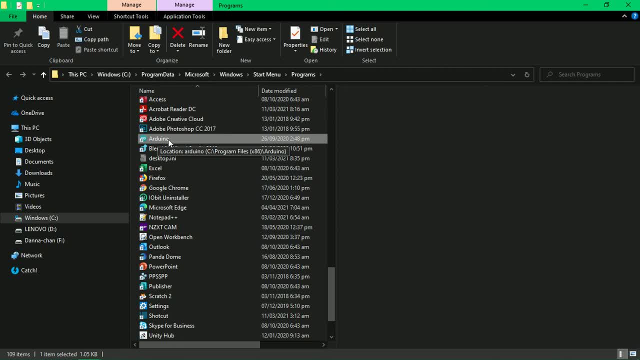 to create a shortcut. it is really not the actual file, but it's only a point pointer to that uh file that you want to open. so where's this? the original um arduino application is located. so this is the path name. so it is in the start menu program. so again. 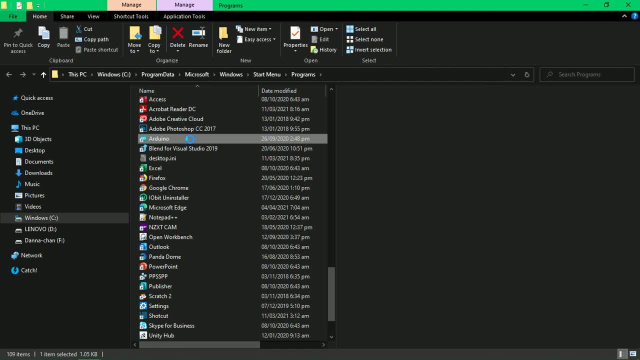 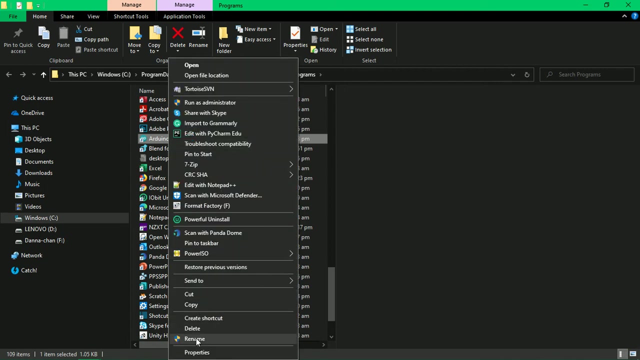 please wait for the context menu to to load. okay, let's wait for it. i'm really very embarrassed with my computer, with my computer, because even the context menu, it takes a while to appear. okay, let's count. okay, thank you very much, okay, properties. so as you can see, uh, the properties for an actual file is different. 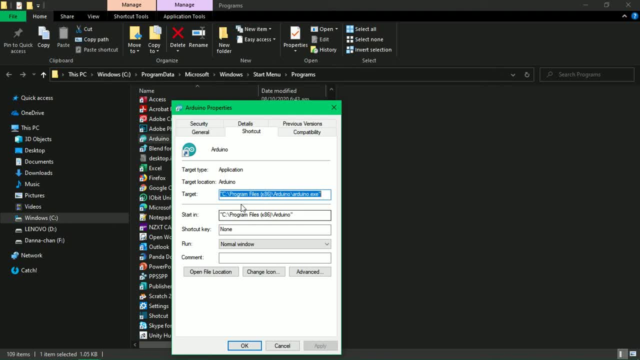 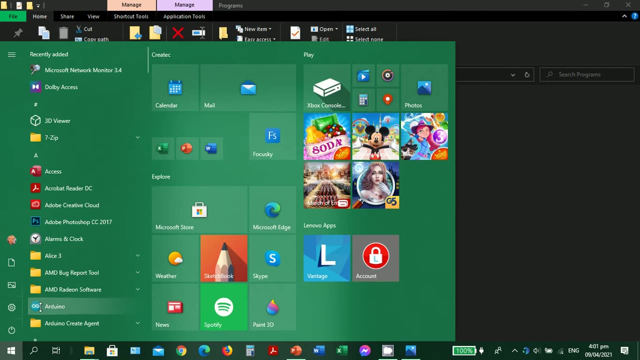 with a shortcut file or a pointer, because you can see here that this is the location of the actual um file that you are opening. it's not really the arduino here, uh, the the ones here. it's just a shortcut, it's not the actual exe file. so again, okay. 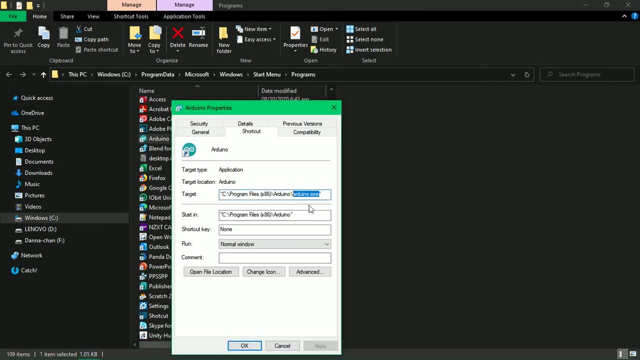 so why does windows do this? the shortcut files? so that, of course, users will not go to the actual folder, because the actual folder is not the actual folder. it's not the actual folder. it's not the actual folder. it's in. uh, very um, it's not very sensitive, it's just that, since this is, it is in. 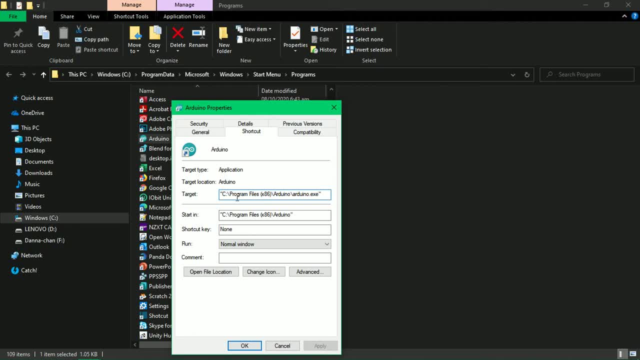 the way, inside drive c, which is the system file c for uh c program files x86. if you are just a user who do not know the, do not know that you can. you cannot just modify anything inside that folder. so, uh, let's see, we can open. of course, if you're going to open it, if you do not know the. 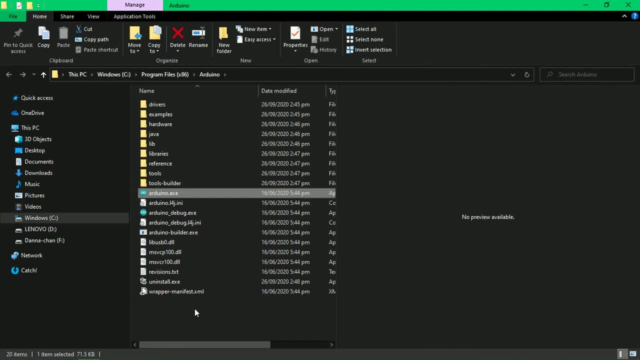 do not know what you're doing. just leave it be again. better safe than sorry. so this is the actual arduinoexe that you are, that you are always. for example, if you want to open the program arduino, this will be the program or application to be executed, specifically and of course. 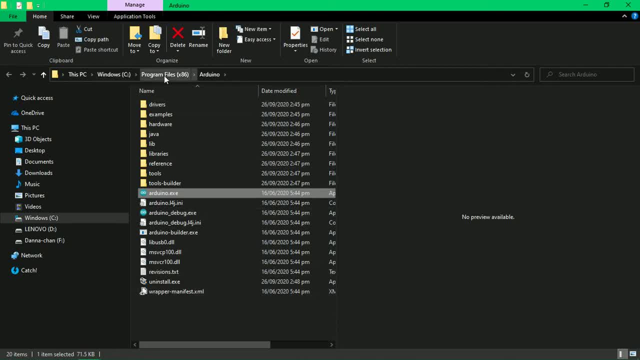 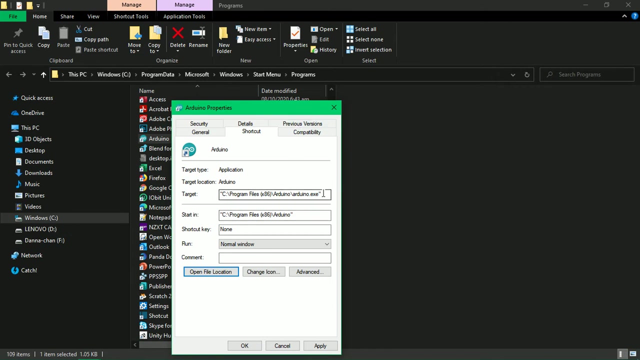 since this is under windows- and then program files, x86. so do not delete anything, modify anything, because it is considered as a system file, so that your installation of the application, example for arduino, will not be corrupted. so let's close this again. so this is the what i've been telling you. 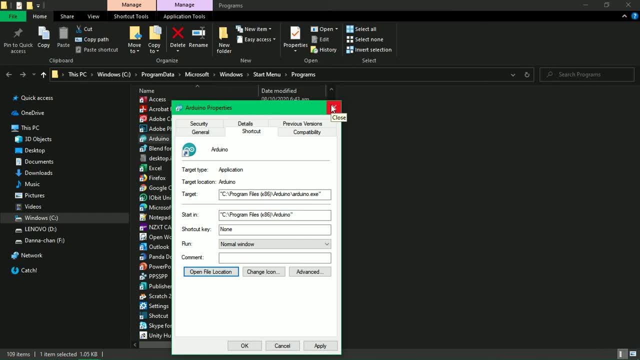 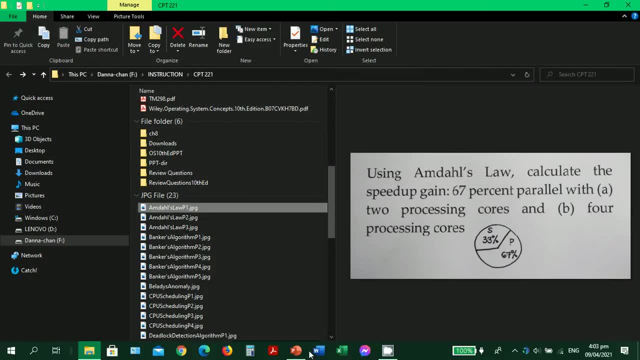 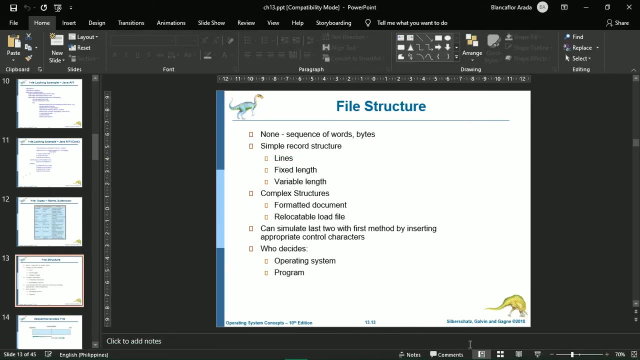 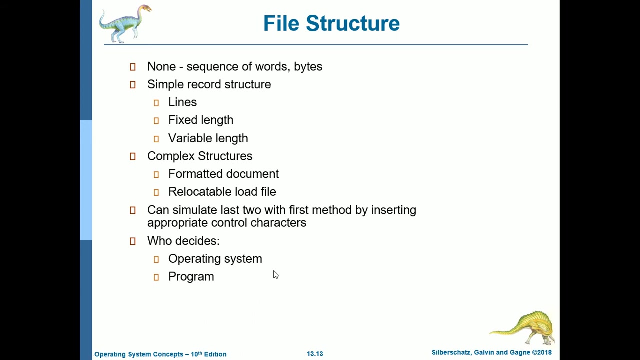 about file pointers, the shortcut links for the files. okay, let's close it now and let's return with our lesson. okay, so again, with the opening of the files, it uh, the one who decides that is the operating system in the program. so what if there is an instance that you installed um different applications, but 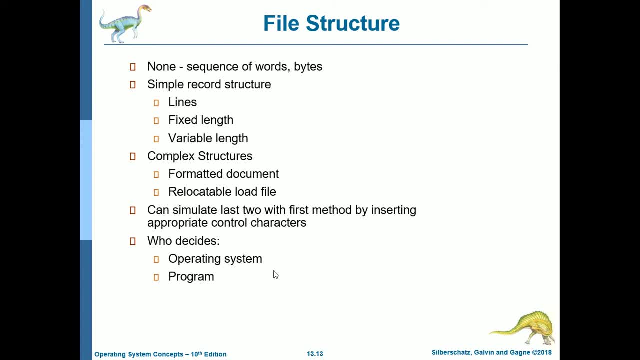 can open that same particular um file type. so it's up to you as a user if you want, for example, to open it in a in this uh application or program. so for example, um, that's that image. um, of course the default is photos applications, but if you are, 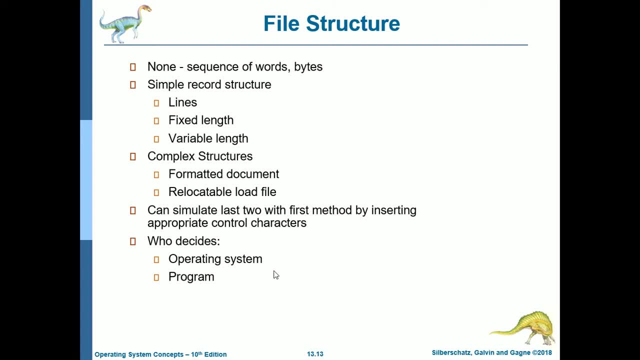 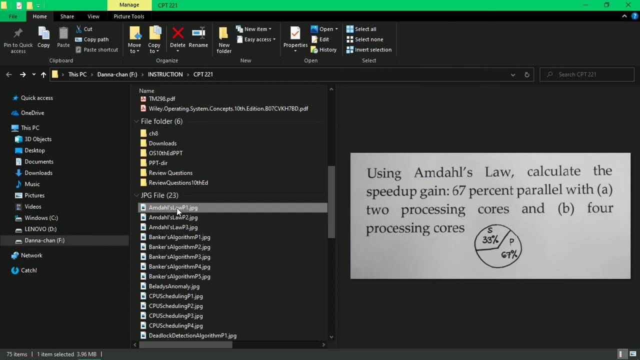 an editor. you want always to edit first your pictures. you can switch it to, you can change it into- uh, change it into adobe photoshop. so again, let's return. let's wait again, okay, ah, let's wait again for the our context menu to appear. i should, i should have already demonstrated it, right, okay? 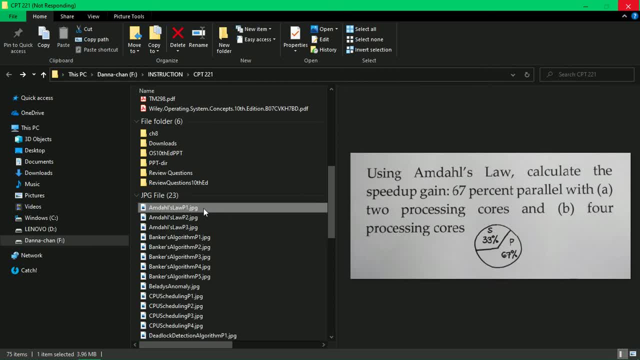 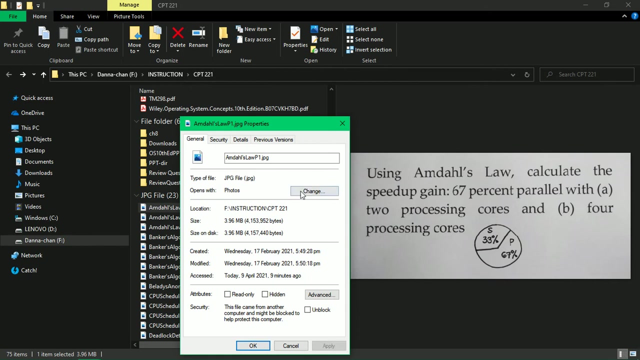 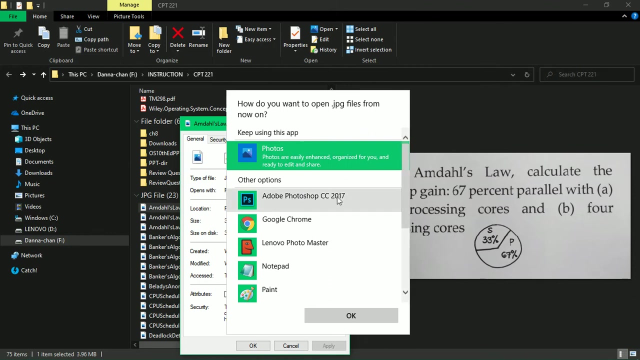 okay, let's wait. okay, maybe you're thinking i should buy a new one, right, but of course it's still functional. it still meets my expectations. okay, okay, properties: okay, so it opens with photos. actually, you can change it with, of course. yeah, this is the recommended. so you can open it by using adobe photoshop, google chrome or photo master, of course, if it's in notepad. 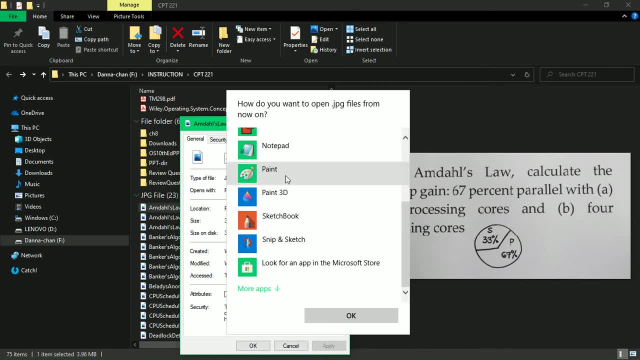 the problem is you're not going to appreciate it. or in paint, okay, as long as it is um related to image files. so opening image files is just okay, but for me, as uh, as me, as the user, i only want to view the photos. it's not i. it's not that i want to always edit it first. so the default app. 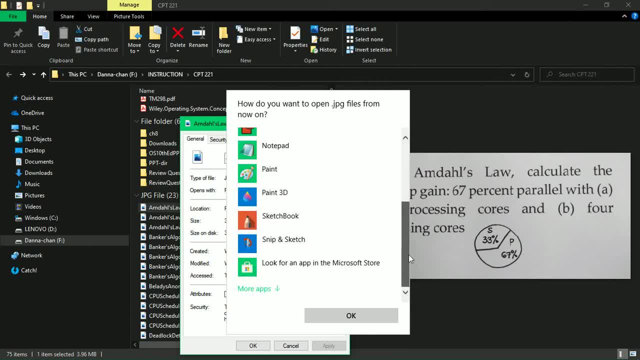 is the photos application. so again, you can change it in here and select the appropriate application. but from the list, if you still can't find what you're looking for, you can click more apps. okay. okay, you can open it in the media player. then again, you have to open it. 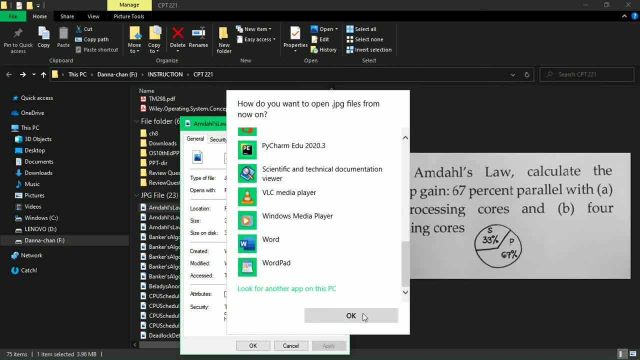 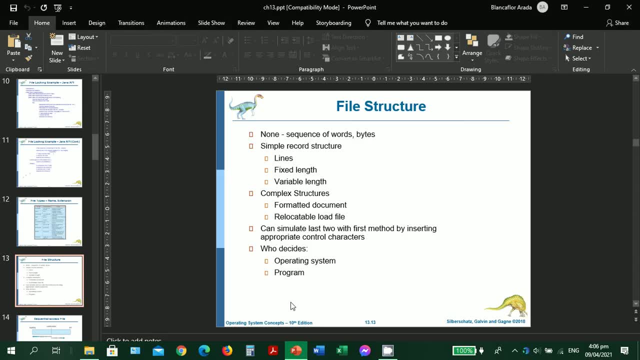 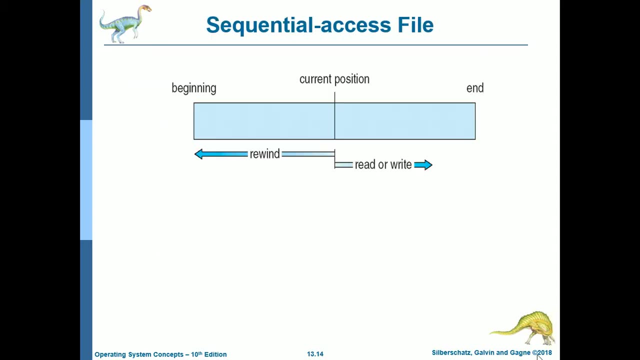 with an appropriate application program. so, since i don't want to change anything, so let it be as the default is the photos application. okay, let's continue. okay, next is we have the sequential access file. so for this one, for sequential access, so imagine it as a tape drive. so you're already here in this position. 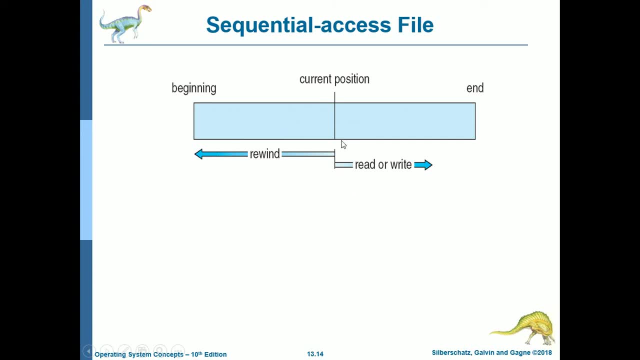 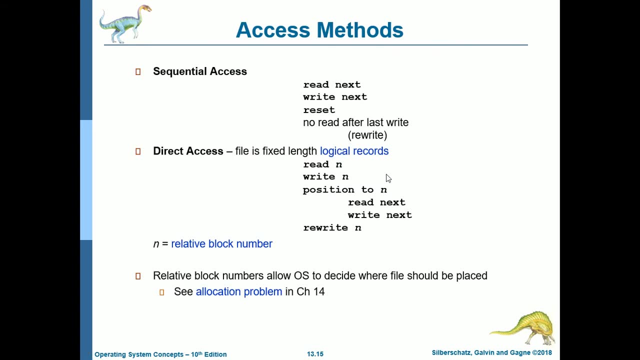 so you can rewind, go back. and for going to the end, it's either read or write. okay for access methods for uh, for file system, we have sequential access. so for sequential access, we have sequential access. so these are the typical um commands we have: read next, write next and then reset. 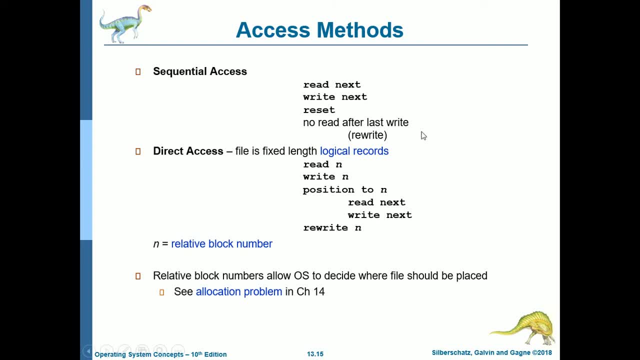 and then no. read after last, write or rewrite for direct access. so the file is fixed length. logical records: okay, the. the typical commands are: read n, write n, position to n and then just with sequential access, read next, write next and rewrite n. n is equal to relative block number. so relative block numbers allow os to decide where the file should be placed. 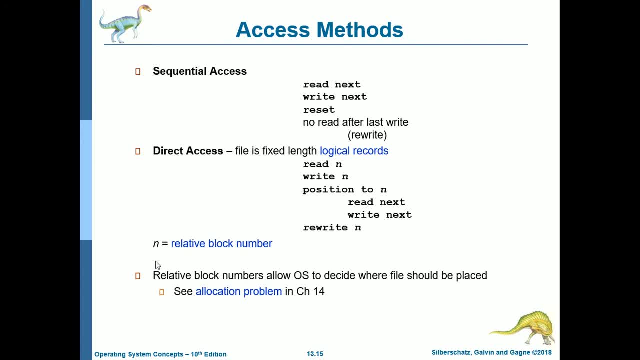 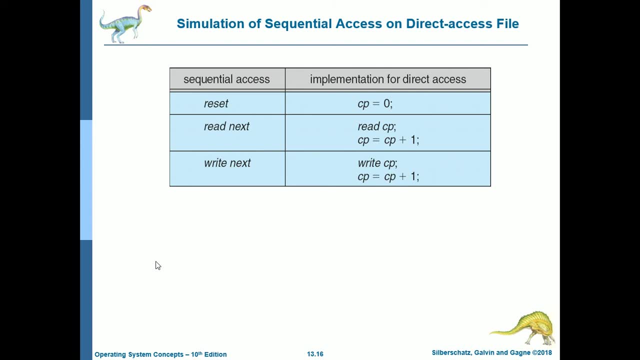 so see allocation problem in the next chapter, in chapter 14.. okay, so simulation of sequential access on direct access file. so for sequential access, so reset, the command for direct access is cp is equal to zero, because you're going to reset and then for read next, so the corresponding direct access is read cp, and then cp is equal to cp plus one. 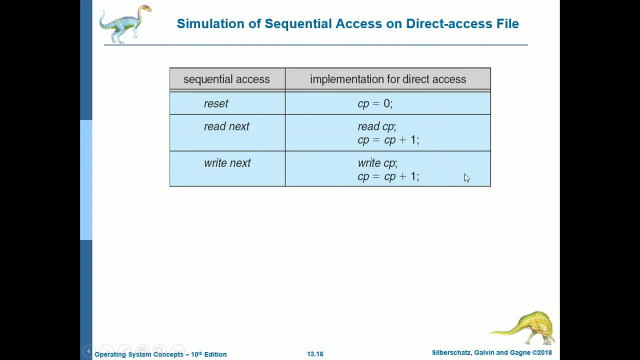 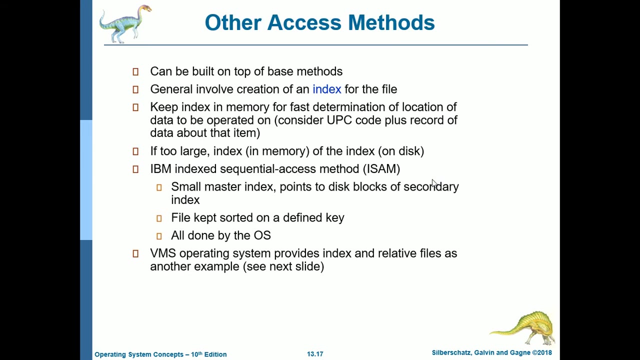 and then for the right next sequential access. its corresponding direct access is write cp and then update cp. so cp is equal to cp plus one. you're going to add one value to cp, okay. next is we have other access methods, so can be built on top of base. 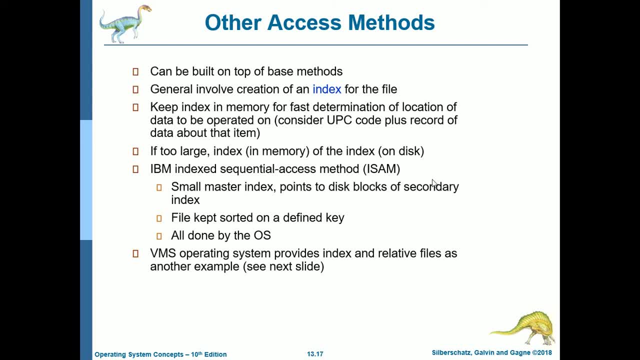 methods so generally involve creation of an index for the file. so keep index in memory for fast determination of location of data to be operated on. so consider upc code plus a record of data about that item. so if it is too large, index in memory of the index and then on disk and then ibm. 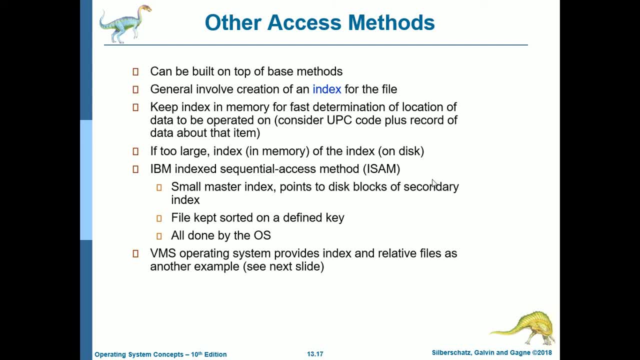 has index sequential access method or isam, so small master index points to disk blocks of secondary index and then file kept sorted on a defined key and all done by the operating system and the vms operating system. this is another, of course. operating system provides index and 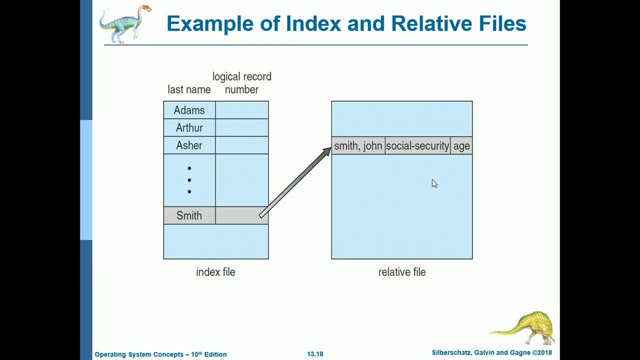 relative files as another example. so, for example, of a relative of index and relative files. so the index file contains list, and then, for example, this, this particular file. so in the relative file, this contains the whole um contents of this, um example: smith. uh, you're looking for this with the last name, smith. 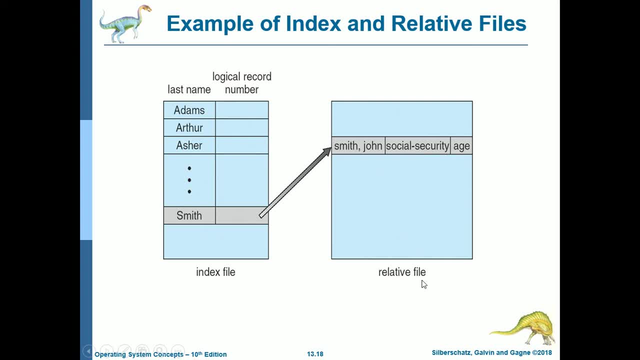 so it contains all the information about john smith in the relative file. so for using index, it's faster because this is listed and, uh, if you're going to look for a file instead in the relative file, because of course it will take a longer time to look for. 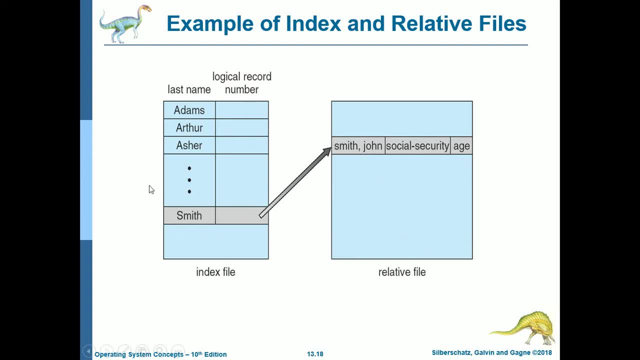 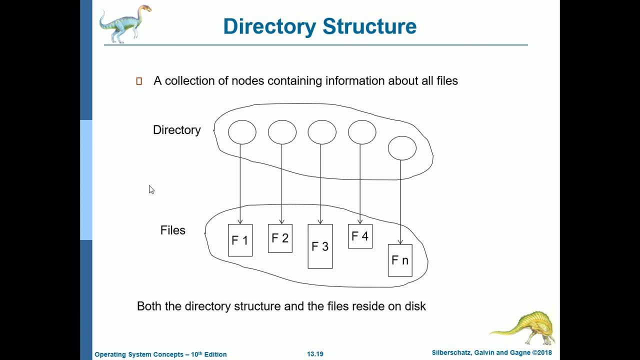 because relative file is larger than the index file, because index file is just a list. okay, next is we have the directory structure, so a collection of nodes containing information about all files. so this is an illustration of how this directory looks like as a simple as this one. so 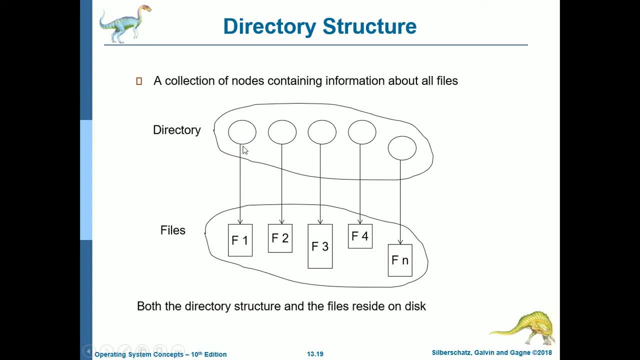 we have directories, so more like folders, and then for every directory there are files inside. so both the directory structure and the files reside on this. of course, if you're going to create a directory, the directory should have a content. so it's not, it doesn't look good because, of course, 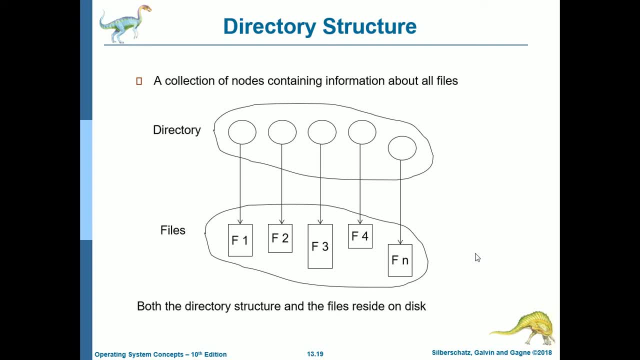 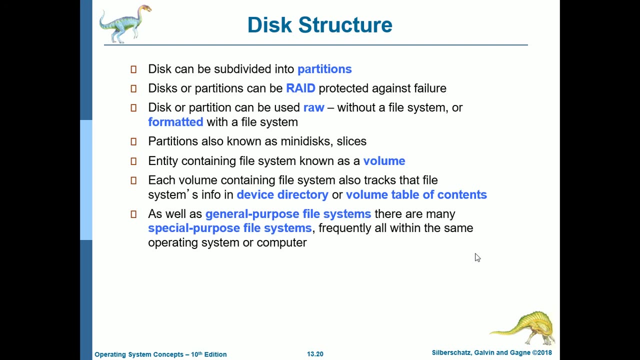 you're going to create a directory, then there's no content. it's empty. for me, if it is a user created directory, it's better for you to delete it, because what's the use of creating a directory for that if going to put a file inside? so next is we have the disk structure, so this can be subdivided into. 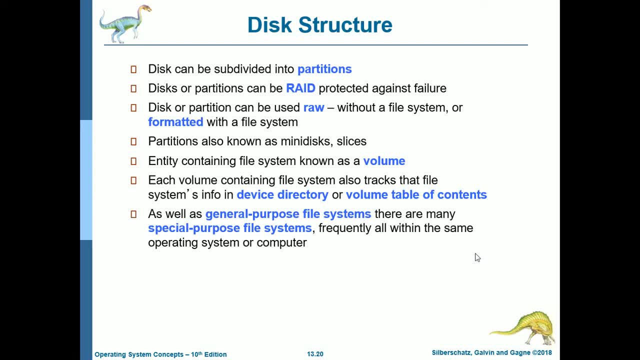 partitions. so if you're going to format your hard drive automatically, it will subdivide your disk into partitions. but of course it depends upon if you want to use the whole disk as a one- it's like a one whole volume or drive- or if you want to put it like, for example, partition in a. 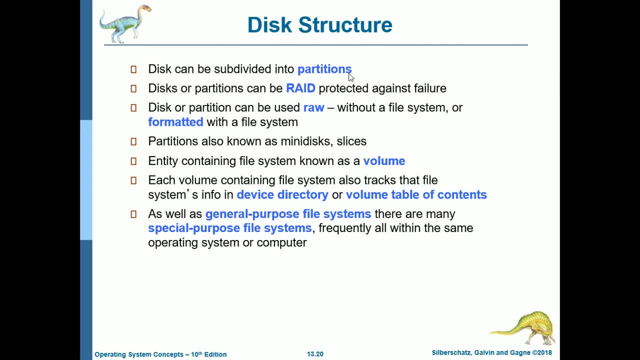 in a it's like a house: you want to partition your living room, your bedroom, your kitchen. so that is like the idea here, with partitions, so disks or partitions can be RAID, protected against failure. so we already have a lesson of RAID or redundant array of independent or 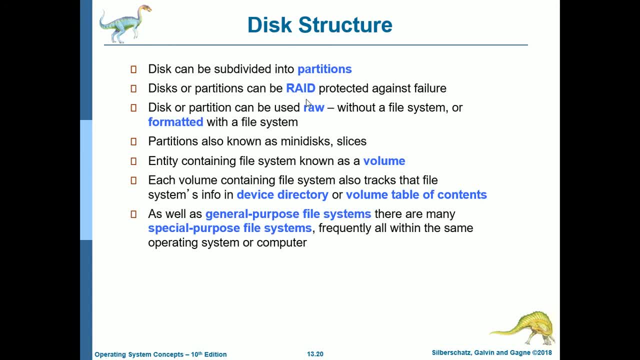 inexpensive disks. and then this disk or partition can be used raw, so raw without a file system or formatted with a file system, so most basically for windows. so it is requirement to format the partition for it to be usable, and then partitions, also known as mini disks or slices, and an entity containing file system known. 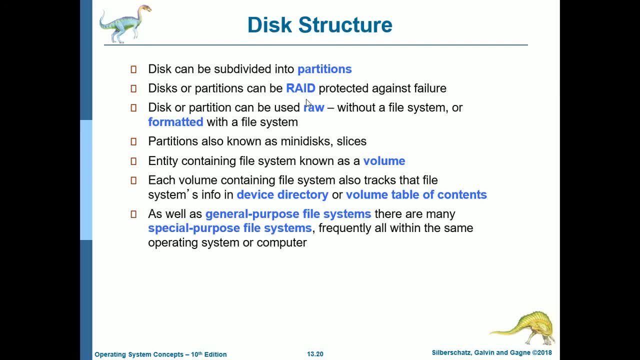 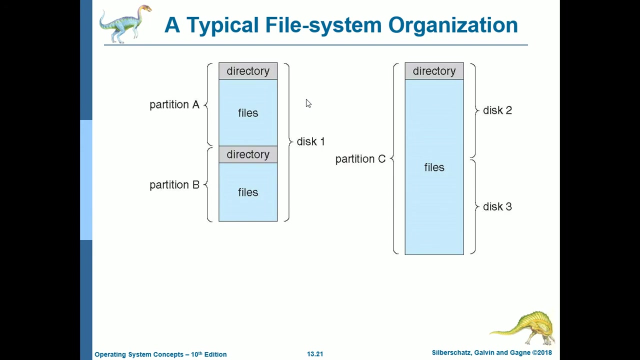 as a volume. so each volume containing file system also tracks that file systems: information in device, directory or volume table of contents. as well as general purpose file systems, there are many special purpose file systems, frequently all within the same operating system or computer. okay, a typical file system organization. so the typical in windows is we have this whole disks. 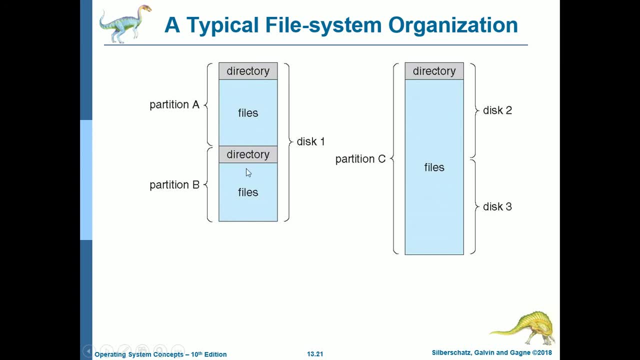 and then you want to divide your disk into two partitions. so that is the common set of partitions that we usually needelen, 등 al questo to be able to set up in a windows system. but there are others, um that, for example. so this whole partition is uh, it, it, uh, it needs two disks. so i'm really actually. 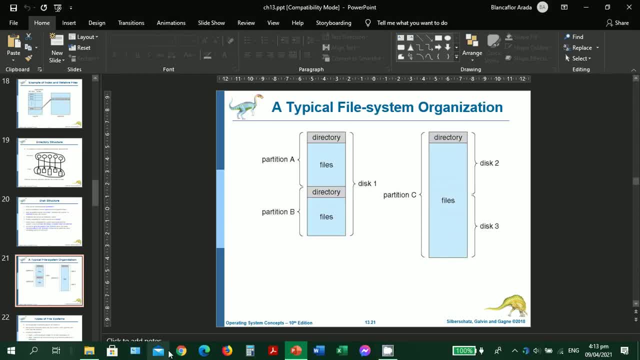 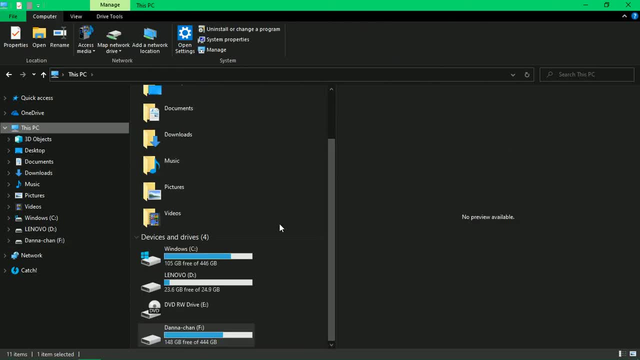 very not familiar with this one. i'm more familiar with this setup, so why so again, let's go back with our, with my file. so let's go to this, this PC, and then you, if you go to this, you can see theoudix atori. as you can see, i have, except for the dvd, uh drive, of course it's a different drive. 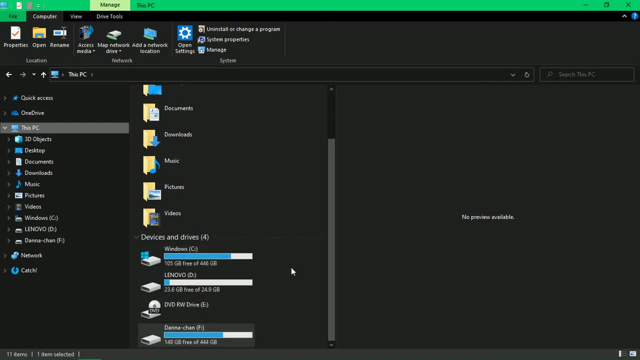 so you can see here as three drives actually um when computer was first, of course um the old computers. um partition is not possible at that time. so if you're going to see your drive with old computers, you can only see one drive. so so for that time, for old computers, if you're, if you see, 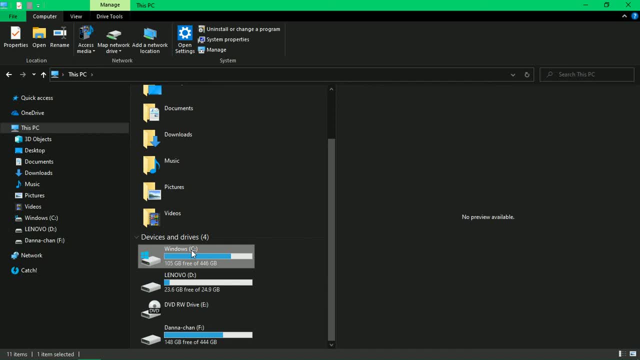 one drive means you have, if you see one uh drive c here, meaning you really have uh one drive in your computer system, a physical hard drive. but now because of partition. so what if your old computer has two drives? so it means that it's not a partition. it really does mean that your computer 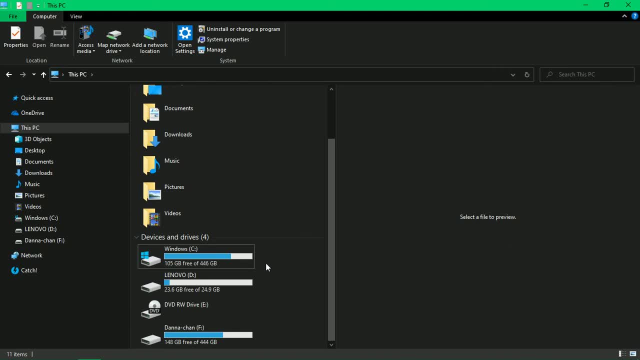 system has two physical hard drives but because of partitions, um, as users we can see that we can um, um have as many drives as you want because of the partitioning of, uh, of the, of the whole drive. so for this one we have three drives here, so we have four windows and then this is a 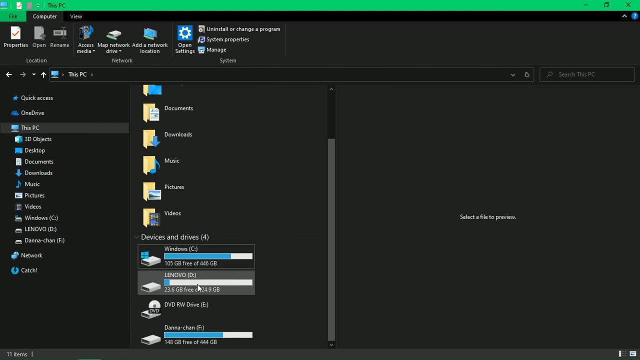 system partition. actually, um, actually it's your choice. actually, the content of this one is for the backup of the drivers of this um laptop, of course the brand, but but of course, as i've i've told you, you can actually um remove this partition and re and this 25 gig. 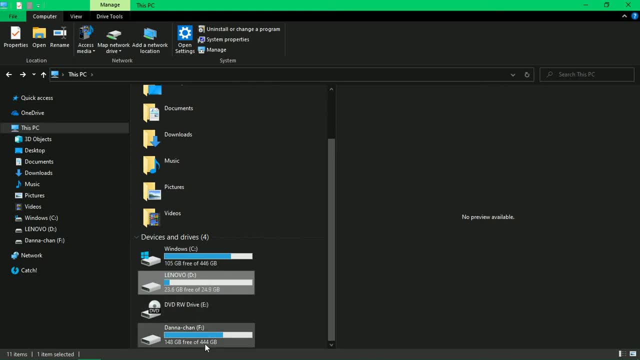 can be um can be added to the other partition, so this partition, so what i've been doing. so it's always like this. so we have a different partition for where the windows or the operating system is installed, and then this partition is used for data. so the 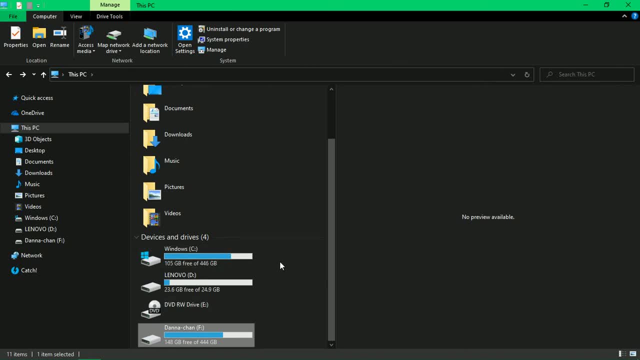 advantage of this one is: um, if your, if your hard drive does not have any partition and you only stored your, your files, your documents, in documents, in pictures and videos, and your, your windows, for example, got corrupted or it has an error or it has crashed, or just say that um the 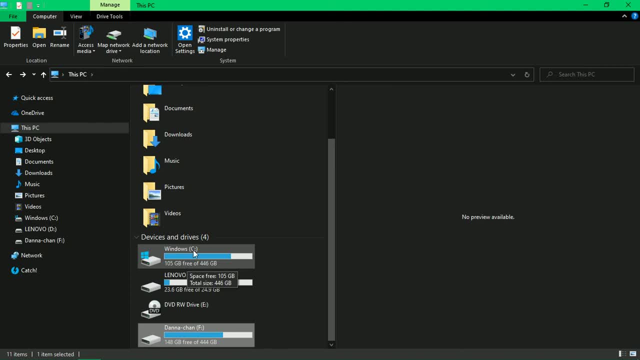 the windows installation becomes unusable, so as your documents. so that's why, um, if i go, i always do it. for example, if there is only one partition for windows, i always um divide it into two: the partition, so that the the other half will be used for data and, of course, all the applications. 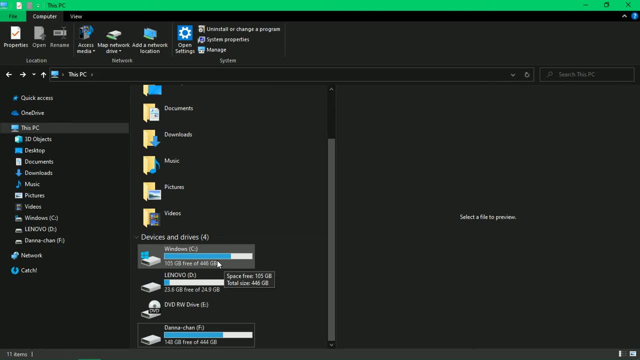 are in uh, in the windows uh drive, where in the drive where windows is installed, which is in drive c, but this one. so why did i remove this partition and include it in my um drive for data? it's just to small, so maybe i can deal with it. so it's just for failsafe operation, so that, if ever, of course, um. 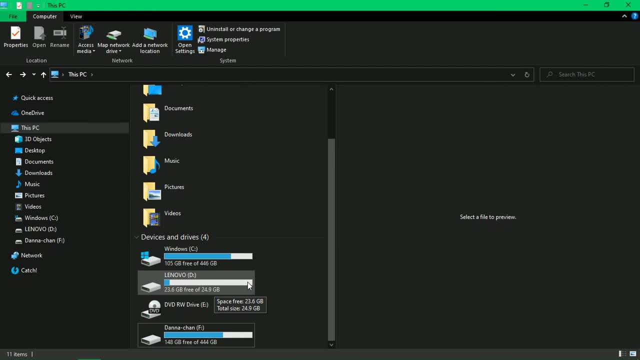 the the laptops nowadays does not have an installation of windows anymore, as with old computers, so the only thing that you can do to revive your old operating system or if if the installation becomes unusable or corrupted, is you have to back up your windows installation by using the backup and 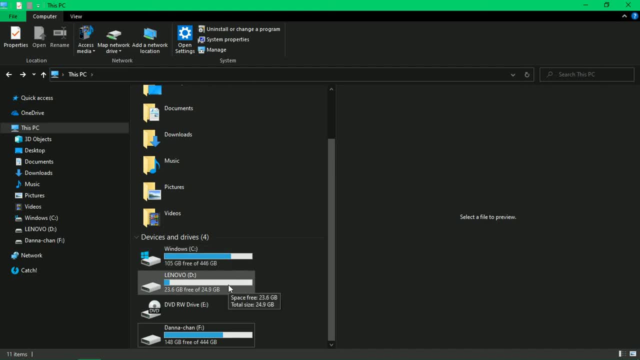 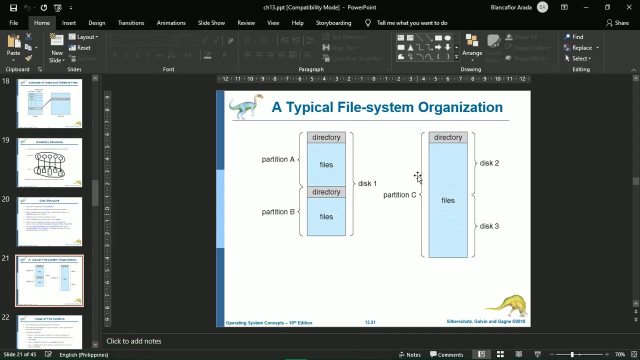 and of course reinstall all of the device drivers for this computer system. so again, um, you can see here three partitions, three drives, but it does not necessarily mean here that it has three physical drives. no, it only has one, uh, this drive, but with three partitions. so this is the uh setup here. so 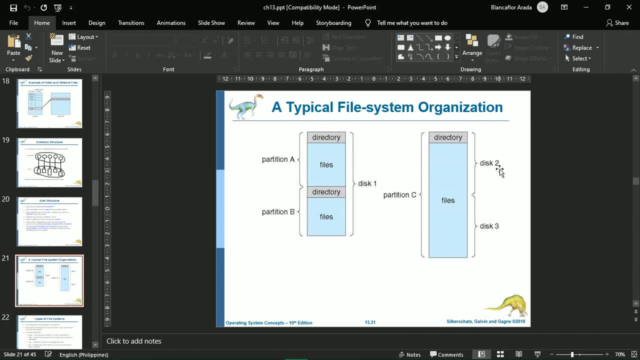 for this one um i. i don't know what to do with this one um. i don't know what to do with this one um i. i don't know how is it possible for two disk and then there's only one um directory of or file system for that. okay, so let's return again with our 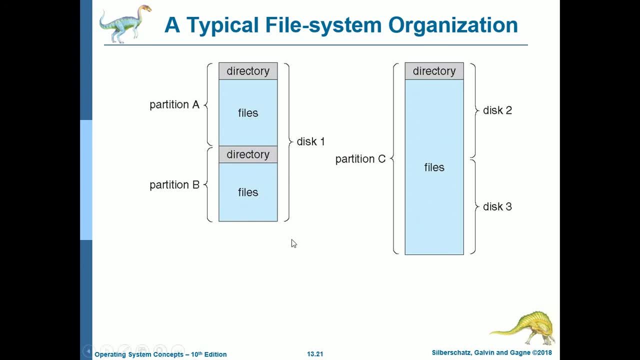 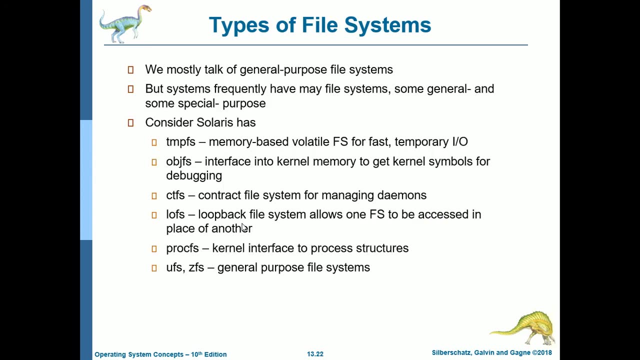 presentation. so again this: this first is the most commonly used for typical file system organization. okay, next is we have types of file systems. so we mostly talk of general purpose file systems. but systems frequently have many file systems. some are general and some are special purpose. so consider solaris has- so it has a tmpfs. 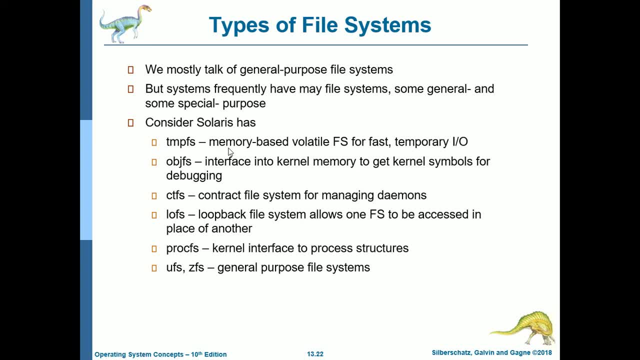 this is memory based volatile file system for fast, temporary i also. that's called tmpfs. we also have objfs interface into kernel memory to get kernel symbols for debugging. and then we have contract file system for managing daemons, so lofs. so look back. file system allows one fs to. 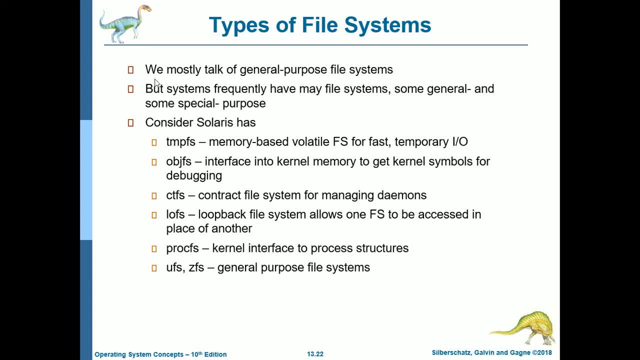 be accessed in place of another. and then we also have another, the proc fs kernel interface to process structures, and we have the ufs zfs general purpose file system for solaris. it uses different file systems depending on the operations of or the the applications. so that's an example for. 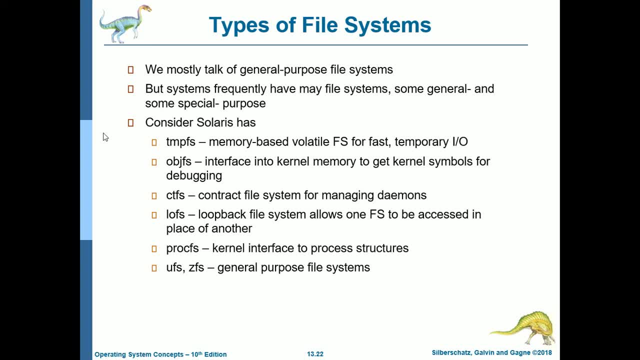 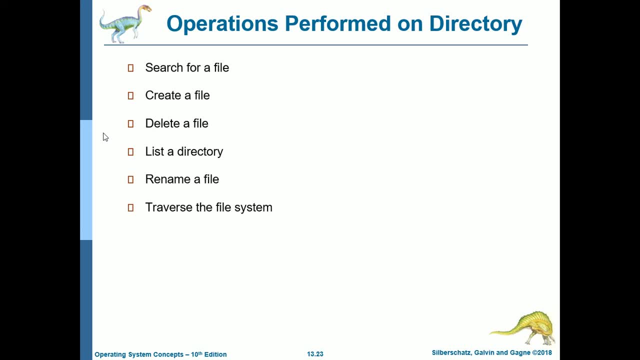 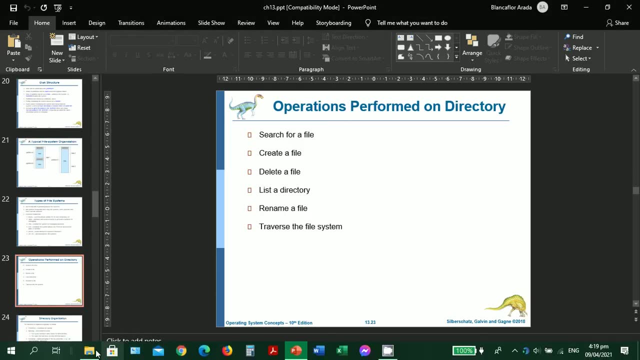 solaris, so we're not really very familiar, of course, because we are more familiar with other operating systems such as windows. okay, next is operations performed on directory, so you can search for a file. so again, so how to search for a file, so it's convenient for windows. 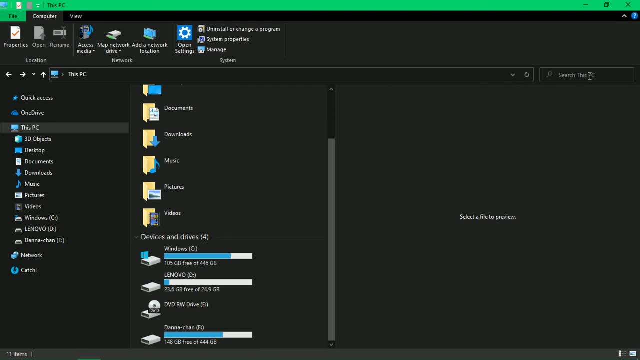 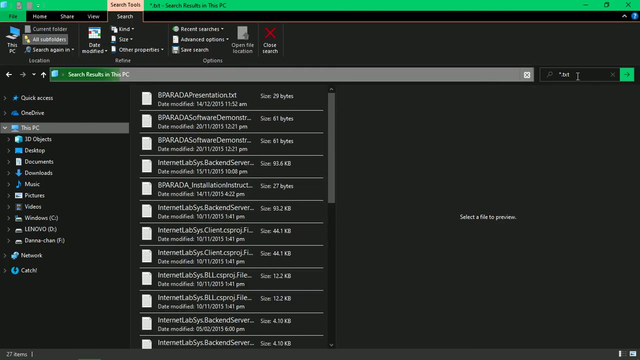 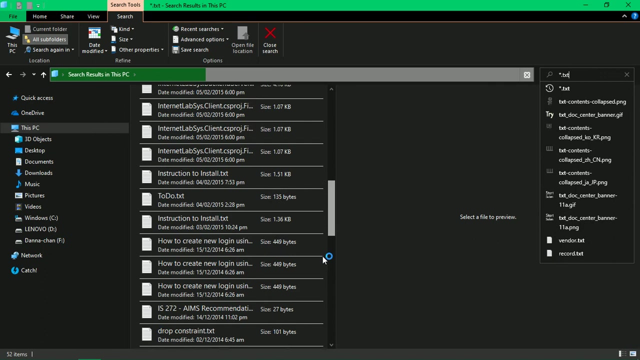 because they already have this search box so you can search anything here. just type anything. so if you're going to search for any text file, you can have. this is a windows rather dos. this asterisk means disregarding of the file name. okay, disregarding of the file name. you're looking for um file type, dot txt, so that you can see here. 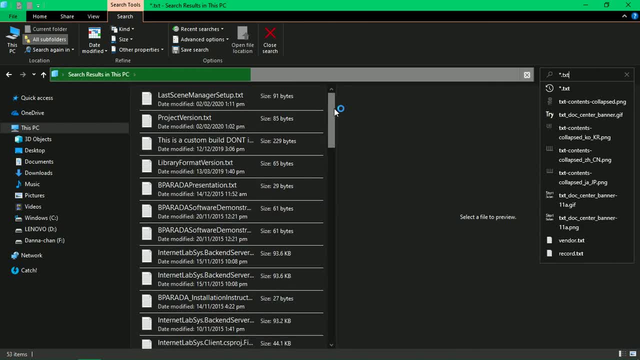 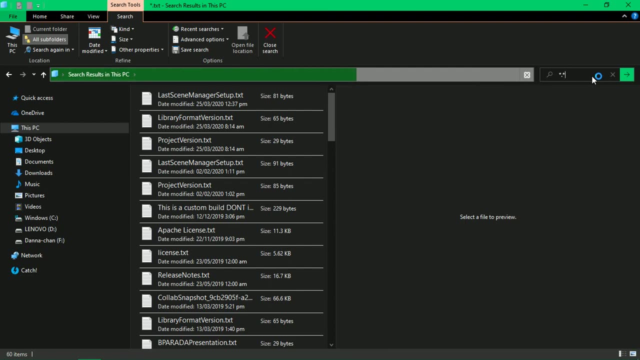 that it really is looking for any file types. that is dot txt, disregarding its um file name. so what, if you're going to use asterisk, dot asterisk? it just means that if that's asterisk, dot asterisk, you're going to search for all files. so you're going to search for all files, so you're going to. 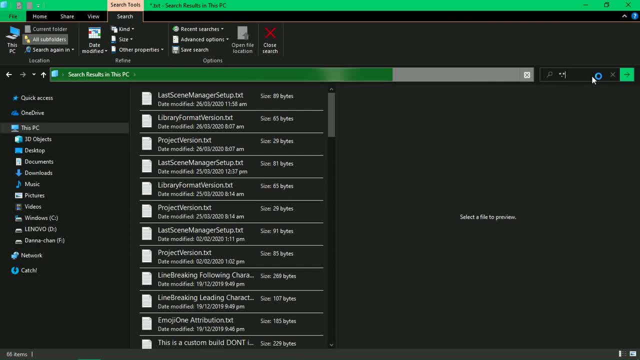 actually it's very, um, cumbersome. you're searching for all files, so um. this, of course, will be more usable if you knew the file name and, of course, the file type. i just illustrated to you the usage of asterisk, asterisk, disregarding of the file name. and then, if you put asterisk dot, asterisk, this: 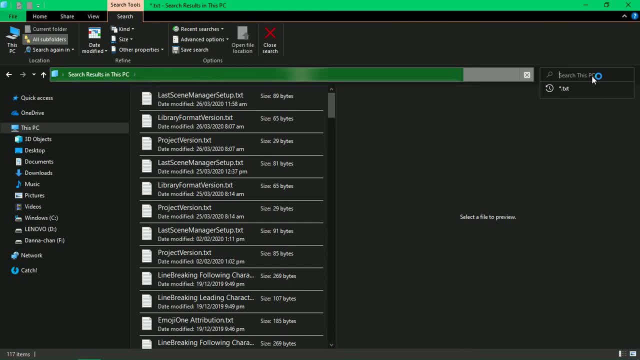 you're searching for files, disregarding of the file name and file type. so it means it will search for all documents with all the files. so you can search for all the files. so you can search for all uh file types. that is inside your computer system. so let's just um stop it uh the search. 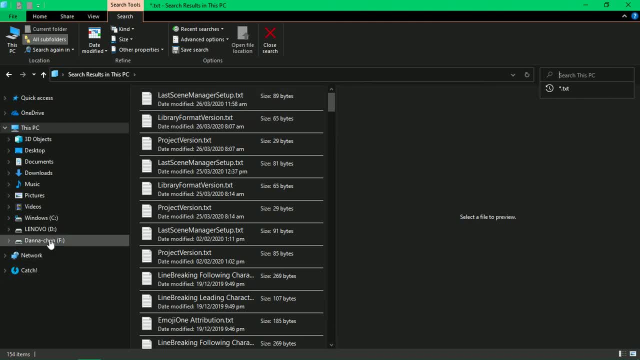 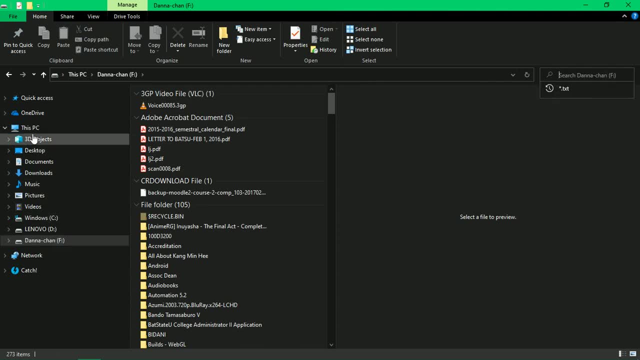 but if you want it to be more specific, you can go to a specific folder. so that's why, of course, you can only search for that drive, because here, of course, the, the, the smaller, the it's like searching for a room. so if you really know where to search your files in that particular folder, it's better. 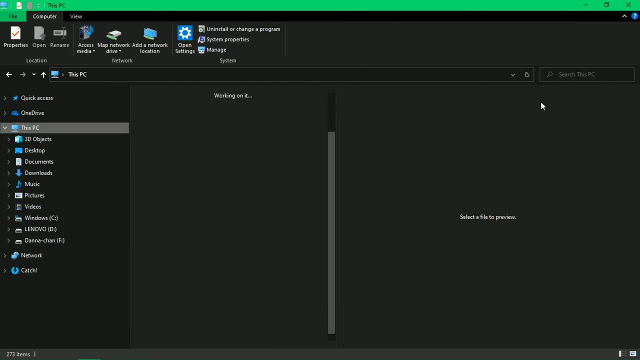 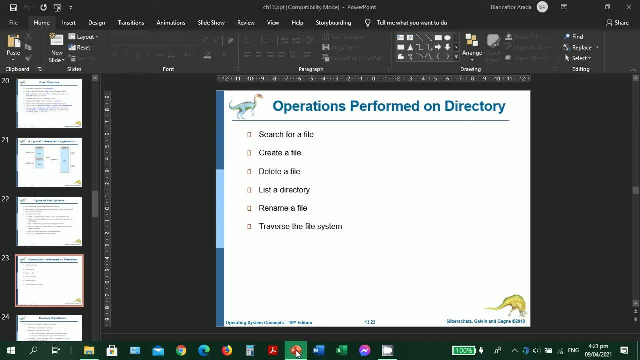 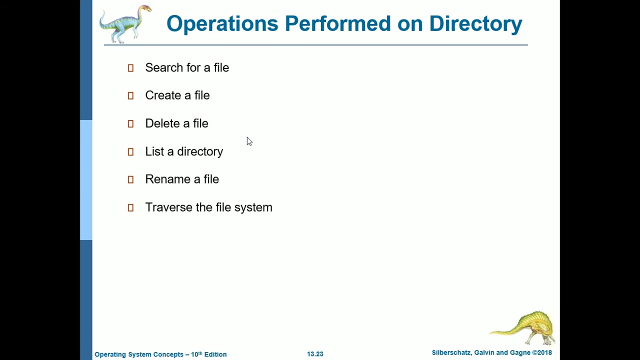 than to search, for example, with this one in this pc, because it will search for uh, drive c, drive d and drive f. okay, so you can also- of course you've already has an- have an experience for creating a file. of course, user created files such as word documents, slideshow, presentation, excel file or any. 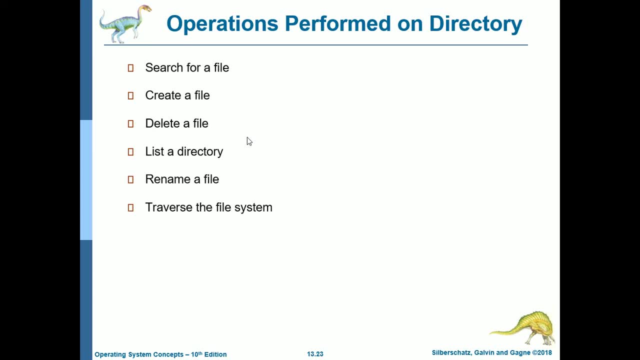 other files that you are required to do, and then you know how to delete a file. okay, it's just right click or uh, then delete, or just click on the file and then press the delete button on the keyboard and then, of course, list a directory. i've already shown you in our previous lessons by using the command prompt. 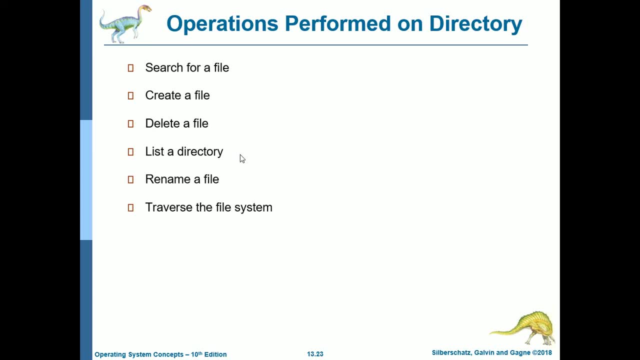 how to list directory in the prompt: dir, slash w, okay, slash p or so that's an example- and then to rename a file. so you can, as you can remember, you can rename a file and then you can rename a file in the properties, as i've in the previous slides, because you can change it there or you can right. 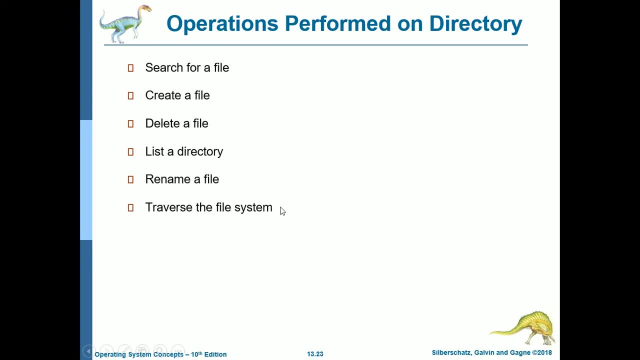 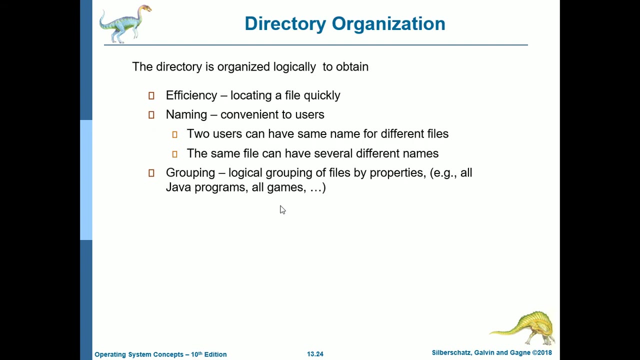 click and then rename a file, and then of course you can also traverse the file system. you are already doing the traversing the file system if you're searching for that particular file. okay. next is we have directory organization. so the directory is organized logically to obtain first is the efficient. 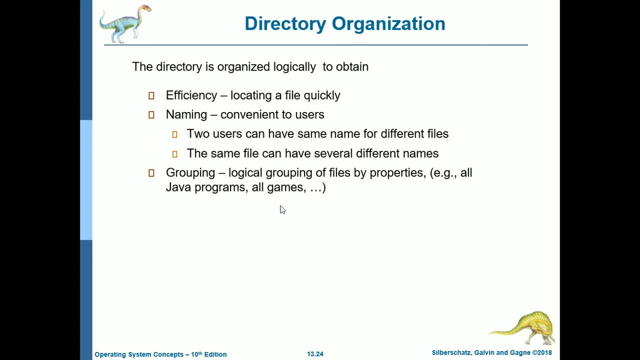 see locating a file quickly and then also the naming convenient to users. so two users can have the same name for different files- it is true as long as they are in different location, and then the same file can have several different names, because if you want six copies and you want to, 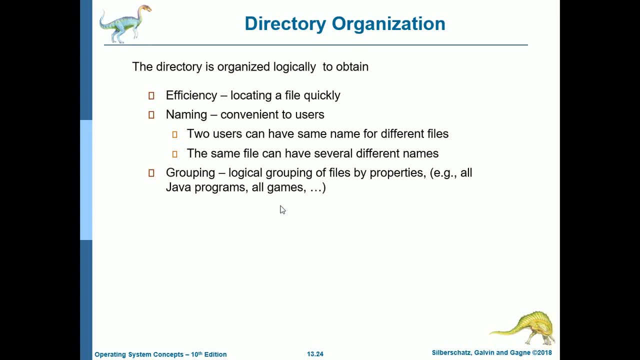 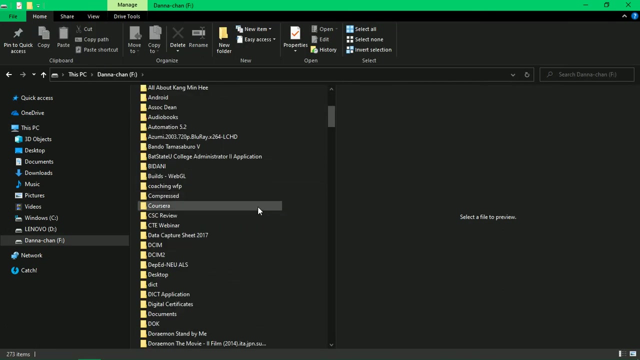 put version one, version two, version three, version n, so that same file can have several different names. and then we also have grouping, so logical grouping of files by property, such as all java programs or all games. so actually in my example we have this grouping. okay, uh, let's go with our folder, so okay, so again with our. as you can see, 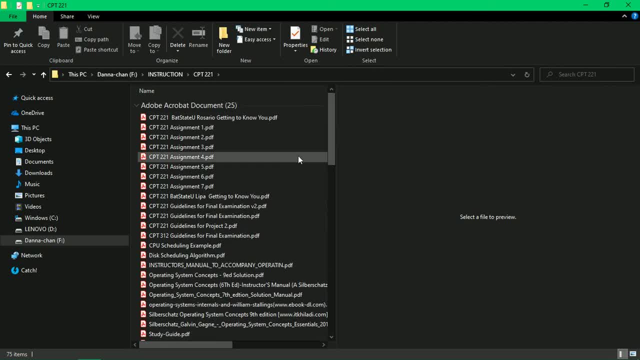 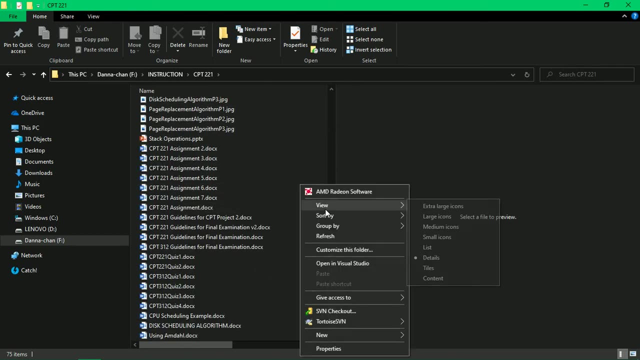 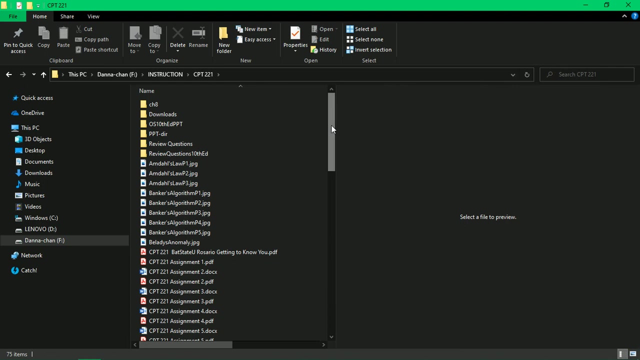 this is already grouped: um. for me, it's better to search by um. we have this one. you can view it as, for example: um, none- okay, if it is none, and then view by example, by name: okay, um. for me, um. i don't know if. if it works for you, maybe it. 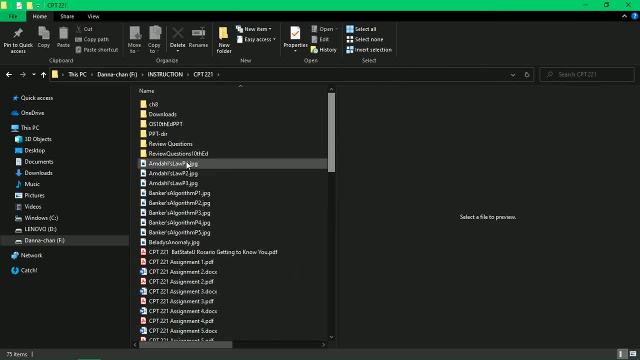 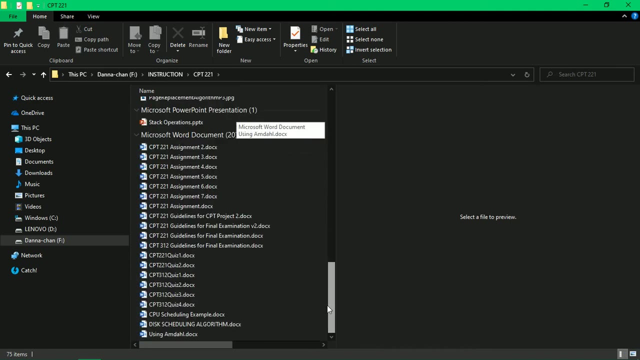 depends upon the person. um, of course this is in alphabetical order, but for me it's very difficult that it is arranged in in this fashion, so i always do is: uh, you can group by type. for me it's easier because if i already knew the file type? 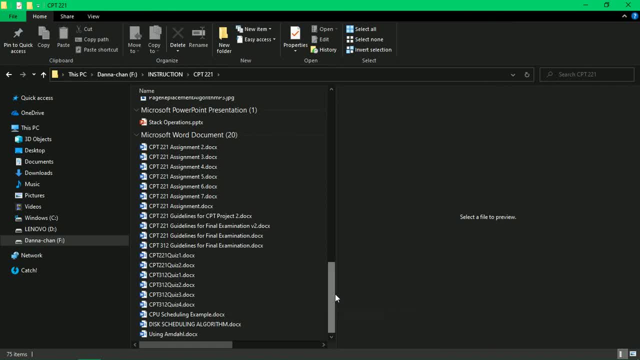 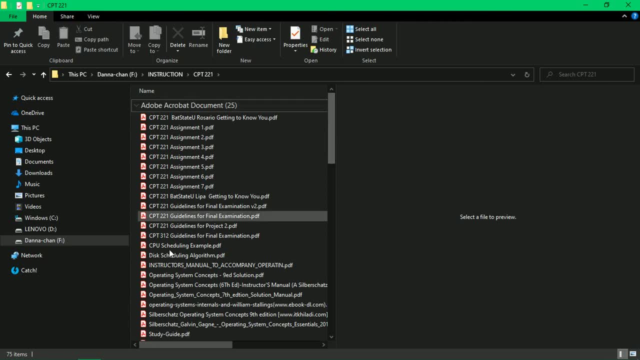 i'm just going to go for example. oh, i know it's a pdf file, so i'll just need to search for this and it's already arranged. uh, these are all grouped for pdf files, so it is uh. click anywhere, then group by type. you can do it. date by: 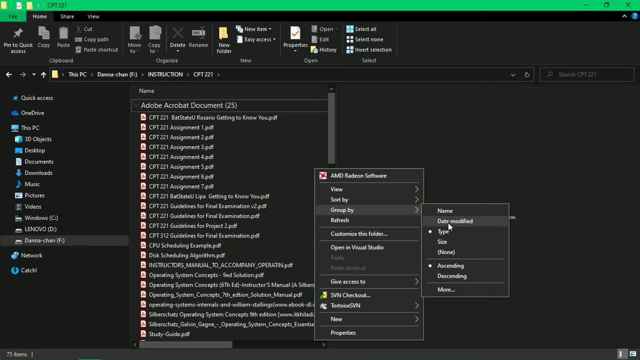 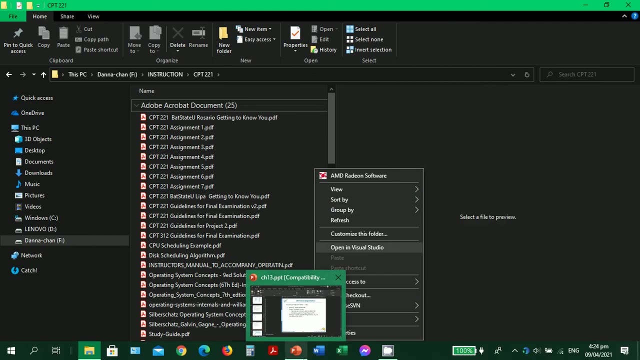 date modified, if you want to, especially specifically if you can remember that you've modified this, uh, this file on this date. so it depends upon your preference, but for me it really works. for me is the grouping of the same file type, so you can change it the way you want, if 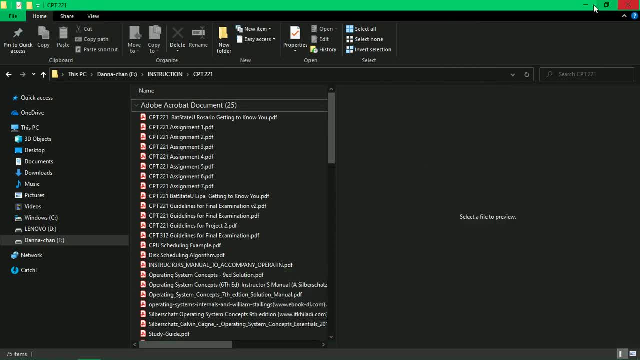 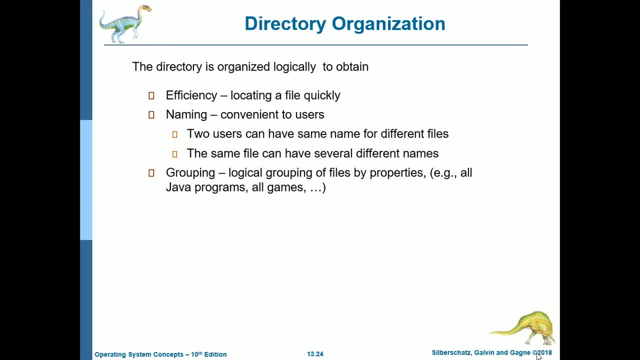 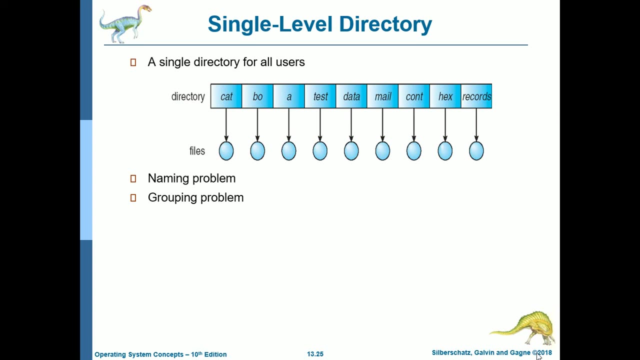 you have your own computer system. so again, let's go back with our presentation, okay, okay. so for the structure, there is a single level directory, so a single directory for all users. so we have an example. we have one, two, three, four, five, six, seven, eight, nine. example: here is we. 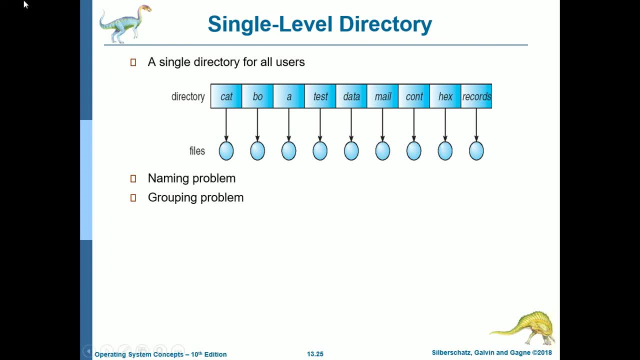 have nine directories or folders and they have their own files. so since this is a single level directory, so one folder and then file. so we we can encounter, for single level directory we have the naming problem, because why so? files must have unique names, of course. and then the grouping. 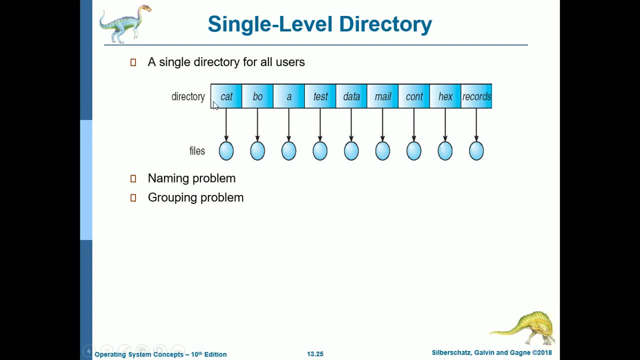 problem. you can't create folders for this example. you, for example, you have files and you want to group it to, to to this type of file, or it depends upon your preferences of whether what is the name or what is the category of that of that file. so you can't create another folder inside the directory. 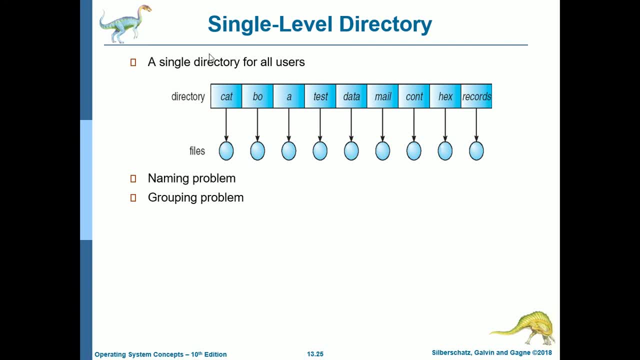 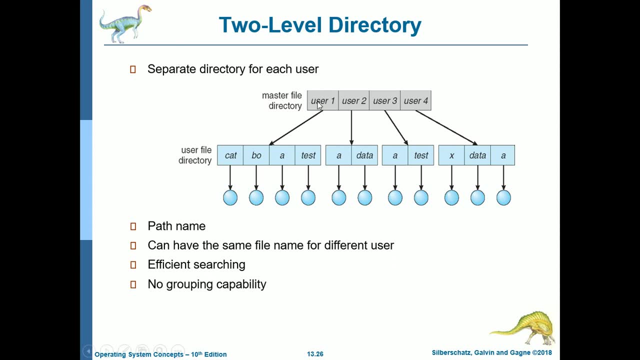 because it's a single level directory. okay, next is we have a two level directory. so we have a master file directory, so it's named after the users, and then they have their own set of directories and we have the files. so, by means of two level directory, there is already a path name and it is also. 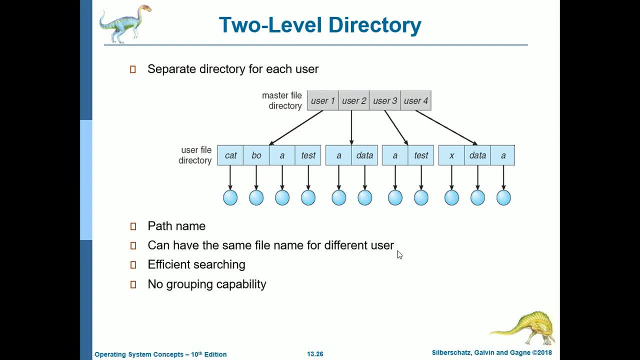 possible that it can have the same file name for different users, of course, because it's a different document for this example. so the same kinship, as if there is something that nothing Somehow beat our king because CSS had a function in the last row: Нап Cooper, natomiast It sell. 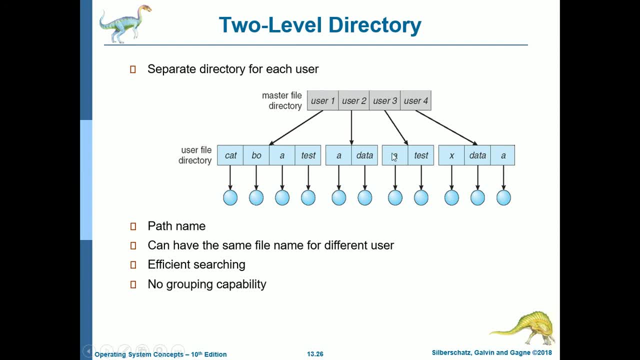 for example, user 1 has a directory also with user two, with user 3 and user four, and this, this directory, does not mean for them that they have the same contents. no, it depends upon the user's preference of what files he or she can put in that a directory or folder. 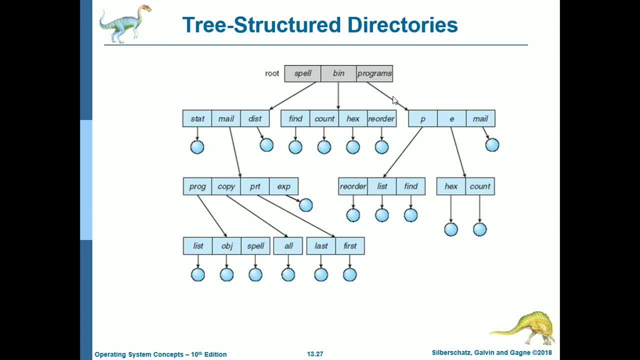 capability. okay. next is we have the three structured directories. actually this is the modern day structure of directories, specifically in windows. so for example, this one, this is the root directory. you can have as many nested directories or folders inside. so, for example, this spell root directory. and then we have mail and then mail has prt and it has another directory. 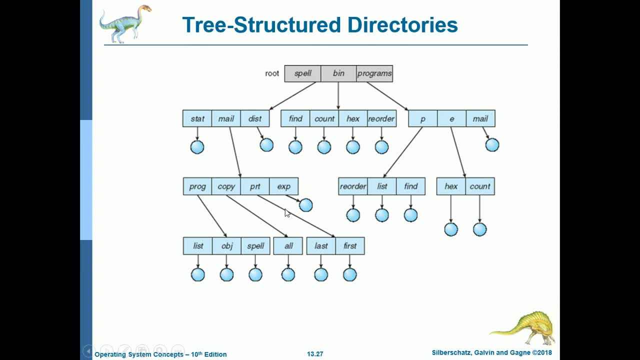 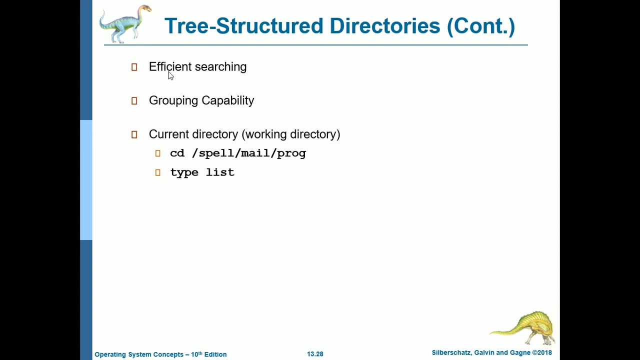 for first and then the file, but also it can be a combination. aside that there is a folder, there is also a file. so that is the three structured directory. so for three structured directories, of course we have efficient searching and we already have the grouping capability. okay, so current directory or working directory, so cd, as you can remember, with the command prompt or 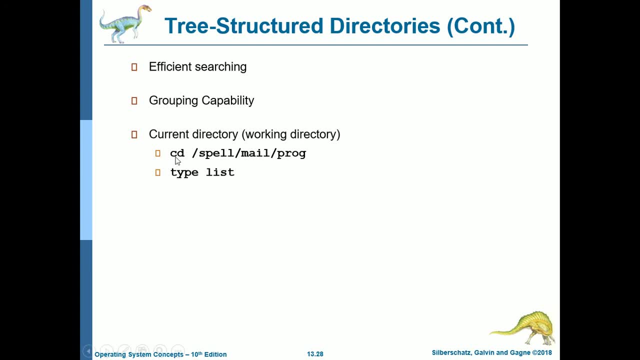 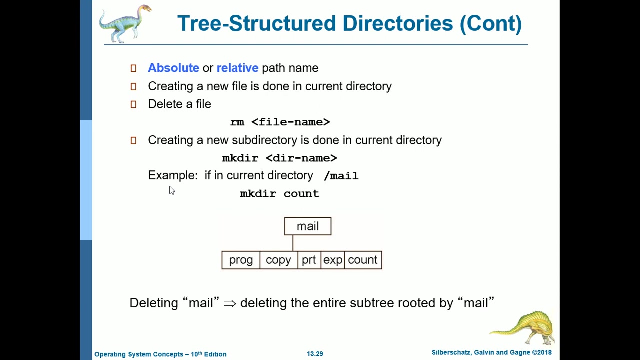 the window shell. so this is different, because cd here in linux is a current directory. for windows it means change directory. so this only means that it is in the current directory or we have another command for type list. okay, we have here. so for this three structure directories we have. 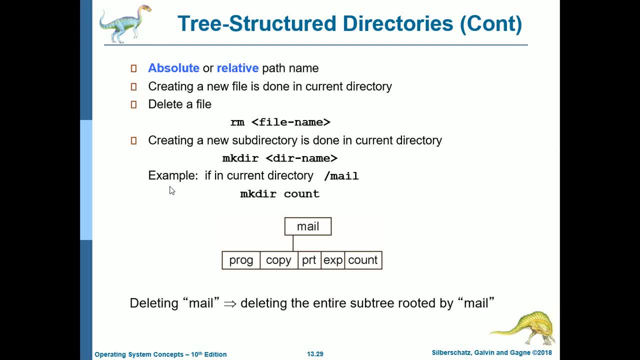 absolute or relative path name. for absolute meaning, its path name starts with the root directory, while the relative path name it is the current directory. so creating a file is done in current directory, of course. so even in our directories. that is for example we use. we are using windows, if you want. 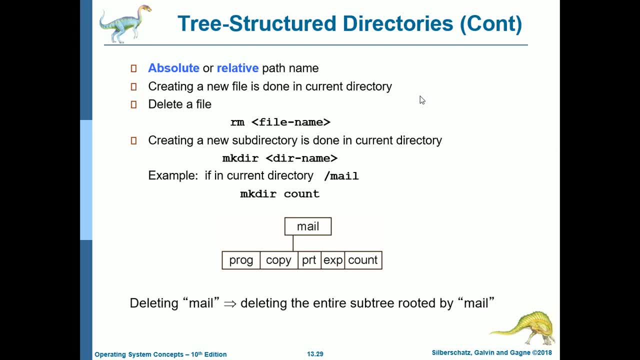 to create a file. it will be done in the current. it will always be done inside that directory or the folder. okay, how to delete a file? so we have rm. so this is linux. this is very different with command shell. so the command is rm and then file name, and then creating a subdirectory is done in. 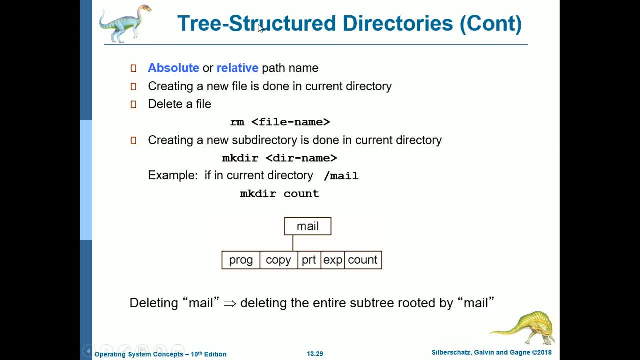 current directory, so mkdr. so this is creating a directory for windows. it's m md make directory. so if in current directory slash mail, mkdr, count so mail, and then it added new directory, count, then deleting mail, deleting the entire subtree rooted by mail. okay, let's create a. 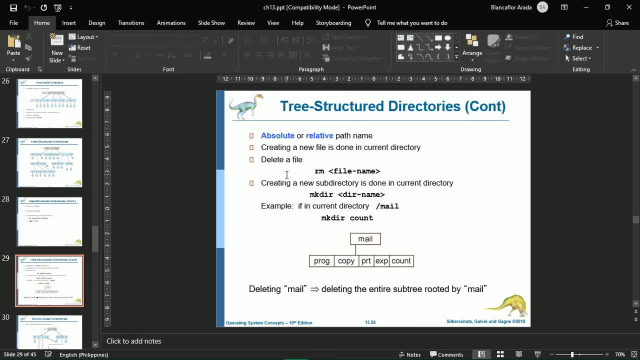 file and then we're going to create an example. so how are we going to create a file? so let's open again our file explorer for you just to illustrate, and then we're going to illustrate it in windows. so again, let's wait. again, i'm really very sorry for. 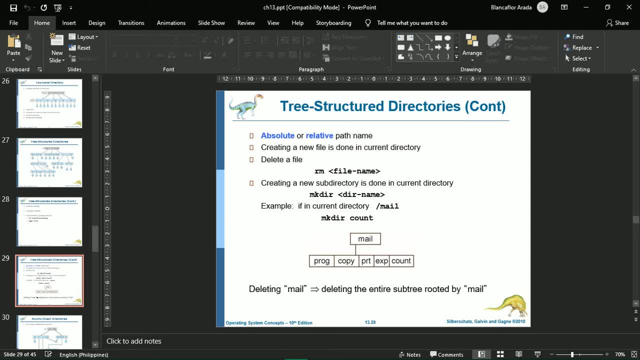 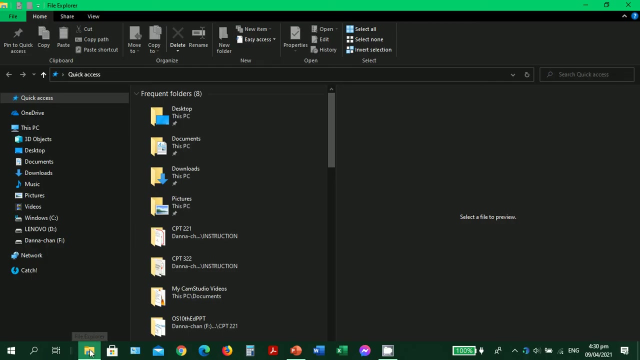 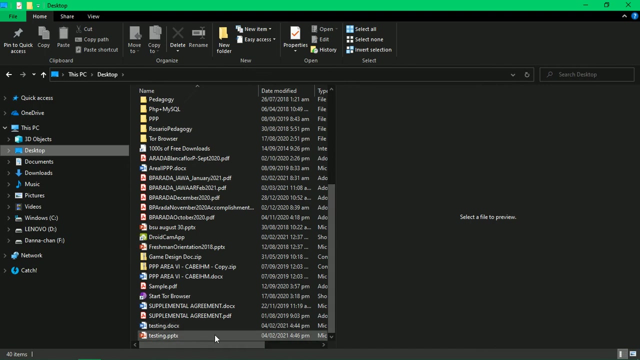 for the past response of my computer. okay, do you think i need to buy a new one? i think so, but uh, i still don't have money to buy, so i'm just going to stick with it for a little while. ah okay, thank you again. okay, let's go with the desktop and then let's create a file. okay, we have. 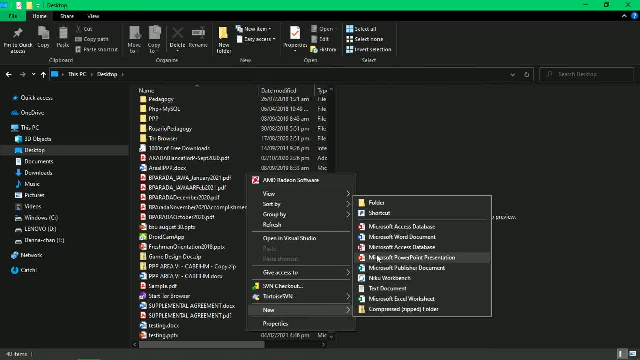 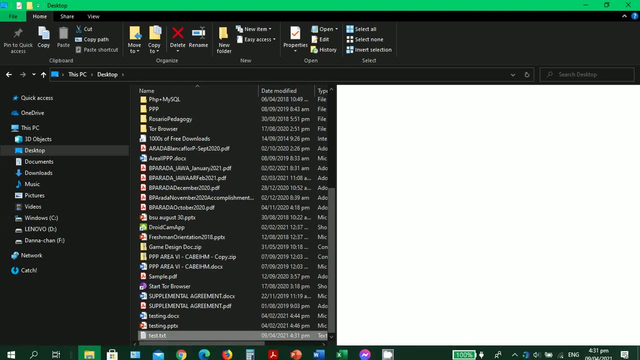 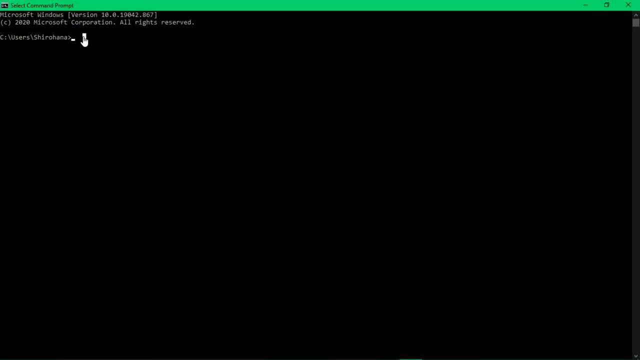 just a simple text file, so new, okay, text document. so again test dot, txt. and then let's open our command prompt. okay, so you just want to locate our um di to locate desktop, dir, slash, w, slash, p, again to list the directory. so of course desktop is here. so let's see the desktop. okay, let's again list the contents of. 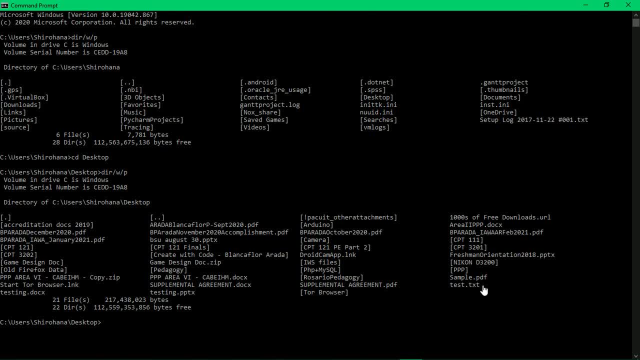 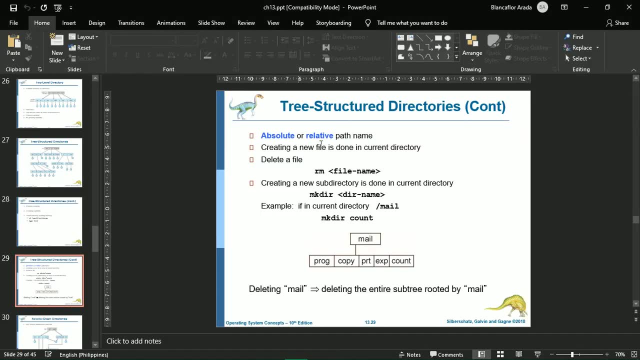 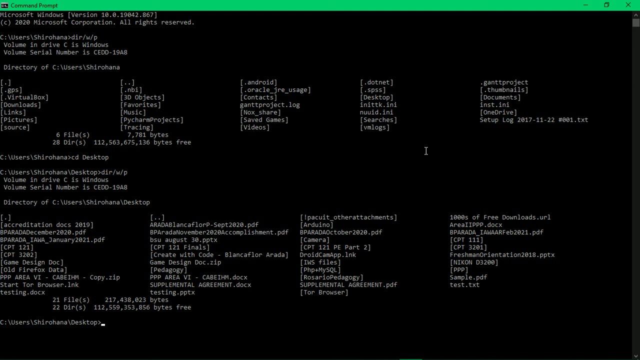 this directory. so, as you can see, it is already here the test dot txt. so what we want to do is what we've already created: a file. so of course, you can see that when i create a file, i'm going to create a file. it is really inside that folder or there or directory. you cannot create a file. 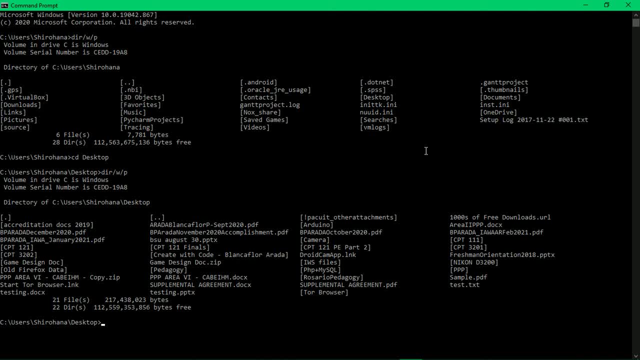 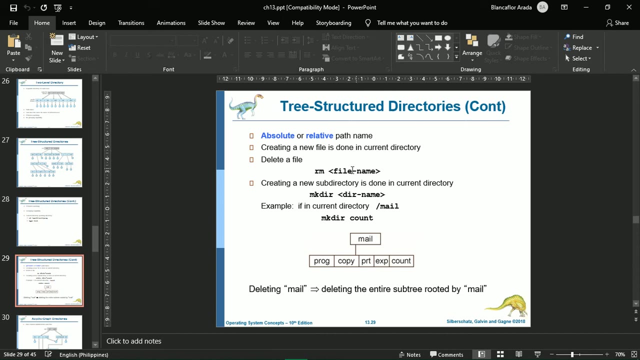 intended file if you're not in that directory. i think it's not. i don't know if it's really possible, but for me, in my opinion, it's not possible. you have to be in that directory to create that file. so if you want to delete a file for this command- for linux it's rm, but as you can, 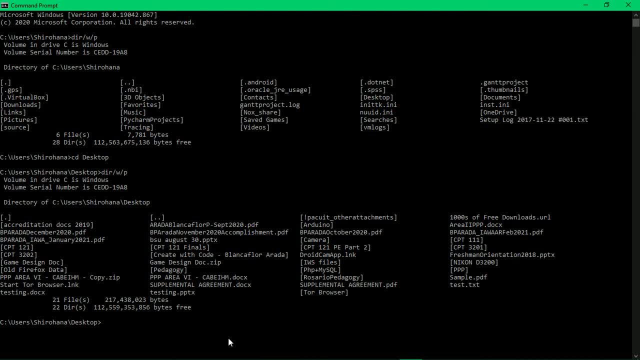 see, we have. okay, so we have a file and we have a directory, and we have a directory and we have a. we want to delete a testtxt. so the command here is del and then testtxt. okay, so it has no response, there's no error. so let's just see if, uh, the delete is successful. so again, dir slash w, slash p. 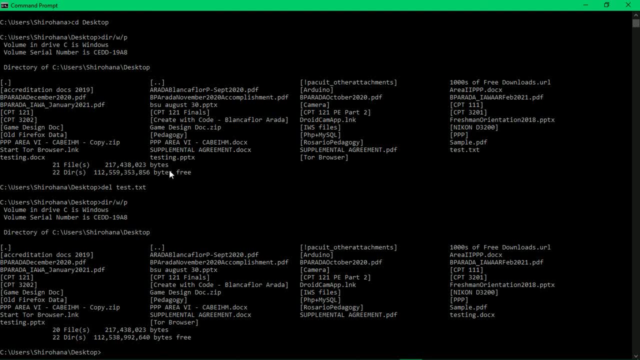 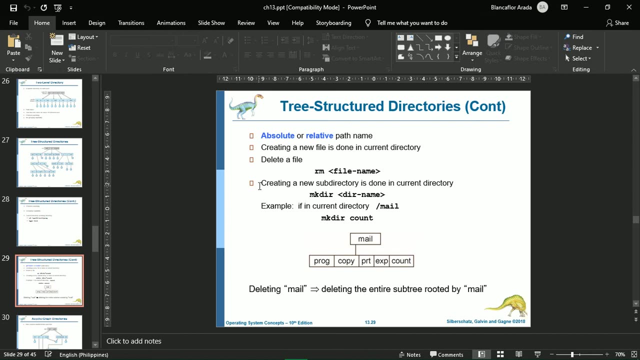 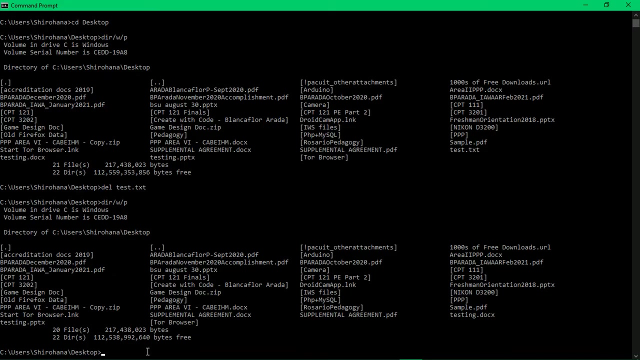 okay, there is no testtxt, so it means i've really deleted the file. so for windows the command is del. okay, then creating a sub, new subdirectory is done in the current directory, again of course. so what if i want to create a new directory? so let's just follow the example. for example, mail. 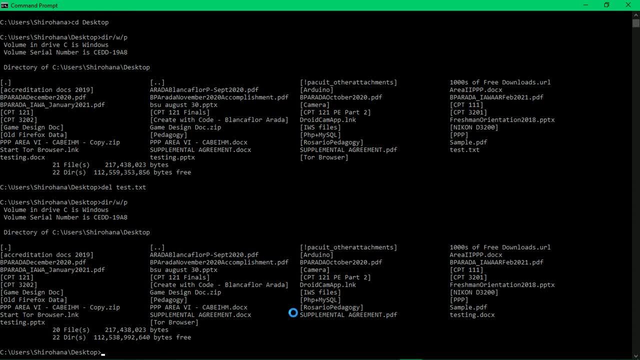 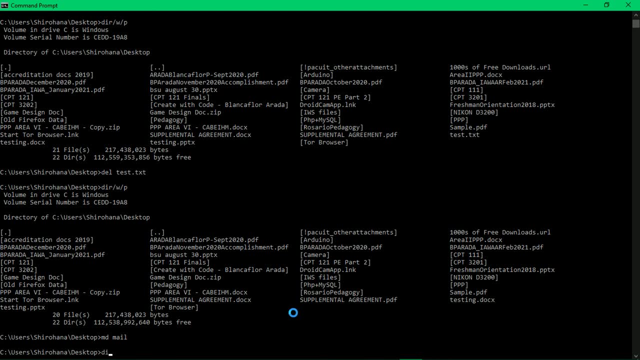 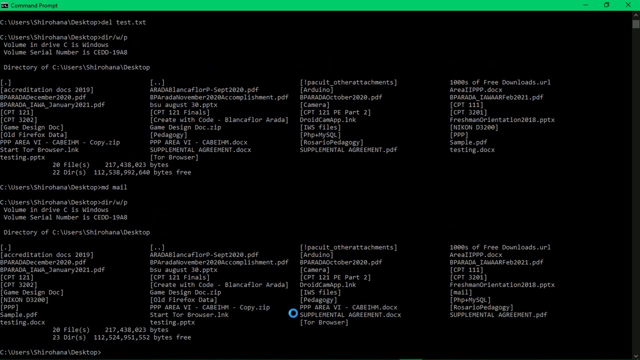 okay, so for creating a directory, we have md, then mail. okay, let's check dir. oh, let's just not type it. oh, dir, slash w, slash, p. just click the up arrow, because it lists your previous commands that you have typed. you don't need to type it anymore. okay, so we already have mail. and then it also wants to have a create a directory. 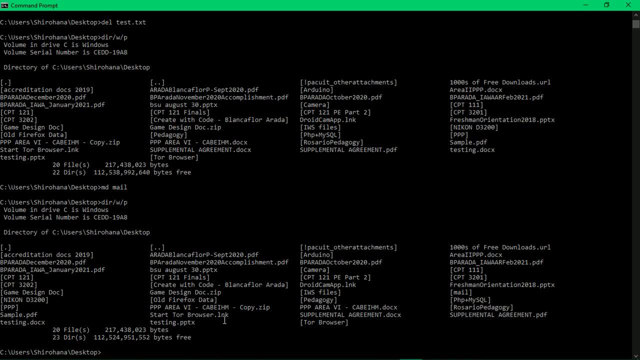 for, uh, the name is count, but of course if you want to create a directory you have to go inside. it's like clicking the folder and you'll be inside the folder for again. for this command prompt. uh, you want to go inside mail, so you have to cd, so again. so for linux, cd means current directory. 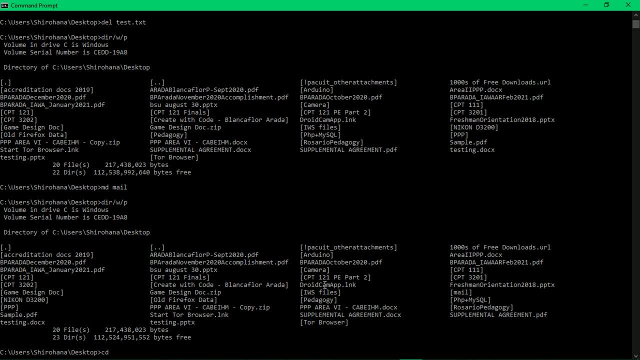 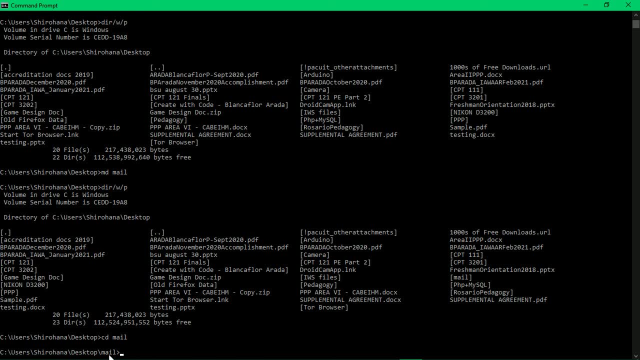 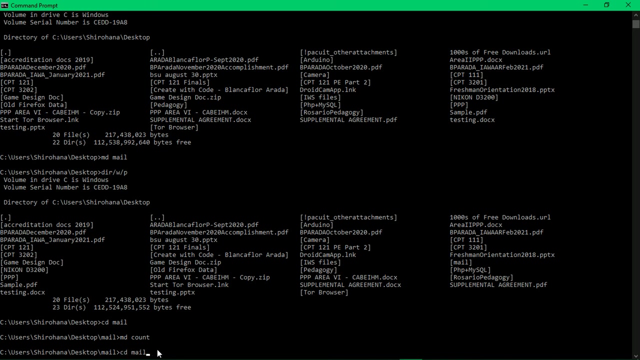 but for windows cd means change directory, then mail. so as you can see, with the prompt you're already inside um the folder mail, and then you want to create again another directory. so dir slash dub. okay, let's not type it anymore up arrow. okay, so you can see here that you already. 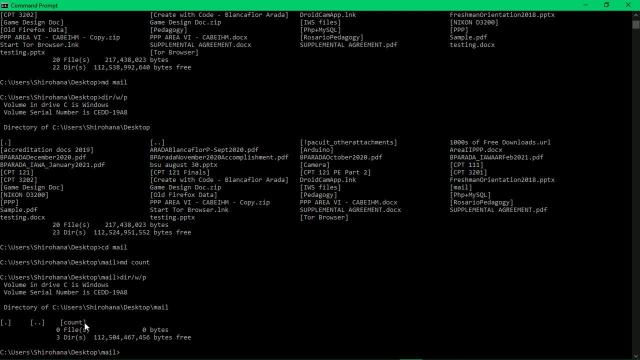 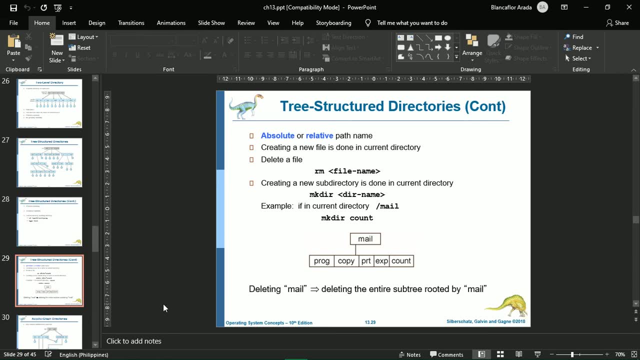 have the um folder count inside the um folder, mail, a nested folder. so can we delete mail or deleting the entire sub rerouted by mail. so for for um for linux, it's possible that if you're going to delete mail, you can delete the entire sub rerouted by mail. so for um for linux, it's possible that if you're going to delete mail, 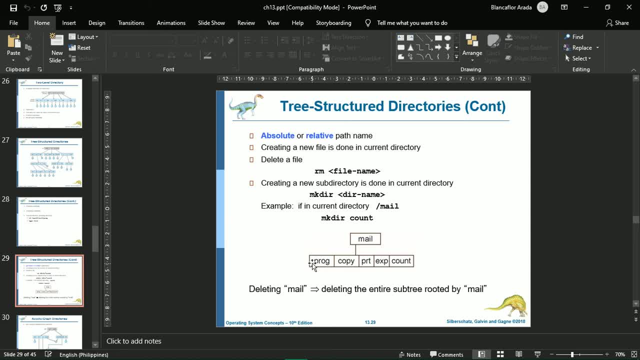 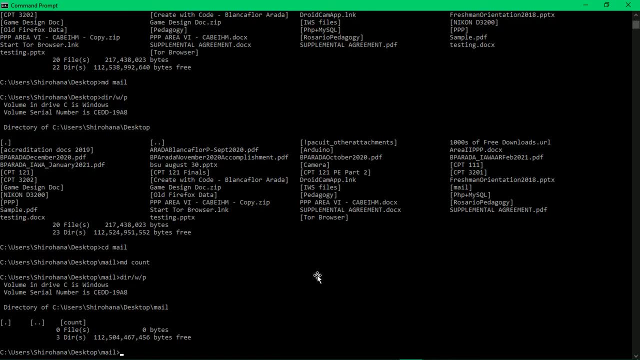 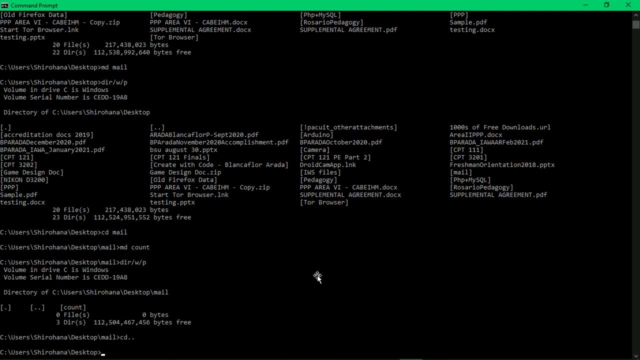 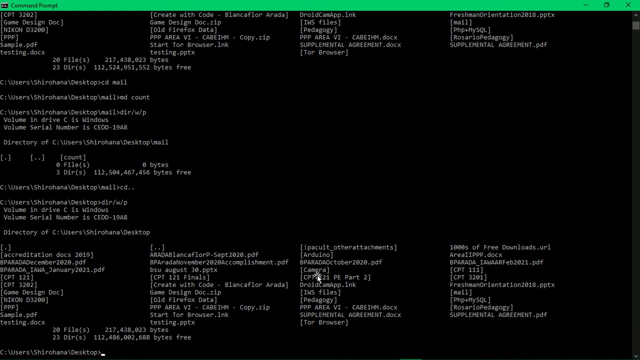 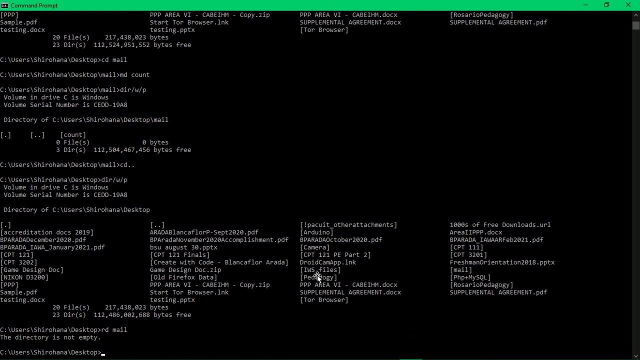 um, you can delete also its child directories or sub directories. so let's just go back with desktop. okay, cd point point, meaning you returned, you exited that current directory. then again, okay, let's delete. so deleting directory here is by means of rd rd mail. okay. so for windows, for command, actually in those. uh, this is really actually not. 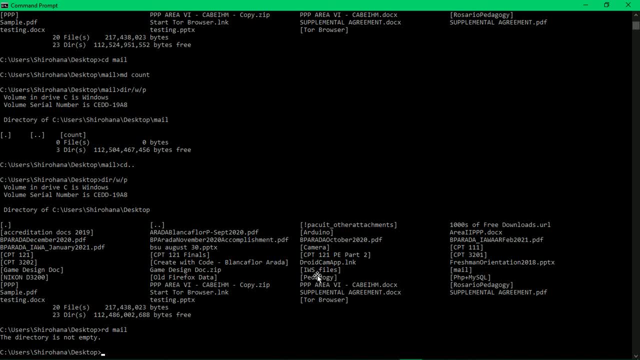 possible. if you're going to delete a directory here inside a command prompt or in dos, previously make sure that the directory is not empty. but of course, if you're going to use our file explorer in windows, just click the the folder, uh, disregarding if it has. 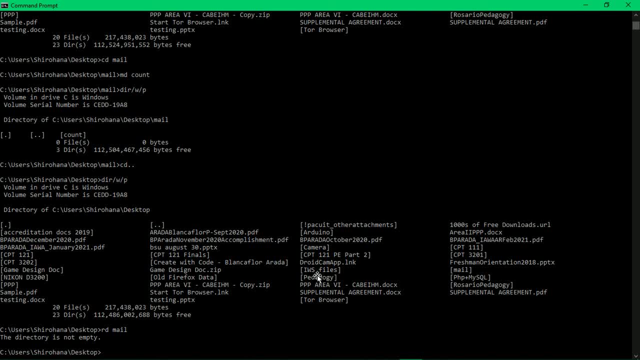 a contents or it has no contents, just right click and then delete it, and then you can delete the. it will be deleted, but for here, for for windowshell, command prompt, windowshell or previous, uh, the dos of disk operating systems, it will always require that for you to delete. 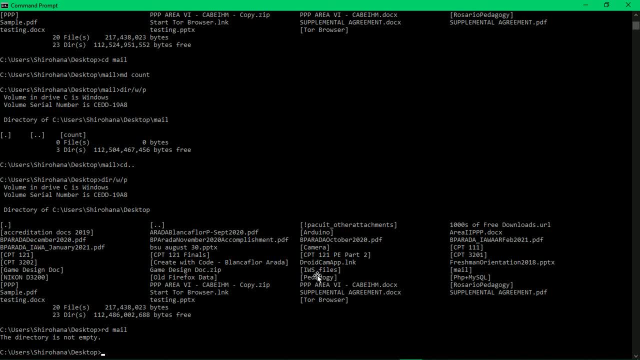 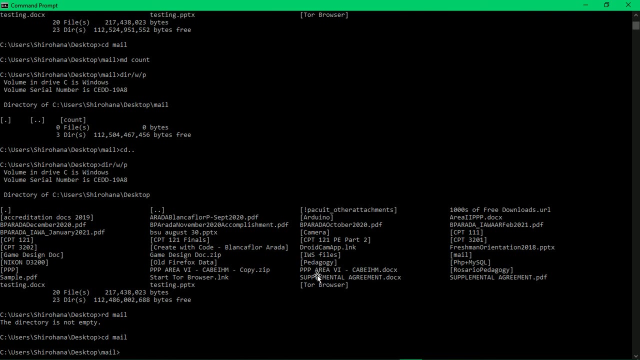 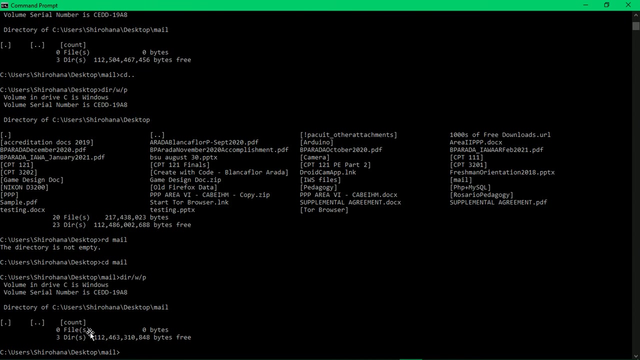 that particular folder or directory is. make sure that it is empty. so you can't delete mail directory, so again you have to go inside, okay, inside mail, okay, and then, since count here, as you can remember, okay, you can remember, it does not have any, uh, contents. okay, just to make sure. 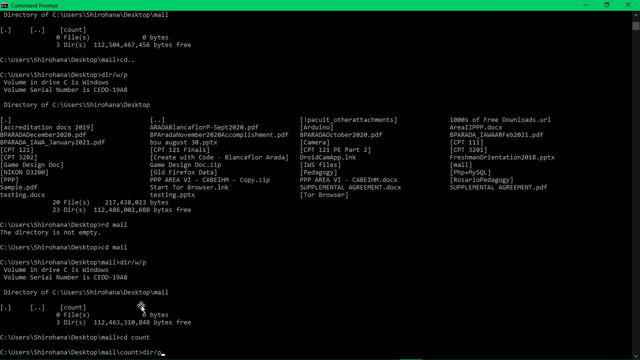 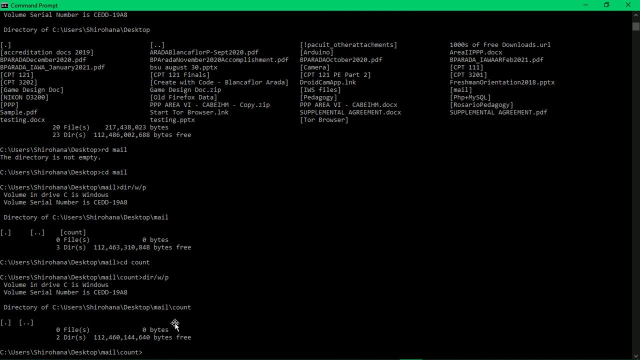 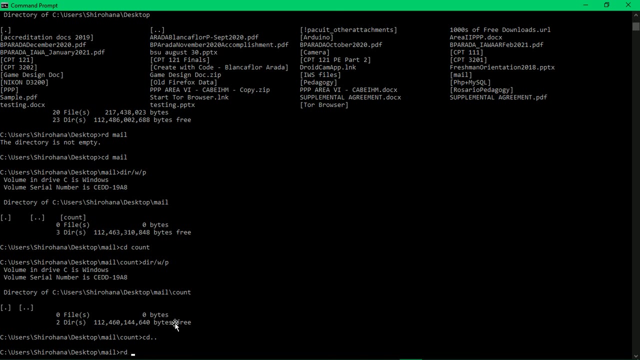 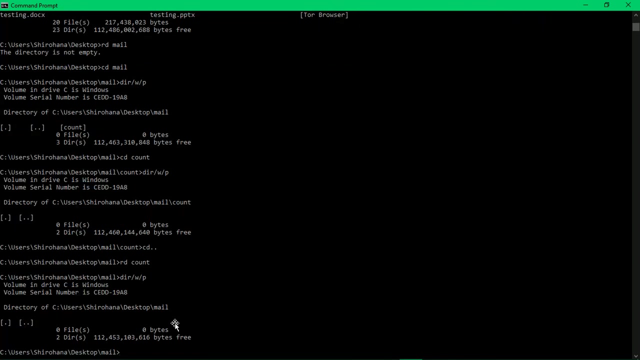 okay, dir slash w slash, dash slash w slash p. it really does not have any content. so, okay, you can't delete this folder count because you're inside it. so you have to go back, you have to be inside mail and then rd count. okay, dir slash w slash p. so count um directory is not. 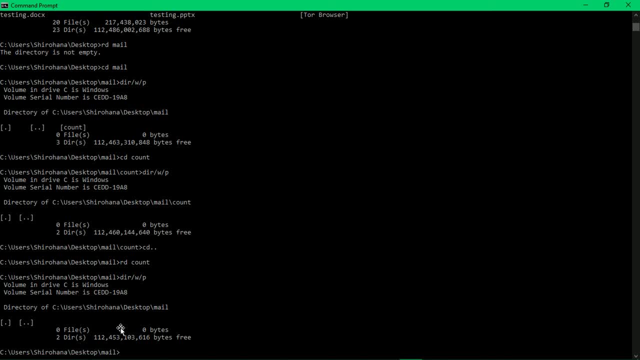 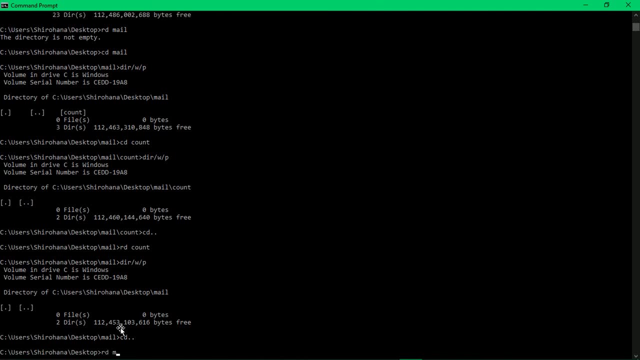 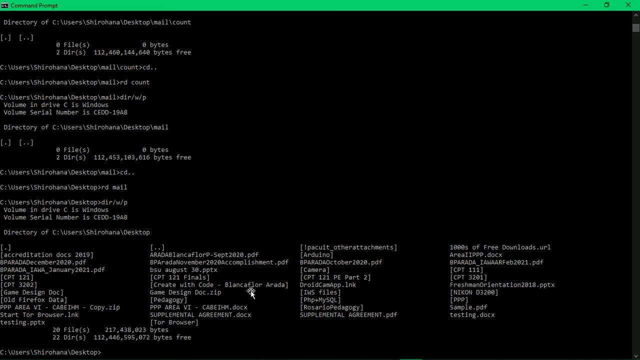 uh, already, it's already deleted. so it's already safe to delete mail directory or folder. so rd mail. okay, so dir slash w, slash p. so is there any mail? okay, does not have any. uh, mail directory inside desktop. okay, so this is how it's done in command prompt, so let's exit. okay, then let's return. 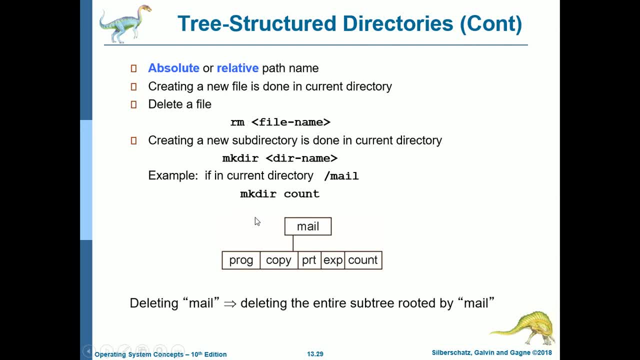 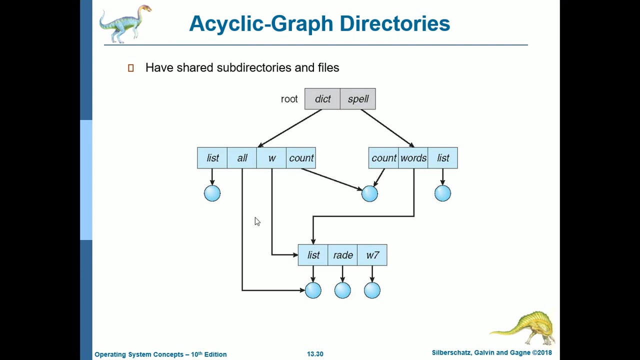 so again, to delete a folder, for file explorer it's easy, just right click and then delete. but if you're inside the command shell you have to make sure that the directory is empty before you can delete it. okay, next is we have acyclic graph directories. so acyclic graph directories have: 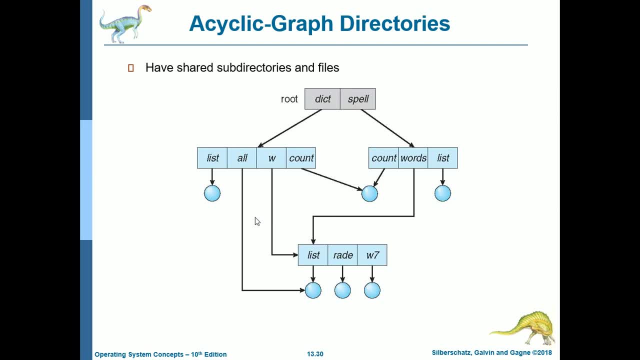 shared directory, subdirectories and files. okay, so this is an example, for we have root for root directory, then dict and spell. so, as you can see, list for dict it has in the folder directory w and then list, and then for spell it is words and then list. so this is what we call acyclic. 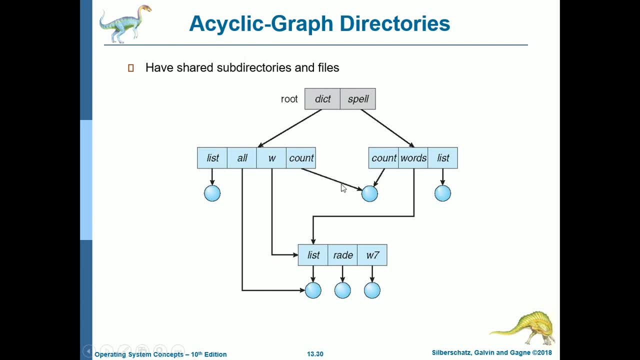 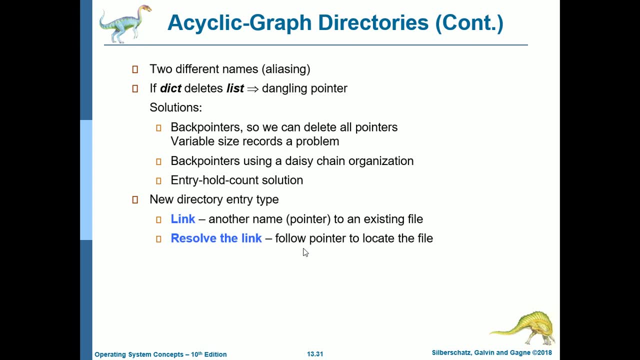 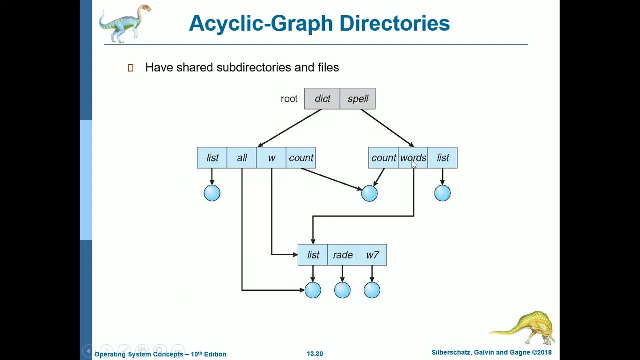 graph directories, because these two directories share the same directory. okay, so the problem here is? so two different names, so aliasing, as you can already see. so for dict, the directory here is w and then for spell it is words, but still they're pointing to the same directory, they're sharing the same. 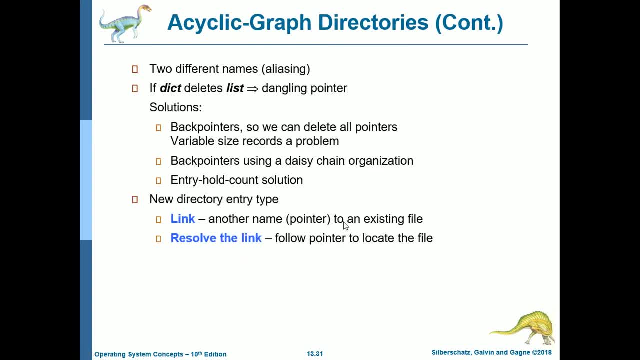 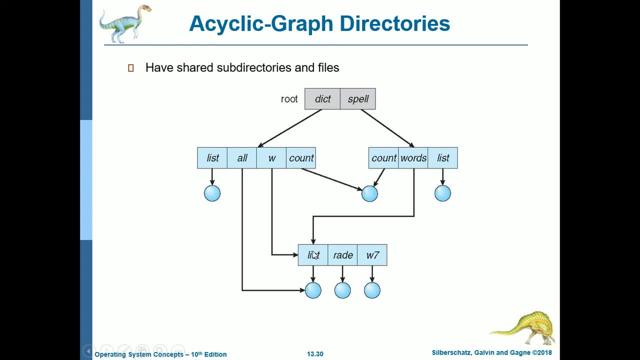 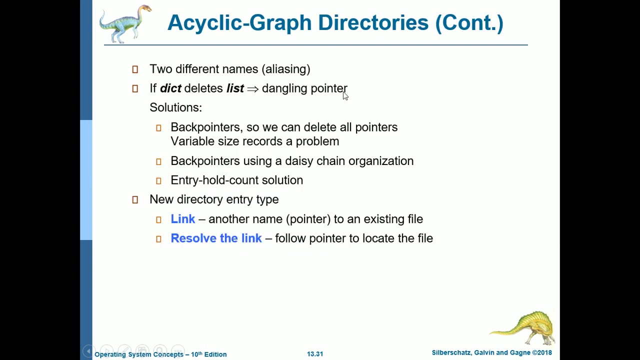 directory. so what if that? if dict deletes list, okay, so the problem here? now let's go back. what if the user dict deletes list? not this list, but this list, because these are shared. so if, if dict deletes this, so where does words be pointing to? so that's why there is a dangling pointer. so the solution is: 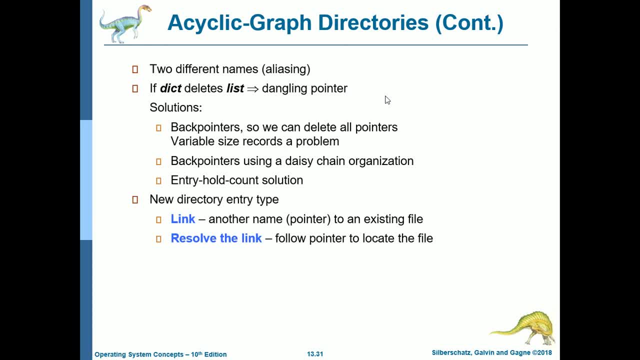 to use back pointers so we can delete all pointers. so variable size records a problem, and then back pointers using a daisy chain organization and then we also have the end entry hold count solution. what is entry hold count solution? account of the number of references. it is typically used in unix for hard links. so next is we have new directory entry type. 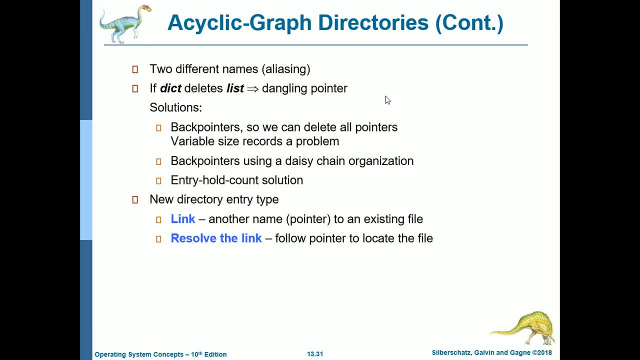 so it's: either we have link or another name or pointer to an existing file, or resolve the link, follow pointer to locate the file. so, as you can already see, to resolve the link, for example your shortcut in your start menu programs. um, it does not look like the icon. 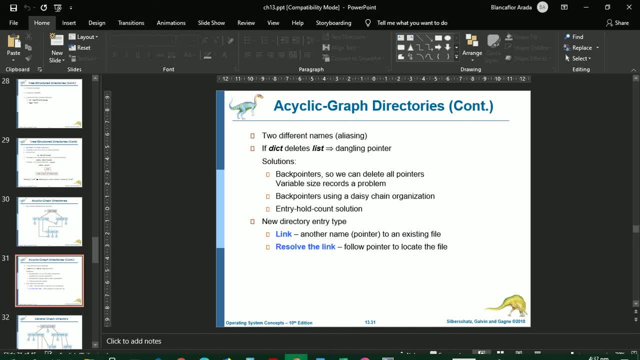 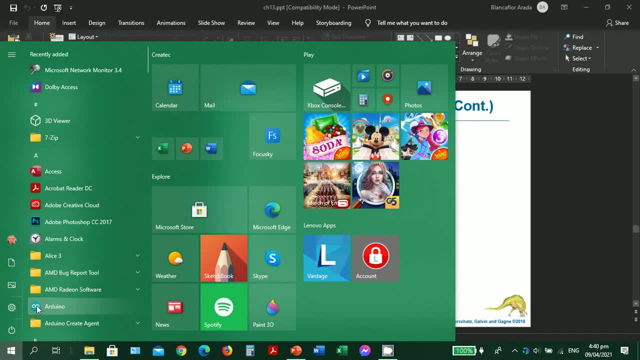 for example: okay, again, let's just illustrate example. uh, you notice that your shortcut here becomes a blank file, meaning um, the target directory or the target application is not correct. actually, you can change the, the direct, uh, the the location, so that it can be corrected. there's also the this: that is the solution for this one. so that is the um. resolve the link. 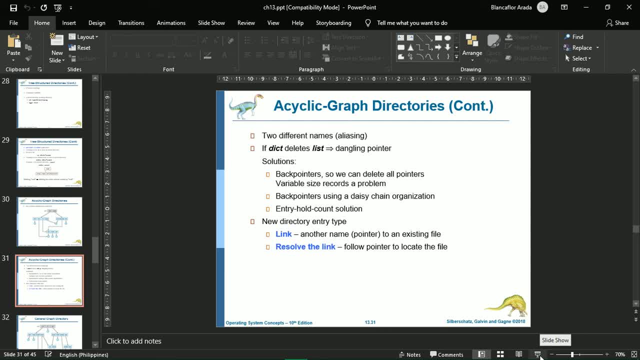 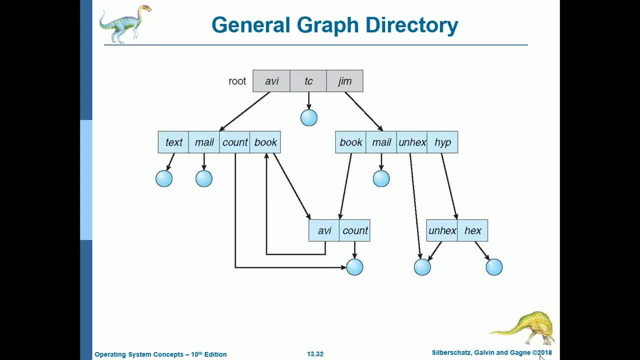 follow pointer to locate the file. you can change the target directory for those shortcut links. okay, next is we have the general graph directory. so again we have the root directory which contains users, avi, tc and jim, and then this is the general graph, because for avi, so, um, the directory of avi book and jim's book directory, it has a pointer for avi and then 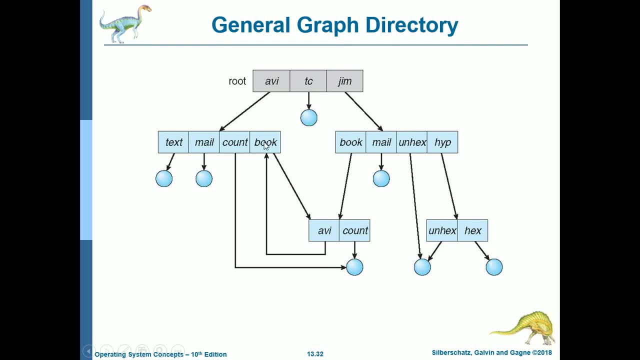 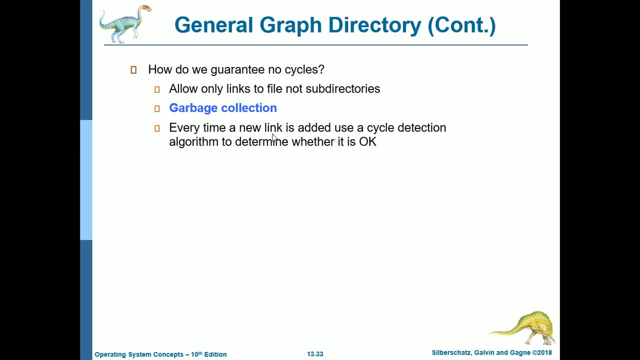 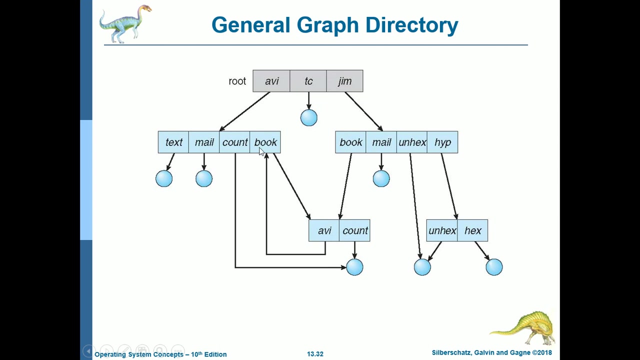 it has also a link inside the directory of book, so that that that is the general graph directory. so, for how do we guarantee no cycles? so allow only links to file, not subdirectories. so, um, for this example, for avi folder, there is also a shortcut here. so that's all. that is okay, because, um, it says here: 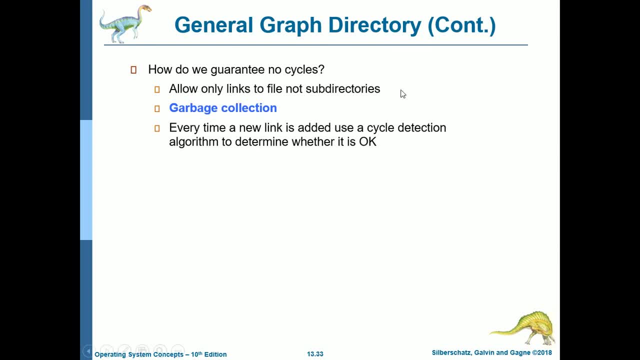 to guarantee no cycles allow only links to file, not subdirectories. and then, of course, we have garbage collection. so to determine whether the last reference has been deleted and the disk space can be reallocated, and then every time a new link is added, use a cycle detection algorithm to determine whether it is okay. 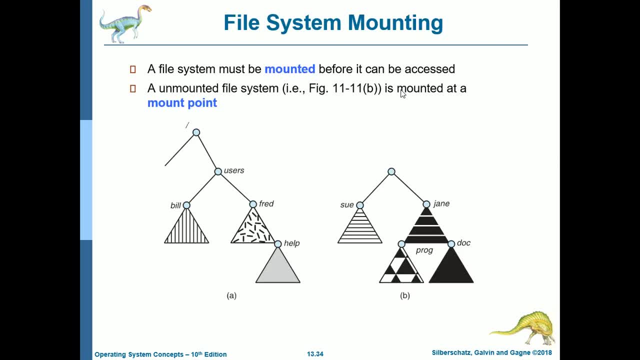 okay. next is we have file system mounting, so a file system must be mounted before it can be accessed. so an unmounted file system with the letter b, so it's mounted at a mount point, okay. so with this one, this letter a is mounted because it is has the root directory, but for b it is not mounted. so that's why that's the difference between. 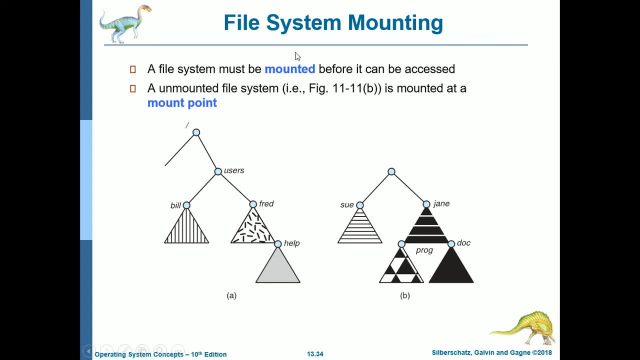 the two. so mounting it's like, um in the case of our computer example, our flash drives. so since our flash drives are drive storage devices, so if you're going to connect it with our computer, and since it's a flash drive, it will be automatically mounted by the computer, since it is registered as 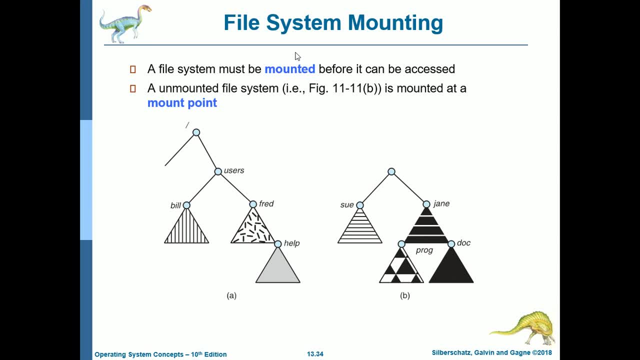 a device drive in the device driver that it has a storage device, so for you to use it it should be mounted. so that's why, if you're going to use your flash drives, you can see that it will appear in the uh alongside with the drives. so it is. 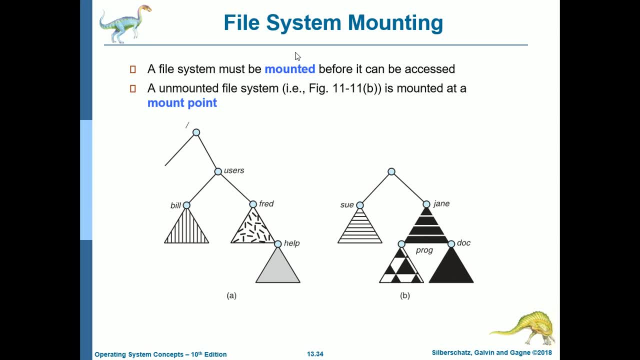 automatically mounted once it is detected, and also for windows. so our hard drives are auto mounted once the computer has started. so you have. you don't have to worry to unmount, uh, to mount the it all by yourself or manually, because windows is the one who's responsible for mounting all the. 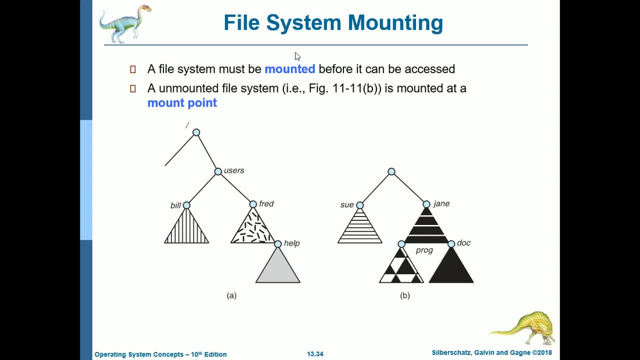 existing drives. so for the case of um of android phones, so if you're, if you're, if your um smartphones is the capability for otg, so if you're going just to insert the otg cable and then connect the flash drive, so as you can see with the storage, if uh, 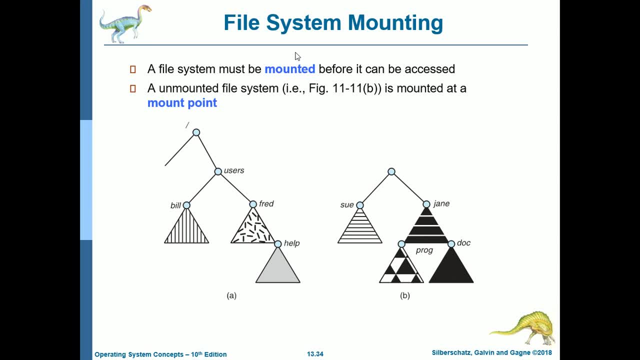 it also automatically mounts if it, if it is detected that the connected in the otg cable is a storage device, and then you can see in the system that, um, you can unmount, unmount the storage device. so what's the use of unmounting? so for again, for flash drives connected in the pc. 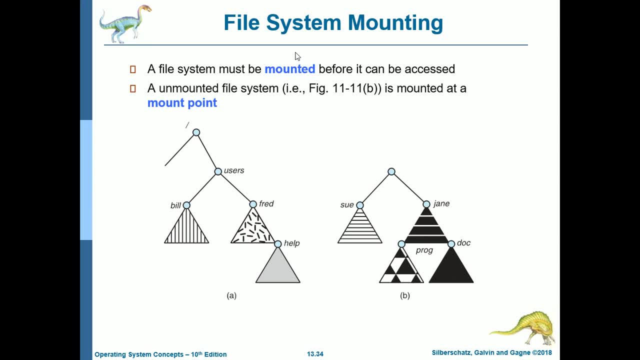 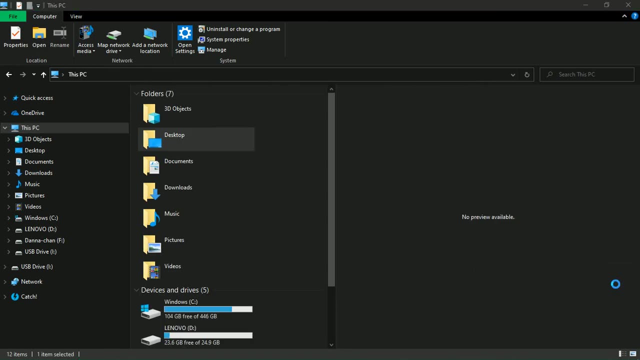 so it's like properly ejecting, so as you can see. uh, let's have an example. okay, i've inserted a flash drive, okay, so let's see if it is detected. oh, there's a problem with my hard drive. well, anyway, so this is my hard drive, so 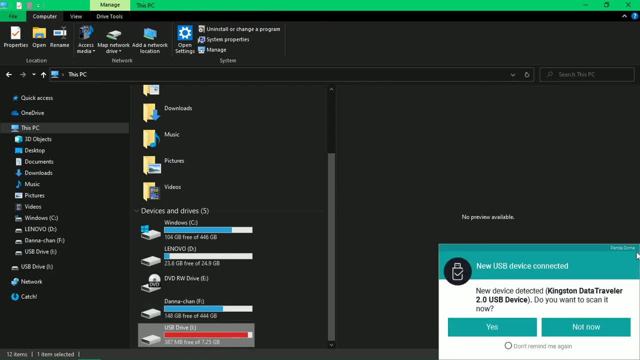 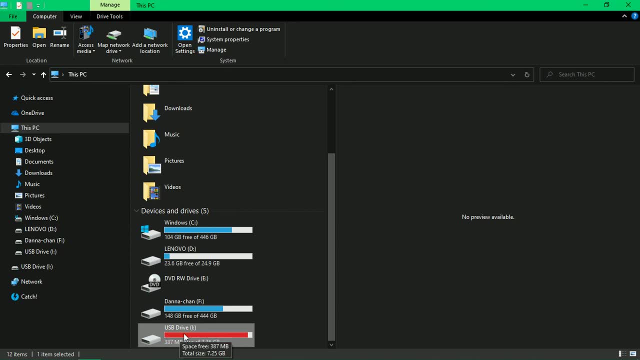 so it is automatically mounted by our uh operating system because it is detected as a storage device, so it is mounted. so to unmount it. so the term here in our computer is what eject for a computer? but for uh smart android smartphones in the system in the storage is we. 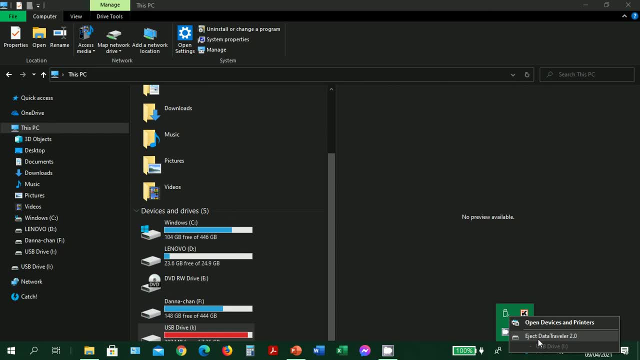 have unmount storage device. they have just this- a different um term for it: unmount and then eject. but the process is just the same. you just have to properly um eject or remove your device. so, um, it's really a really good practice that if you're going to disconnect hard, uh. 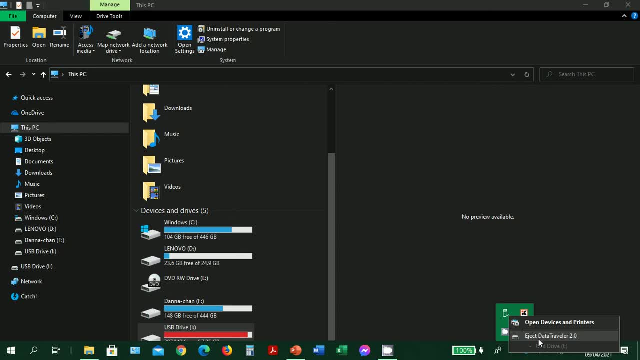 flash drives, you must properly eject it or properly and mount it, because there are cases that if you do not uh unmount it properly or eject it properly, uh, the time again that you're going to insert the device, it becomes unusable. so better safe than sorry, just follow the uh the protocol. 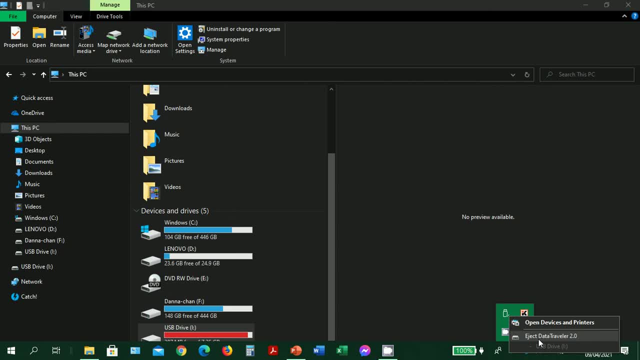 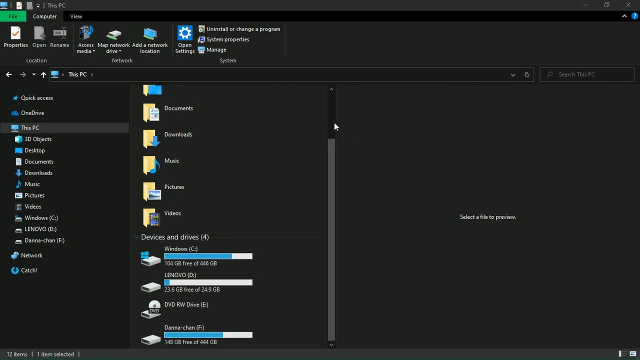 that to eject your removable drives properly. so if you have here eject- or actually it's also in here- you can eject. so this way you can also connect your remote driver to the tablet, and then you can also protect your files and of course your um removable drives too. so it's better to properly eject, or. 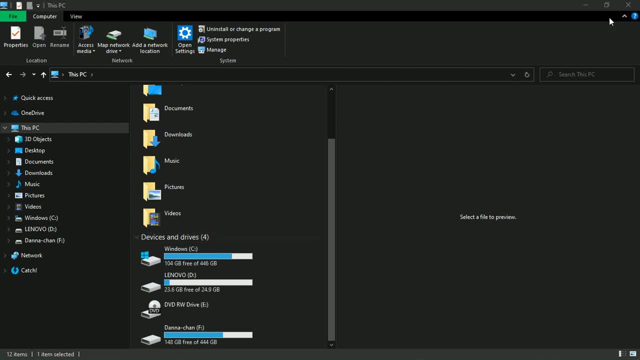 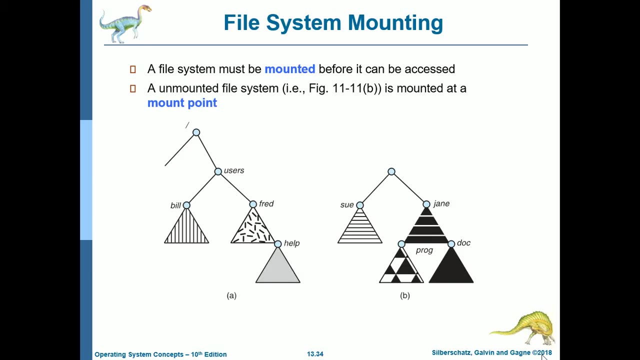 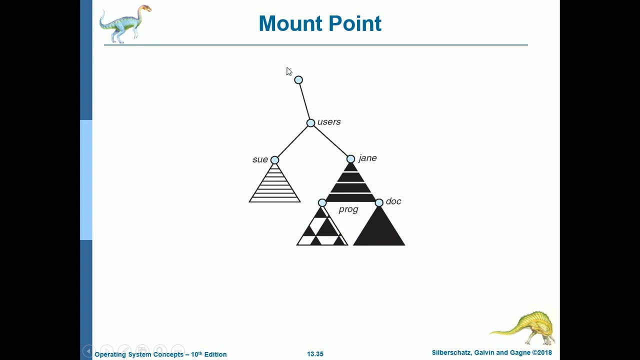 properly unmount, specifically for um, for smartphones. okay, so that is the concept of file system mounting. so the mount point is this one, so the root directory. so it means that it is mounted on your system and then, for windows, you can actually know if your drive is mounted, because you can see the drives in the list in this pc, for example. 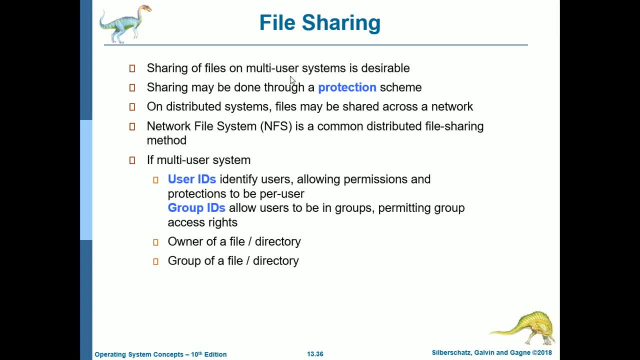 okay. next is we have file sharing, so sharing of files on multi-user systems is desirable. so sharing may be done through a protection scheme on distributed systems. files may be shared across a network, so sharing of files on multi-user systems is desirable. so a network file system, or nfs, is a common distributed file sharing method. 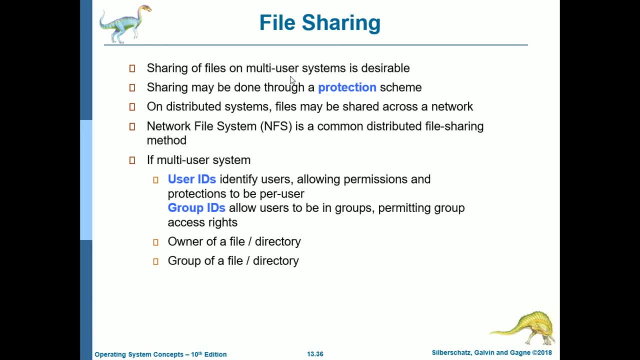 if multi-user system, they can use user ids to identify users, allowing permissions and protections to be per user, and then group ids allow users to be in groups, permitting group access rights, and then you can be an owner of a file or directory or group of a file or directory. 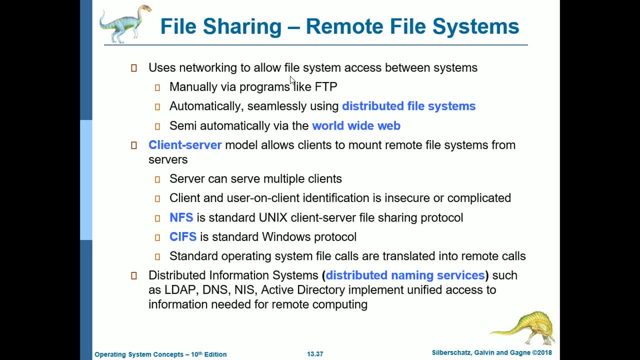 this can be shared. so for file sharing in remote, remote file systems. so uses networking to allow file systems access between systems manually via programs like ftp, automatically, seamlessly using distributed file systems and semi-automatically via the world wide web. and then the client server model allows clients to mount remote file systems from. 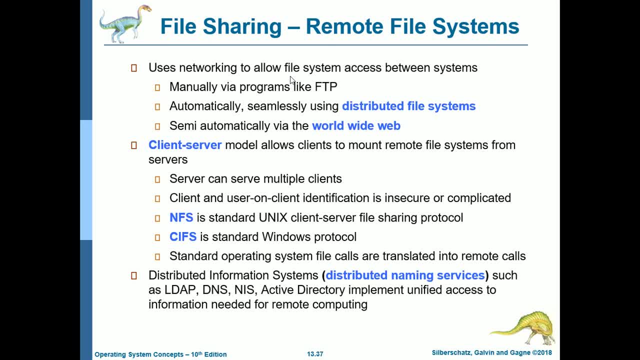 servers. server can serve multiple clients, client and user on client server, and client server can also be used in remote, remote file systems. so again, nfs is a standard unix client server file sharing protocol and cifs, which is common internet file system. so the windows network file system now used on many systems, the cifs. it is the standard windows. 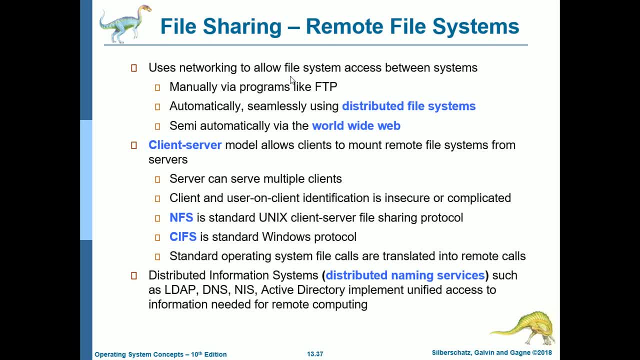 protocol, so standard operating system. file calls are translated into remote calls, so distributed information systems or distributed naming services, such as ldap. so ldap is lightweight directory access protocol or dns. so dns is domain name service or domain name system. and then nis is network information service and active directory implement unified access to information needed for. 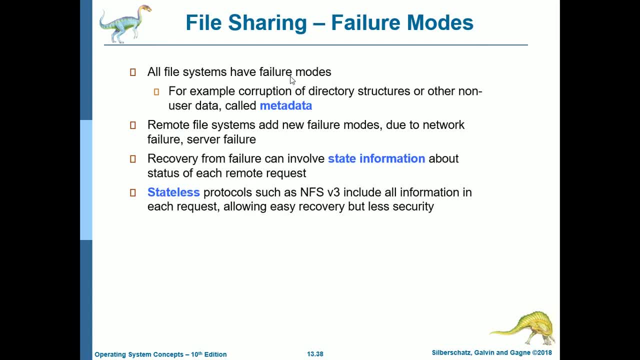 remote computing. so what are the failure modes for file sharing? so all file systems have failure modes. so, for example, corruption of directory structures and other non-user data called the metadata. so remote file systems add new failure modes due to network failure or server failure. so recovery from failure can. 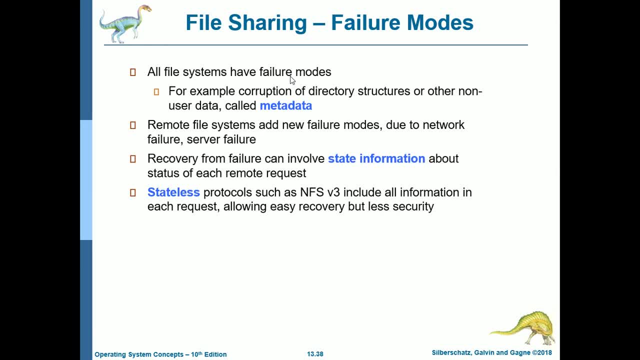 involve state information about status of each remote request, so state information. so in remote file systems, the set of information pertaining to connections and ongoing file operations, such as such as which files are open. so for stateless protocols such as nfs, version 3, include all information in its request, allowing easy recovery but less security for stateless protocols. so 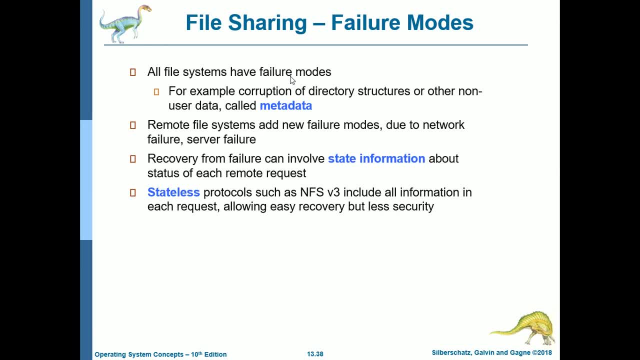 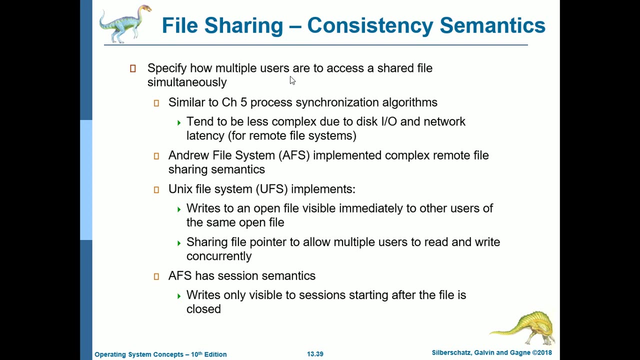 in a remote file system, a protocol in which state need not be maintained for proper operation. so that's cool. that is why it is called stateless protocol. okay. next is for consistency: semantics for file sharing. so specify how multiple users are to access a shared file simultaneously. so similar to chapter 5's process synchronization algorithm. 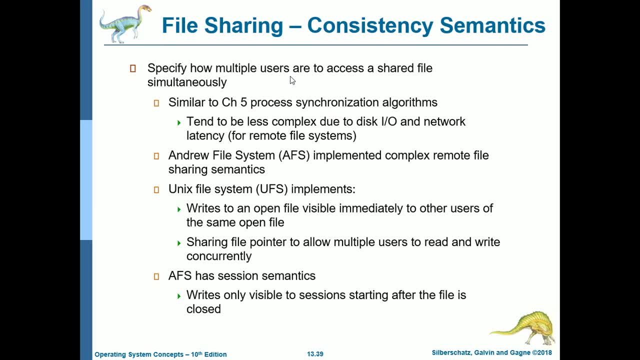 so it tends to be less complex due to disk, io and network latency for remote file system. and then there is a file system which is called android file system, or afs, implemented complex remote file sharing semantics. and then unix file system, or ufs, implements writes to an open file visible immediately to other users of the same open file sharing file. 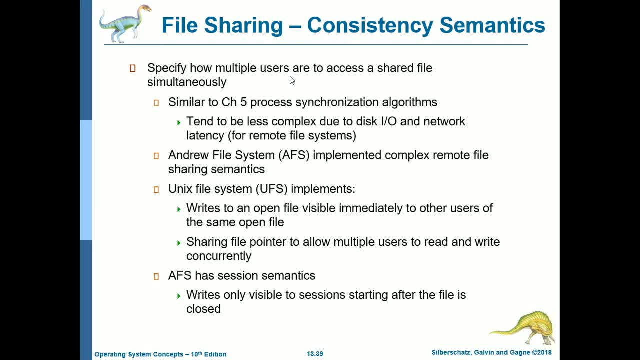 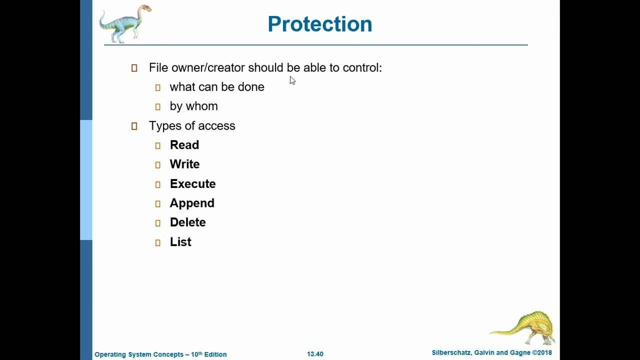 pointer to allow multiple users to read and write concurrently. so for android file system it has session semantics writes only visible to sessions starting after the file is closed. so next is we have protection. so the file owner or creator should be able to control what can be done and by whom. 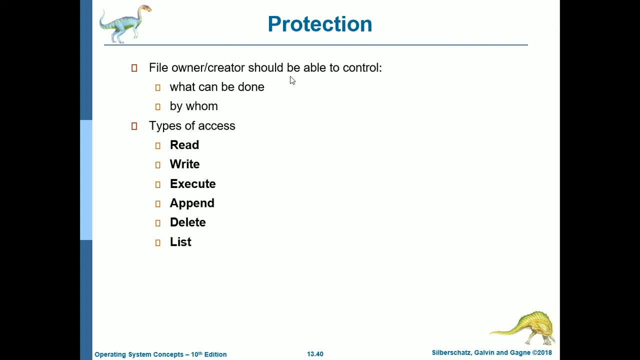 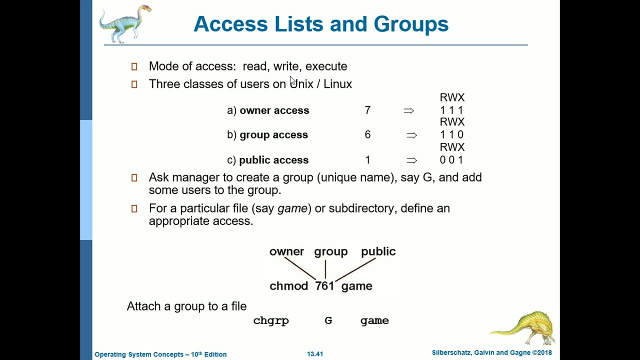 so the types of access are read, write, execute, append. so append is write new information at the end of the file and then delete and list. so next is we have access, lists and groups. so the typical modes of access is read, write and execute. so for a unique file system it is important to have access, lists and groups. 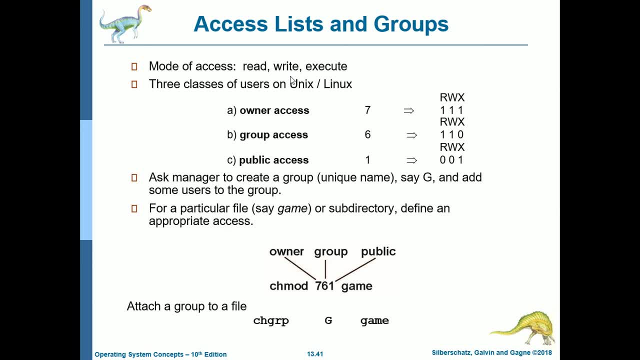 and linux, though the three classes of users are. so owner access, so the code is seven. so this is for read, write, and then x is for execute, so y it is seven. so, um, so owner can read, it can also write, because it's one it, and then it can also execute. y it is seven because, as you can remember, with 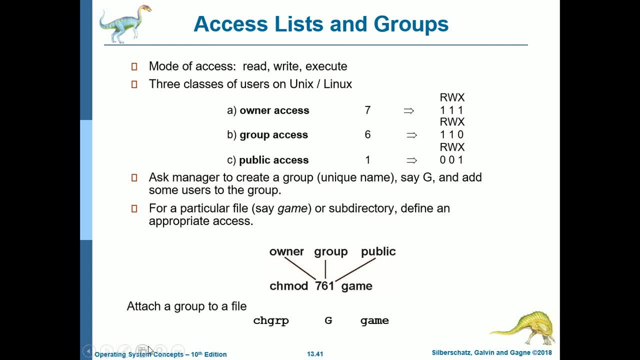 um, binary, okay, let's have. this is four, okay, then two and then one. let's add those that are one, four plus two plus one. four plus two, six plus one is seven. so their code for owner access is seven, based on the binary. okay, so that's. 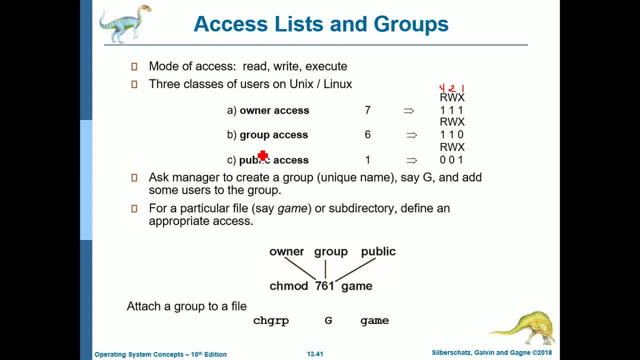 why it's code seven? okay, next is group access is code six. why it is code six? uh, group access can read and write, but it cannot execute. so six is code seven and then y is code seven, and then y is code seven, because four plus two is equal to six, and then public access is only it's code one. why? 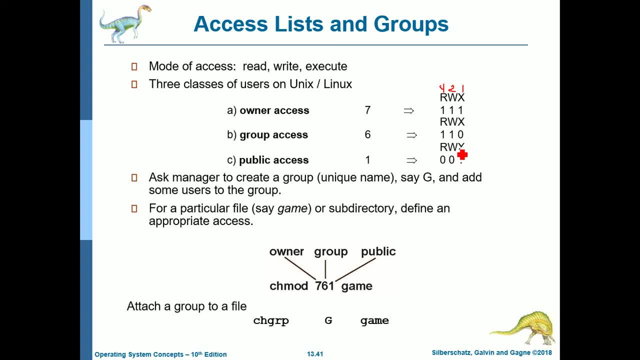 public access. it cannot read, it cannot write, but it can execute. so that's why its code is one. so ask manager to create a group or unique name, say g, and add some users to the group for a particular file, so say game, or subdirectory, define an appropriate access. so 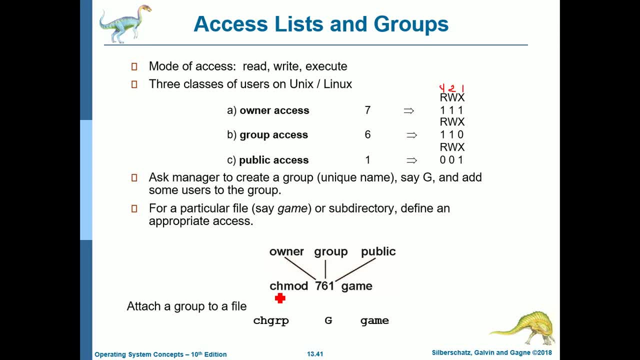 to to define. so ch mode 7, 6, 1. so meaning uh can be a owner group or public, and then the subdirectory is game. so attach a group to a file, ch, group g and then game. so this again the, the commands. here is not windows, but more of unix or linux. so this is the windows 7 access control. 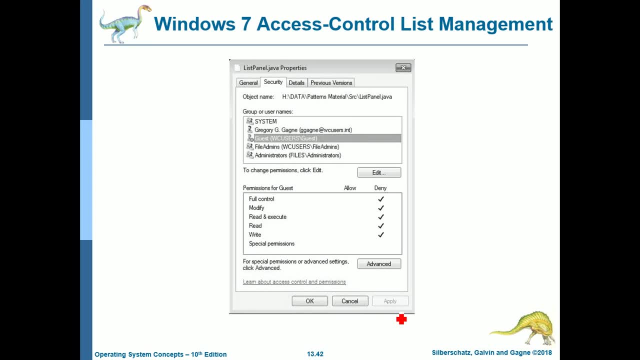 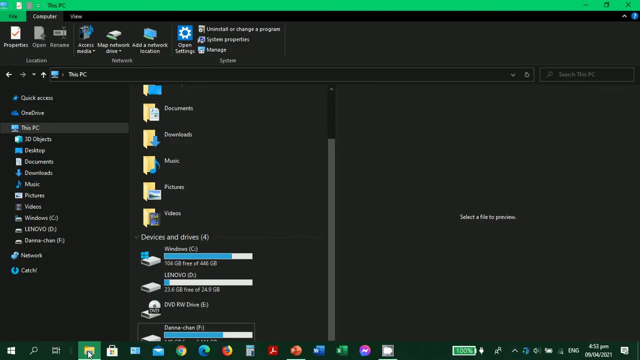 list management. but again you can see the, the command is windows and then you can see the command is theid to g and then you can see the command is going to the h你就 dis, we train the feature. so Again you can see that in our okay. so just discard my okay. let's again return. 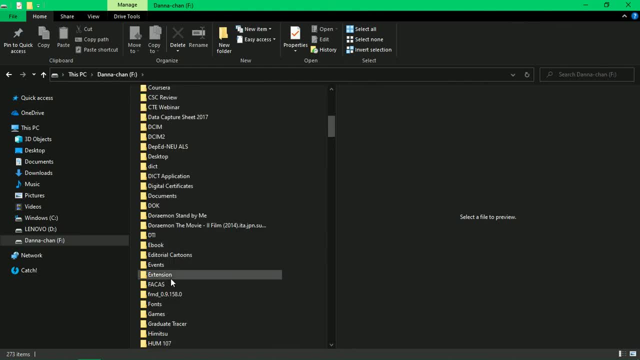 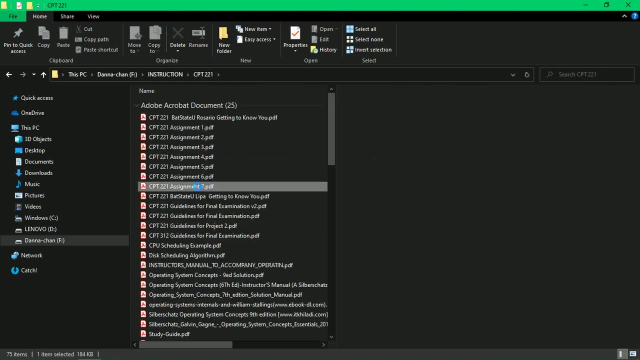 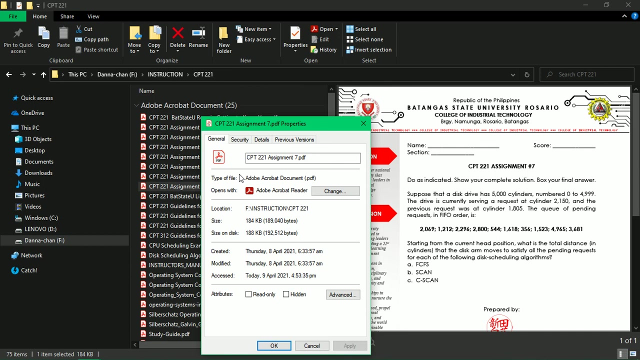 So again, sorry for the delay for the context menu again. Okay, let's return to our. okay, Let's wait again for the context menu to appear. Okay, counting, Okay, thank you again. Okay, properties, then security. 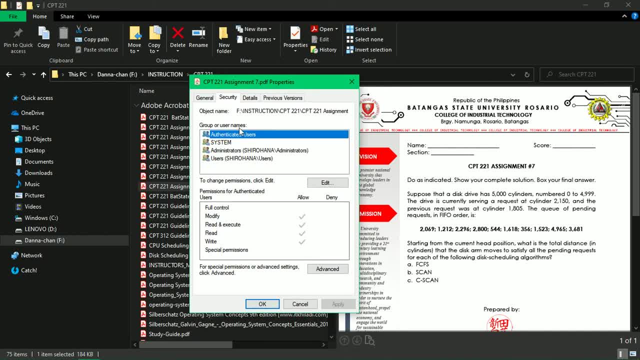 Actually it's in security, So the group or usernames that can access this file, we have authenticated users. So for authenticated users, so this ID. so the ones in the presentation are the common access modes, But here in Windows we have full control, modify. 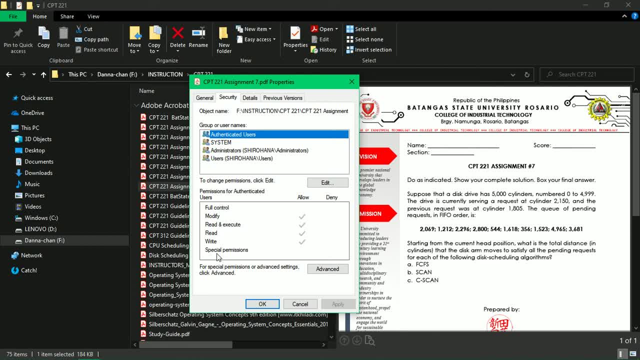 Read and execute, read, write and special permissions. So if you're an authenticated user, you can modify the file, You can read and execute, read and write. So because that's we have allow, Then there's no marks for deny. 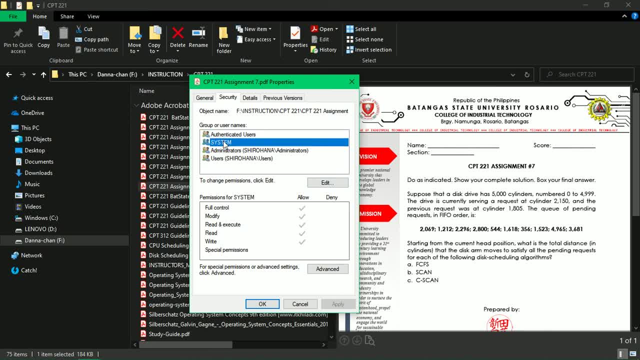 Then for system. so if the user is a system, it has full control. So that's the difference with authenticated user from system, because it does not have any full control And then the only thing is we have- there's no check for special permissions. 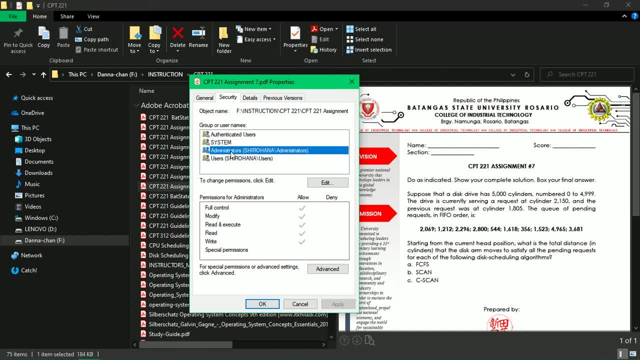 So for administrator, so just the same with system, If you knew the username and password of this computer system. And then for users, so if you're a public user, so you have only read and execute and read Or any users identified inside this folder. 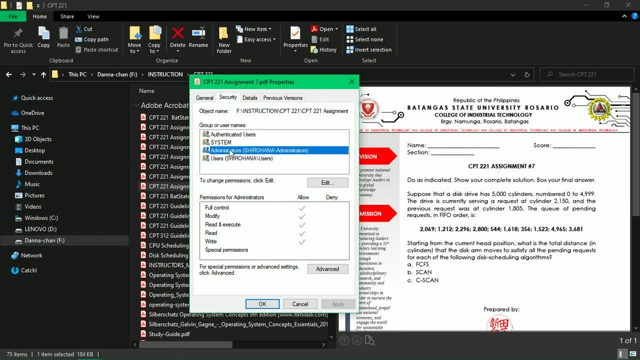 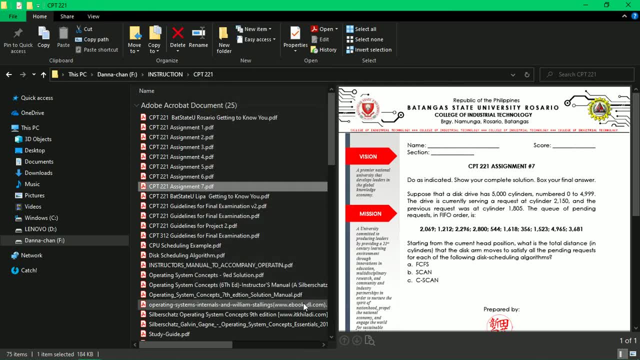 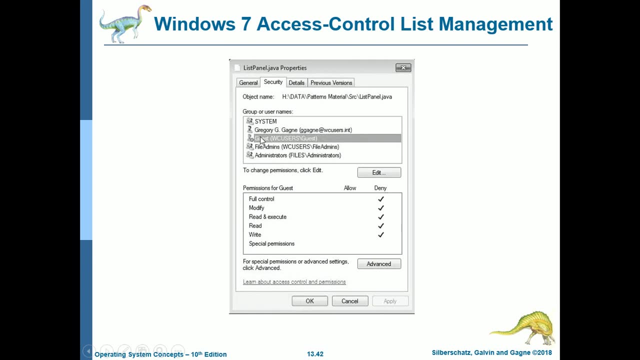 So you can see different users. they have different access modes. Okay, Okay for this example. so if you're a guest, it is all deny, You just can view the file. Okay, this is an example of Unix directory listing. 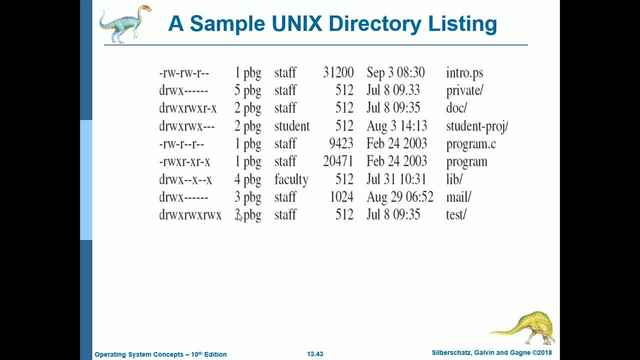 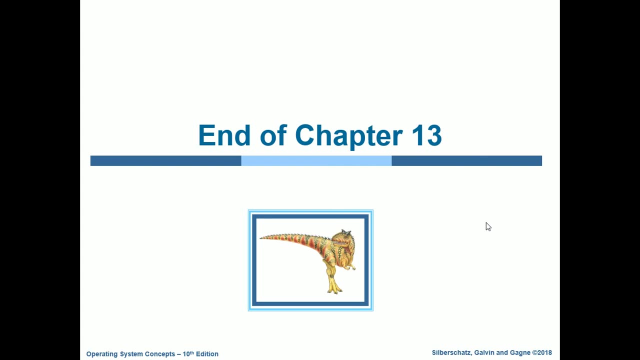 So of course it's A little bit different with Windows, Because of course we're familiar with the Windows system. So it's just show that this is the directory listing for Unix. So okay, So this is the end for our chapter, for our lesson.